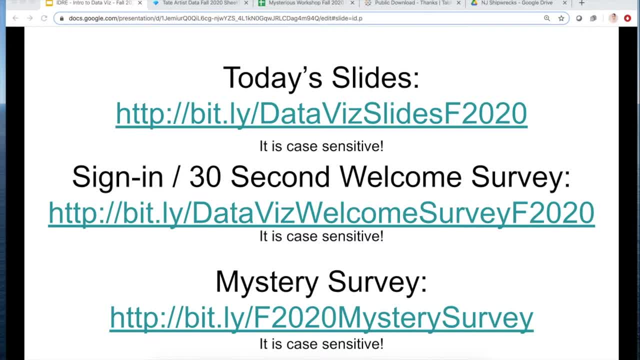 time. so data and visualizing data is very important to what I do and what I love to teach. Letting a few others in to join us and if you're just joining us now, please take a look at these surveys, fill those out really fast and I'm sending. 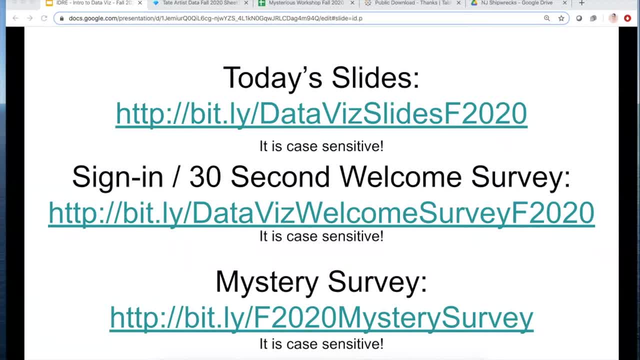 you a link to the slides for today in the chat So as we sort of get settled in, keep a lookout. I just want to say for a coding for creatives workshop for me in November and for more XR or extended reality workshops that I'll be teaching in the winter and spring and if you have 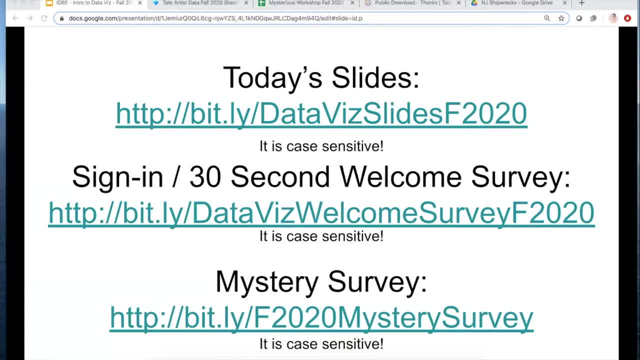 any questions or interest in learning a particular skill in extended reality. let me know, immersive technologies are sort of my main thing as we were trying to build out our resources in that area, So I'd love to hear from any of you who are interested. 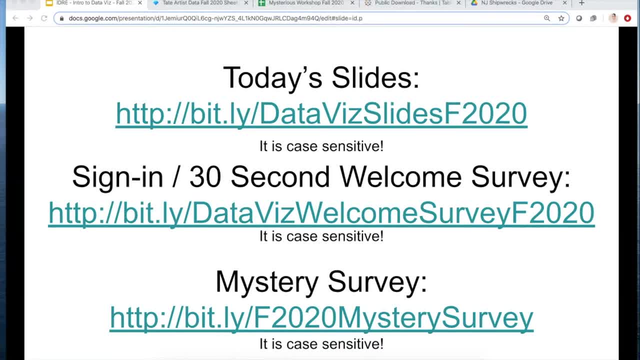 And so please, someone is asking in the chat to add the links in the chat for the surveys. I'd have to pop out to do that, But actually if you go into the slide deck you can get the links right in the slide deck. 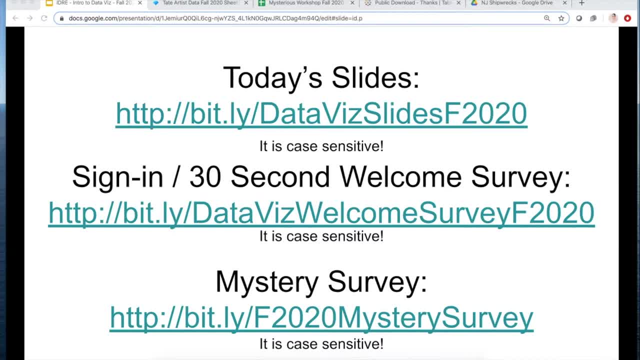 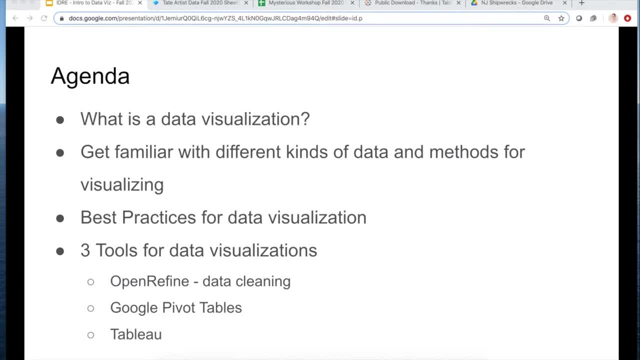 So you can help yourself there. All right, So I'm going to go ahead and move forward and go over our agenda for today. So today, what we'll be covering is: what is data visualization, first and foremost. We'll also get familiar with different kinds of data and methods for visualizing. 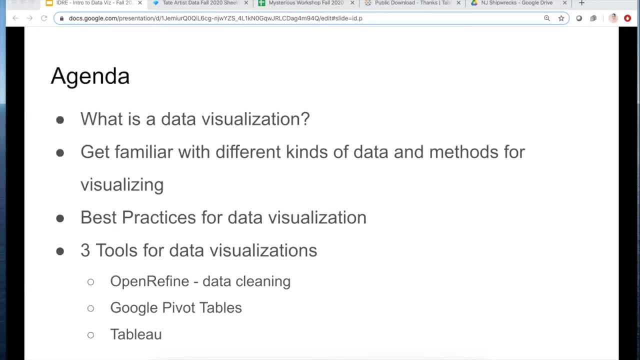 We'll cover best practices for data visualization And then we'll look at three tools for data visualization. So first is OpenRefine, which used to be Google Refine and is a free, open source tool that helps with data cleaning. So, before you visualize your data, 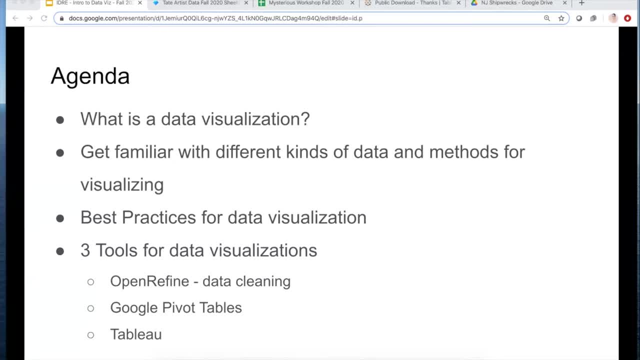 You want to make sure that you have clean, standardized data, So we'll look into that. Then we'll also work with Google Pivot Tables as a bit of an appetizer, And then we'll get into Tableau, which will be our main course for today. 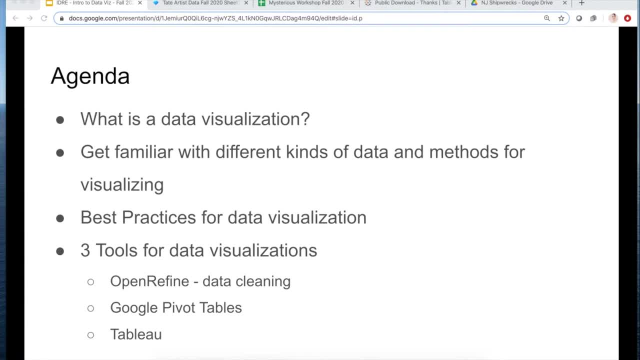 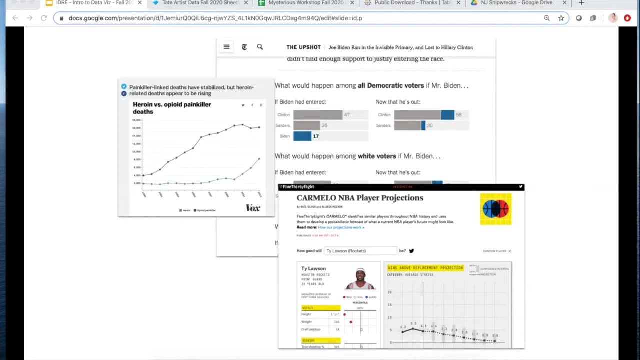 So if you have any questions again for those just joining, you can follow along with this presentation at the link in the chat. So data visualizations are everywhere today. We see it in news, medicine, politics, sports. They play a vital role in how we communicate and understand what is happening in the world. 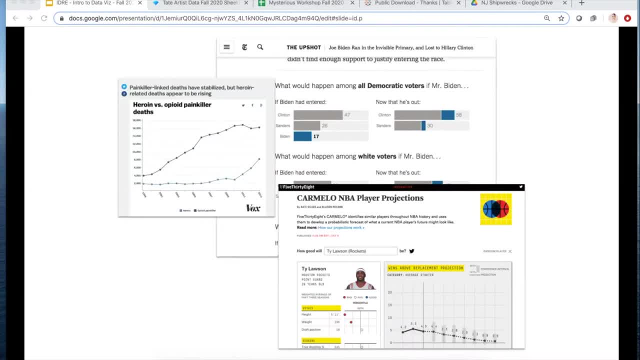 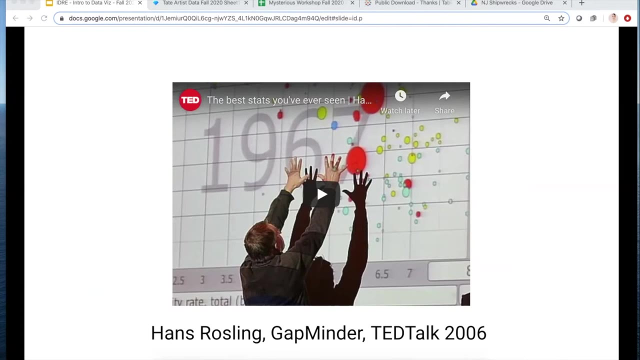 around us. More specifically, for scholarship, they can be a vital method contributing both to the process and product of research. So Hans Gossling's gap minder Data visualization project is a great example which you can see here. I won't play the video now because I know videos over Zoom can be a little stop and 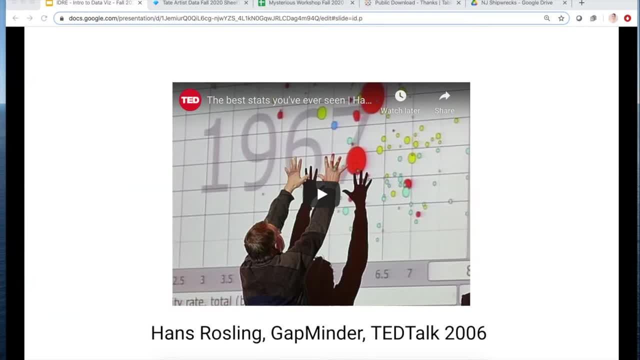 start at times, But if you want to take a look at that at your own leisure, I highly recommend it. But it's a great example of how we can create strong academic arguments with data visualizations. He plotted health data from all over the world. 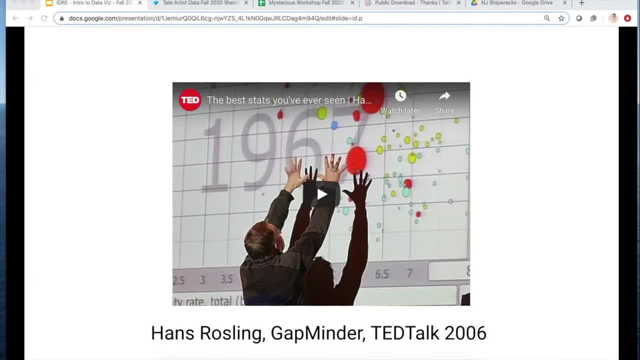 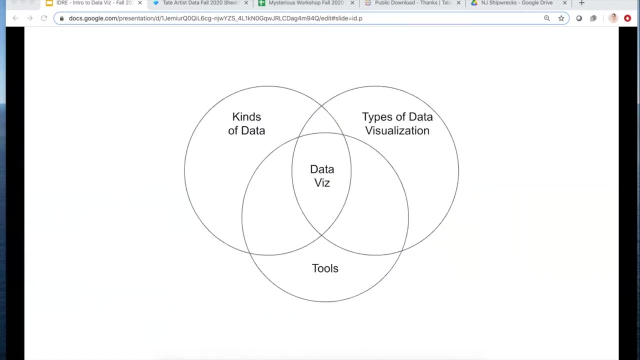 And animated it so we could see the change. over time, This bird's eye view really shifted the narrative in regards to developing quote unquote countries and what their health situations were like. So to make a data visualization, you need three things right. 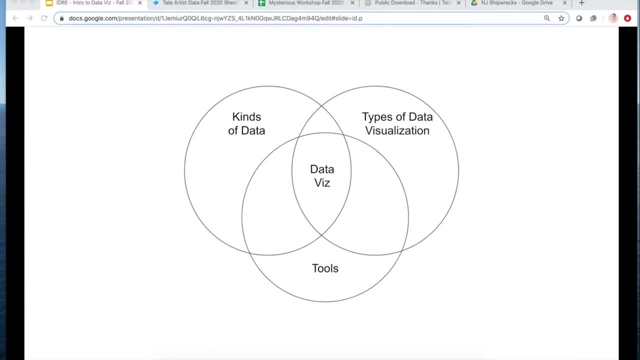 Data format for data viz and a tool that can produce data. So it's that format, So it's the intersection of these three things, And to pick the best visualization type for your data, you need to understand what kind of data you have. 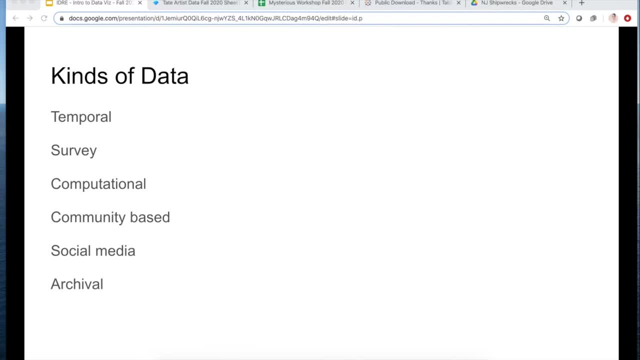 Here are a few examples of the kind of data people want to visualize typically. So there's temporal data, So this is time-based data, where the goal is to understand changes over time. Things like survey data can help us get an overview of what's happening in the world. 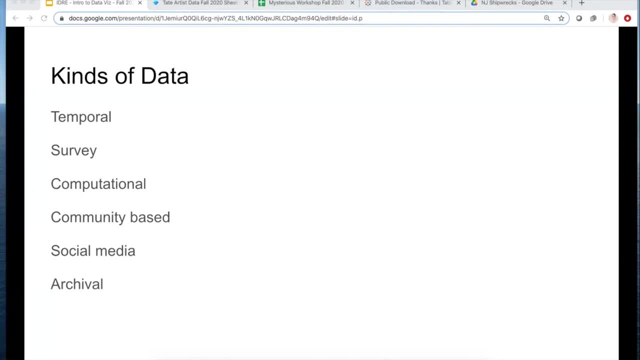 And then there's data analysis. And then there's data analysis. So there's overview based on clear boundaries set by the PIs of the study. There's computational data. right, Usually these are big data sets that involve mathematical equations to produce. 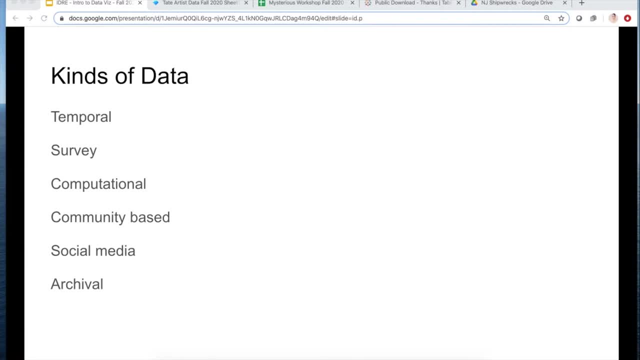 There's community-based, So census or demographics. We see that a lot- Social media, Calming platforms like Twitter and using indexes or hashtags to identify particular information Or social media Archival data. This is what I'm most familiar with. 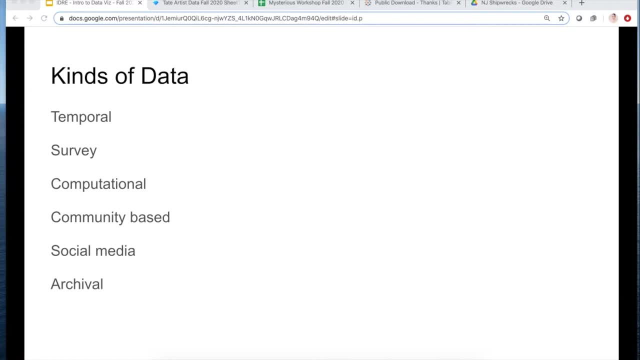 Usually collections data has a lot of metadata attached to it, So old manuscripts, photographs, things like that found in special collections. But maybe we can just take a second as a way of getting to know one another and what everybody's working on. If you wouldn't mind sharing in the chat what kinds of data you're working with or what. 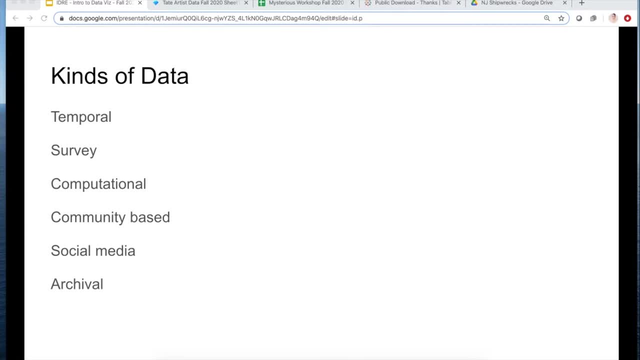 other kinds of data outside of this that you're interested in. So I'll give everyone a second to just go ahead and put that in the chat, And then we'll get started, Thank you, Thank you. Thanks for the chat. So Catherine shared that she's working with lots of social media data. 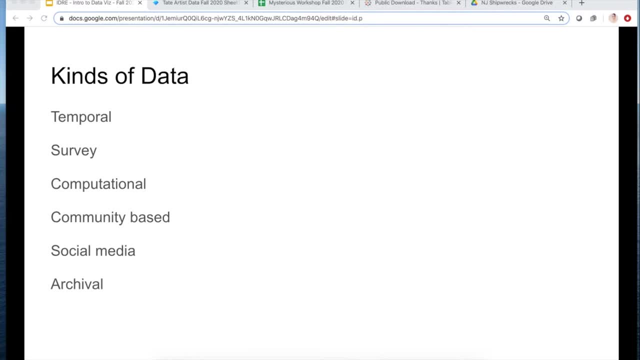 Lots of people work with social media data, Computational archival, Great Medical records, Absolutely, Biodiversity data surveys- Sure, All of these are wonderful, And these are exactly the type of things that we're talking about here, right? 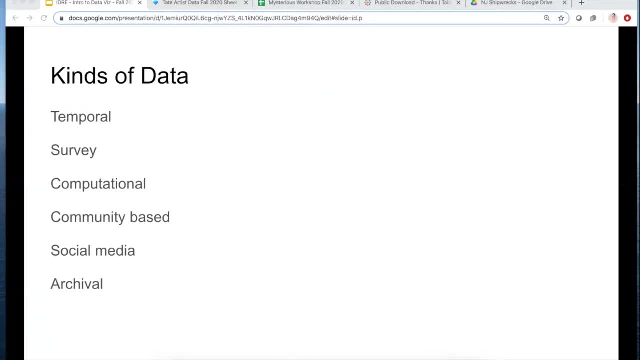 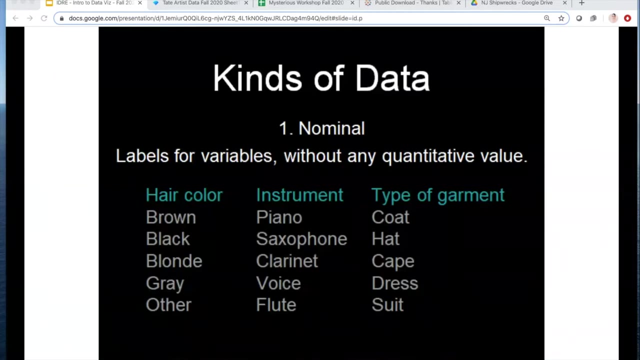 And it's really important to be able to showcase these things in a way that we can communicate a lot about this data in a single image. So that's where the power of data visualization comes in. So it's important for us to understand a little bit about. 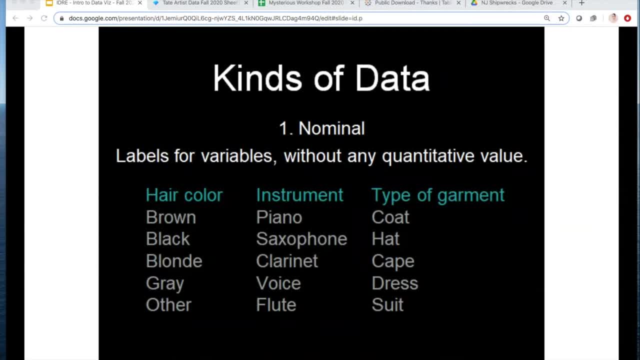 the kind of data we have in order to know how best to represent it visually. I'm not a statistician, but these basics are very helpful to know And I hope any people in statistics in the room will feel free to correct me if I'm getting anything wrong. 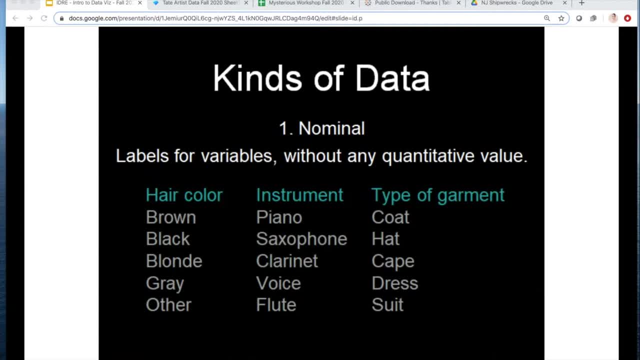 or confused. help me clarify things, if need be. But in statistics, nominal data, also known as nominal scale, is a type of data that is used to label variables without providing any quantitative value. It is the simplest form of a scale measure. 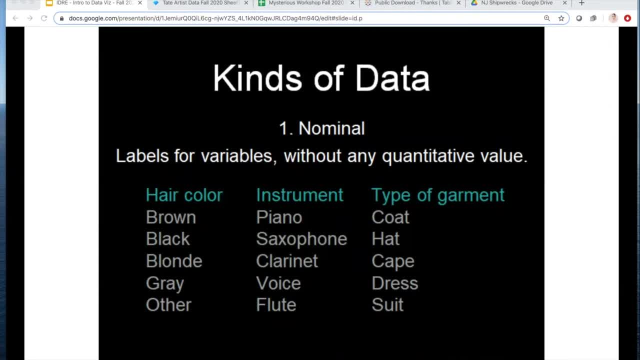 Unlike ordinal data, which we'll talk about in a minute, nominal data cannot be ordered and cannot be measured. So here are some examples: things like hair color or different kinds of instruments- right, Those don't have a value per se, but they are things. 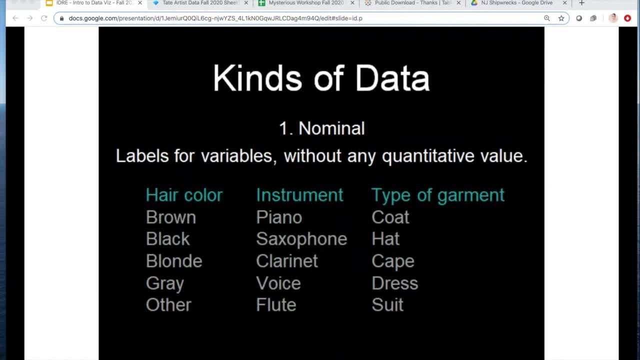 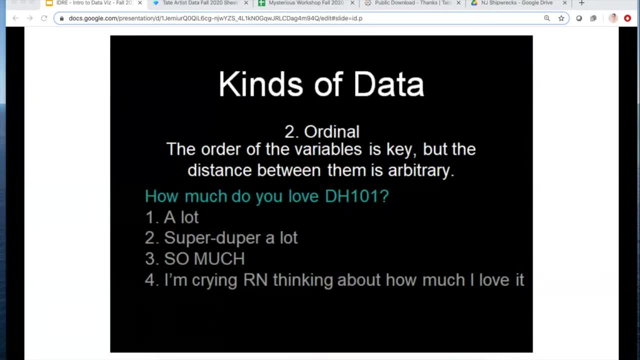 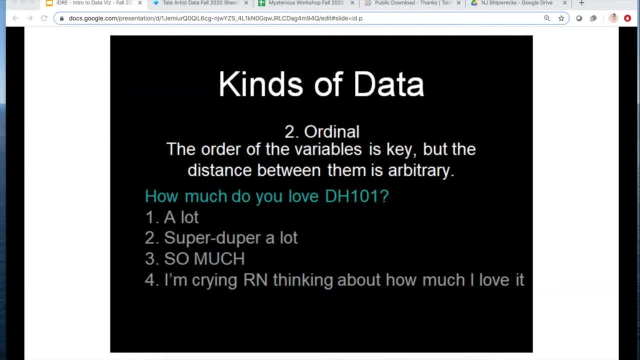 the equal increments of the underlining attribute. So I teach DH 101 on occasion- digital humanities, introduction to digital humanities, And so this example pertains to that. So if we're giving an example of ordinal data, it'll be these types of categories right A lot. 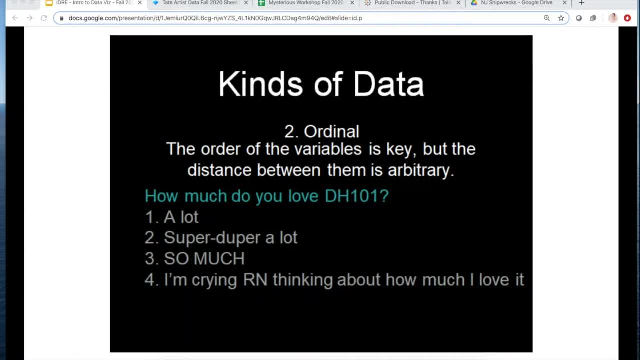 super duper a lot so much. I'm crying right now, thinking about how much I love digital humanities. Well, all of these things don't have a specific measurement in between them. We just understand intuitively the difference between them, And this will become clearer when we talk about the next. 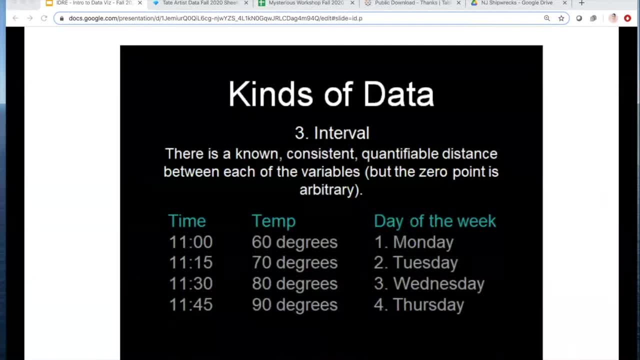 thing which is interval. So interval data, also called integer, is defined as a data type which is measured along a scale in which each point is placed at equal distance from one another. Interval data doesn't have a defined absolute zero point, which is present in ratio data. 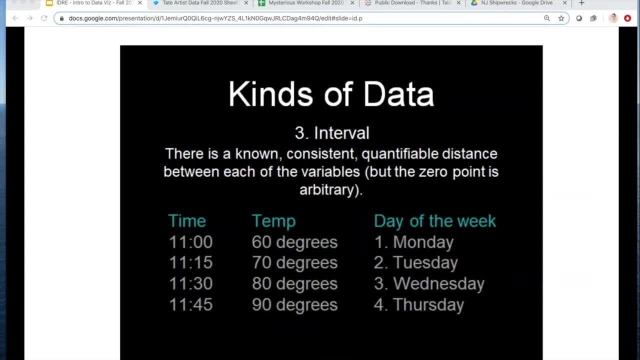 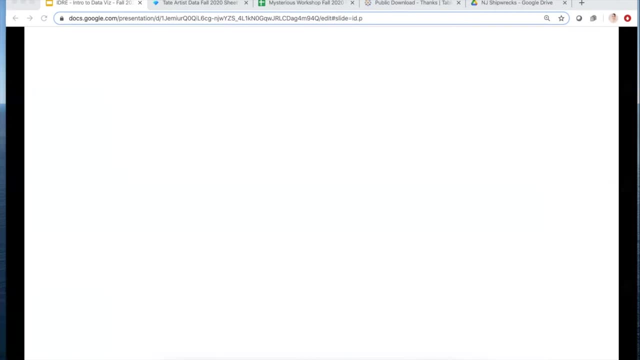 which we'll talk about in a second. The lack of absolute zero makes comparisons of direct magnitudes and possibles. For example, object A is twice as large as object B- is not really possible in interval data And with ratio, which is our final kind of data that we're going to talk about today. 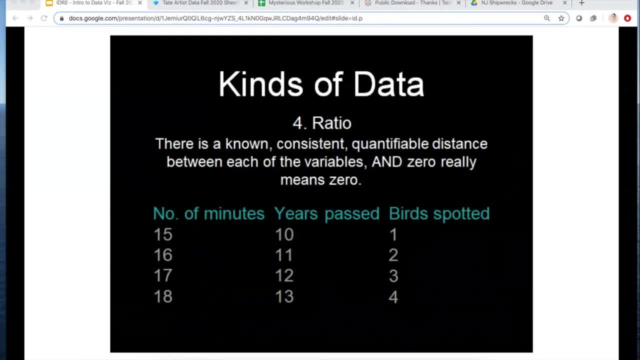 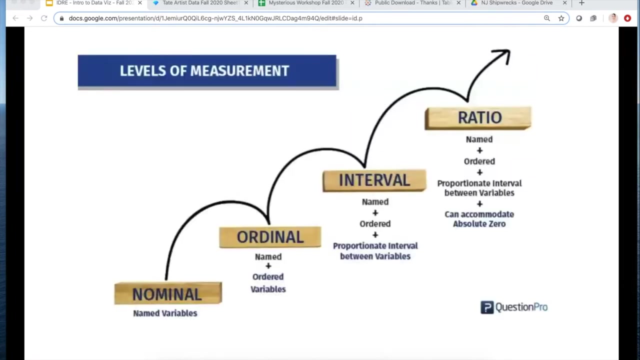 there is a known, consistent quantifiable distance between each of the variables, and zero really means zero. So, for example, you can't have a partial bird spotted. You spot one bird or two birds or three birds right And in any relation to each other. we can view these kinds of data like stepping stones. 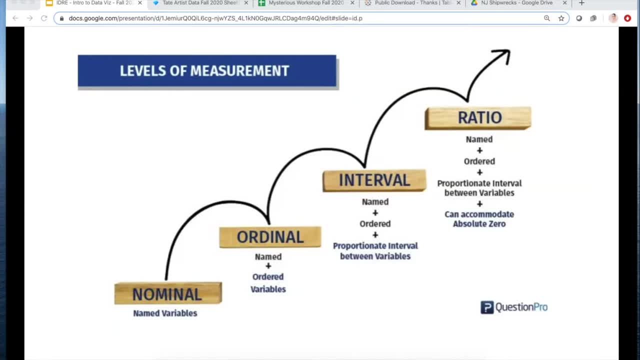 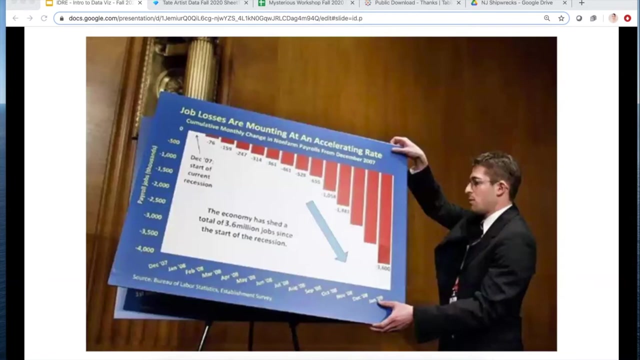 getting more specific and ordered as we go along, And I think this chart makes that really clear. right, We've moved from nominal to ordinal all the way to ratio, each time getting a little more ordered and a little more specific. So what does it mean to take these various types of data and visualize it? What actually 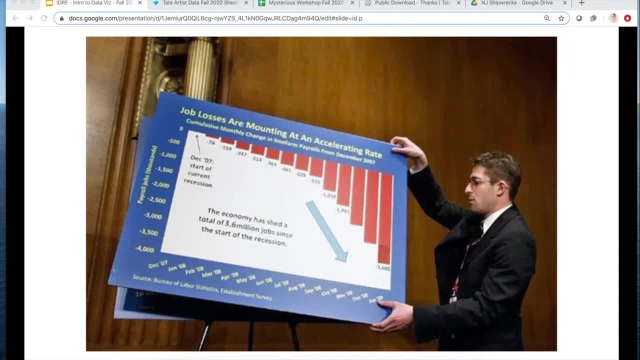 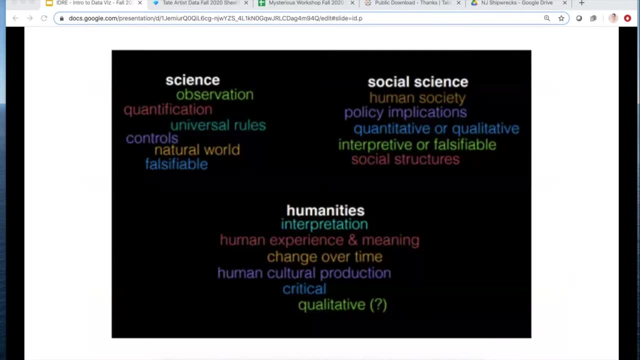 is information visualization? Well, my answer. what I like to say is that it's a mapping between discrete data and a visual representation. More broadly, in terms of scholarship, data visualization is a method like many others, So methods and methodologies vary within disciplines. 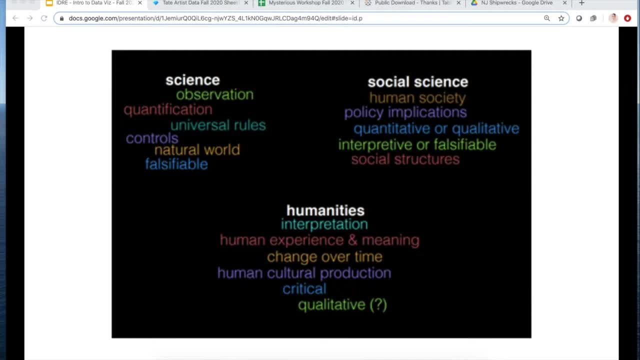 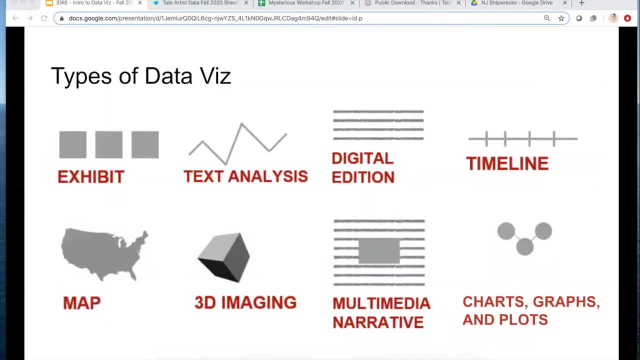 due to overall research objectives, And you can see from these examples here, if you look at science compared to social science and versus humanities, some of these things overlap And as a result so will the process and product of our visualizations. So, for example, the type of 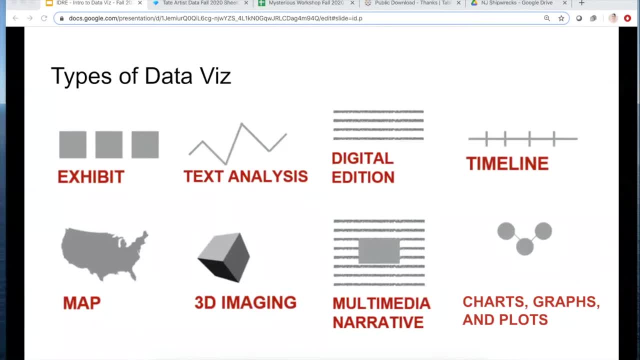 data viz you will choose to use will depend on what type of data you are working with and the goals for what you want to communicate about that data. So, as someone who comes out of museums, if I'm thinking about a digital exhibit- right, I'm thinking about a digital exhibit. 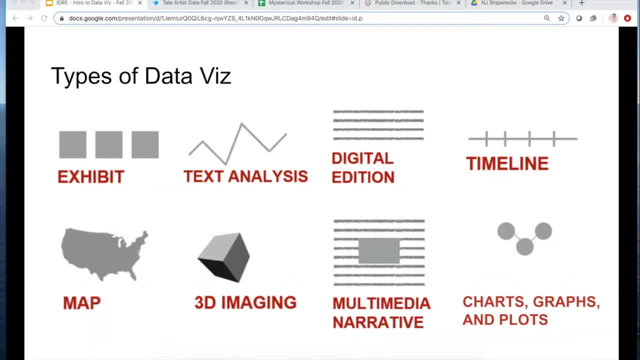 I'm going to be very focused on images For text analysis. we might be looking at trends and wanting to see how often a word is used. Things like digital editions are going to be really focused on how text is displayed for a reader. Timelines: really hard to showcase a large amount. 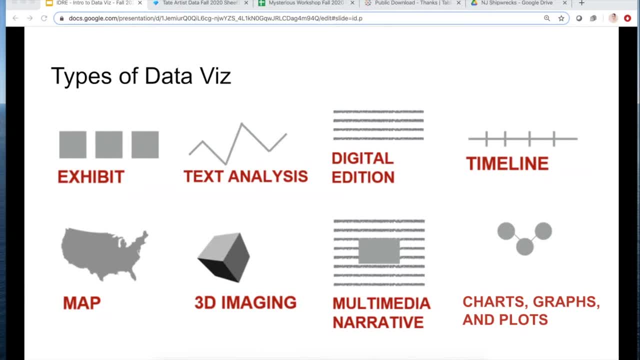 of time on a limited screen space, So the functionality there of how you do that really matters, And so on and so forth we can see here. Are there any others that people don't see on this list? I'm always curious if there's other types of data, viz that people are working on, perhaps things. 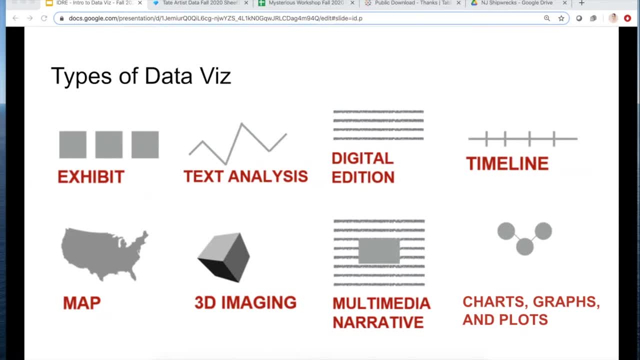 like word cloud. Maybe you want to put in the chat or unmute yourself and share. That's okay. If something comes to you, feel free to share it in the chat, But today we're really going to be focusing on the data viz. 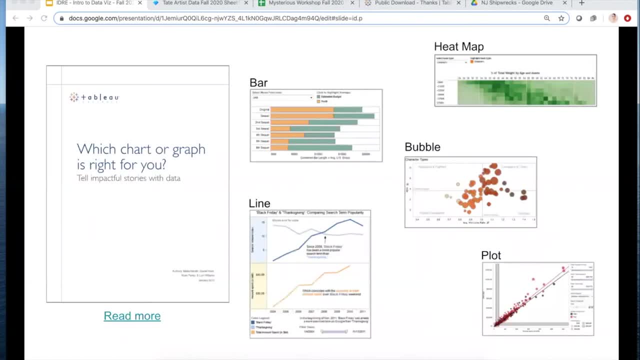 We're going to be focusing on charts, graphs and plots. So some of the most common data visualizations are graphs, which in one of the types of data vizs today, which is one of the types of data vizs we'll be making today, and they form a subgroup. 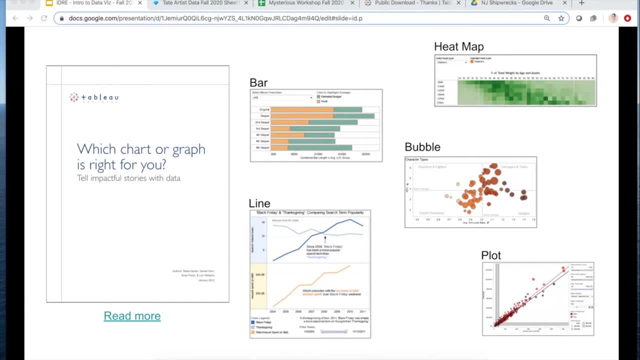 of charts, So graphs specifically present mathematical relationships in data sets. In other words, graphs make pictures of numerical, numerical information. Graphs can be simple and they can be quite complicated, but they should always be selected to present their data as clearly as possible. 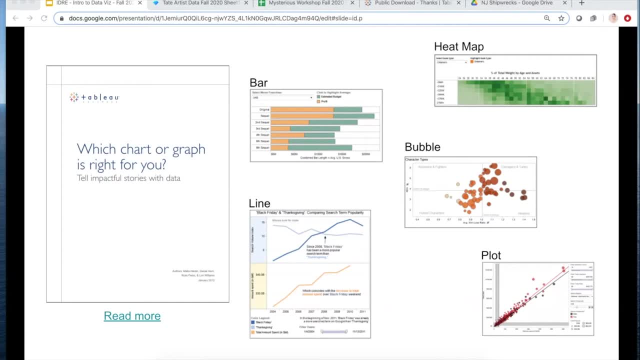 So keep in mind that sometimes two graphs are better than one if each graph shows a different aspect of the same data set. Plots are another type of data viz and they're different than graphs in a few cases. Plots are another type of data viz and they're different than graphs in a few cases. 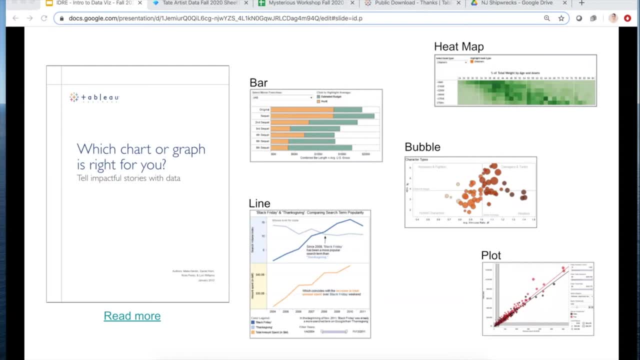 Plots are another type of data, viz and they're different than graphs in a few cases, key ways. So we make plots out of points and for something to be a plot, both axis axes must be continuous. For example, you can make a plot of a height, of the height versus weight of a population. 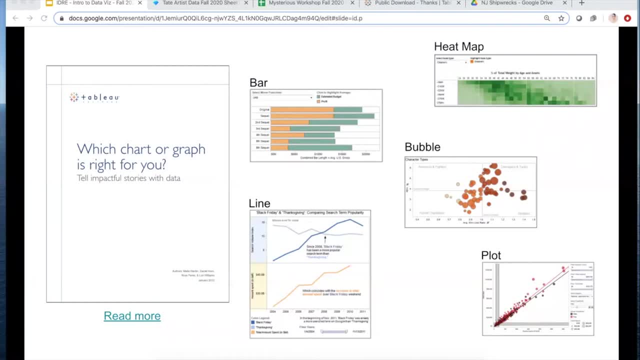 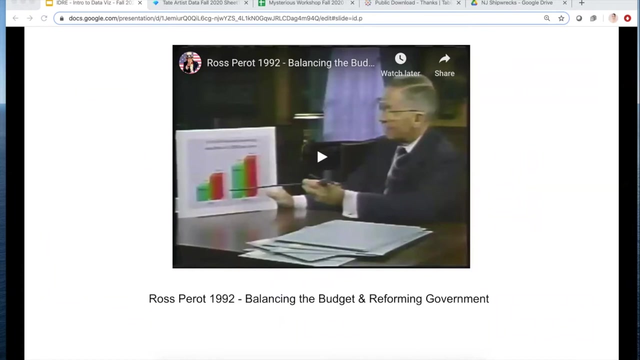 but not the height versus the species, because species are discrete. So you can't plot a point halfway between a cow and a chicken, right? Does that make sense? So I'd say that plots are a subset of charts and graphs. So now that we sort of have that basis, I want us to think a little. 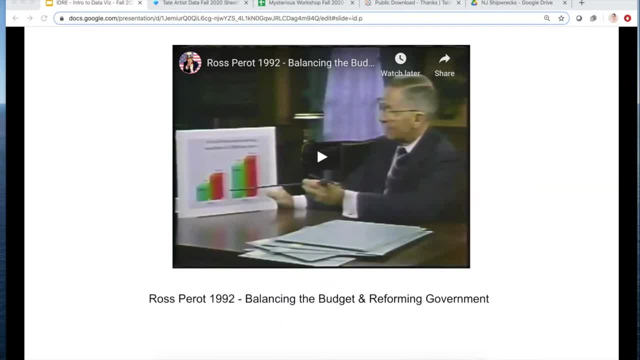 bit about why do we visualize and why is visualization so popular. now, before we jump into doing some visualizations ourself, We tend to think that information graphics have some special access to the truth and that they simply present fact. And since we're in the middle of an upcoming election, and I hope everybody is- 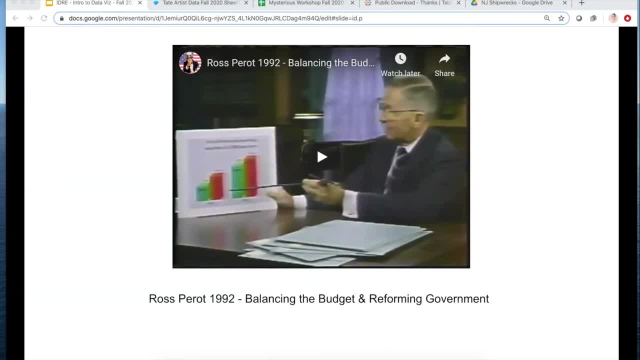 registered to vote and if you haven't done so already, so quick plug on that. It's a great right that we have and we should all do it if we're able. So this is an example of another billionaire that was running for office in 1992.. 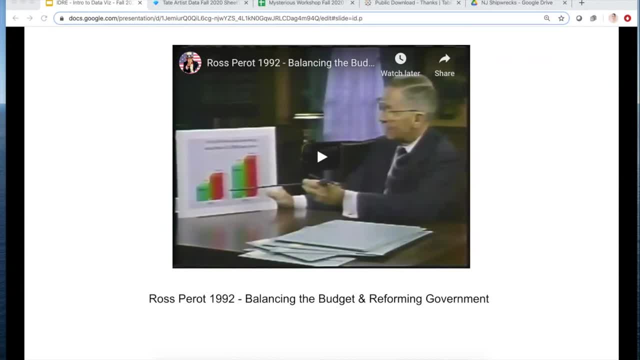 His name was Ross Perot. for some of you who may remember, Many of you were probably not even born, But, for example, this is one of several of his infomercials that ran during the 1992 general election campaign And he was known for these charts that he would use And what stands out. 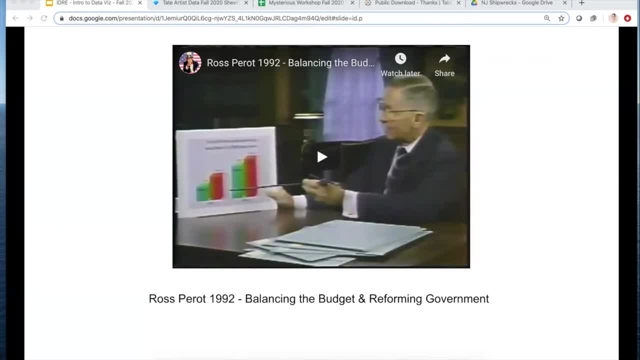 of in his presentation. I won't play it for you now again. I'll let you enjoy that on your own. but what stands out about his presentation and his use of these charts and graphs is that these numbers seem definite. right They seem to be. he seems to be an authority on all these. 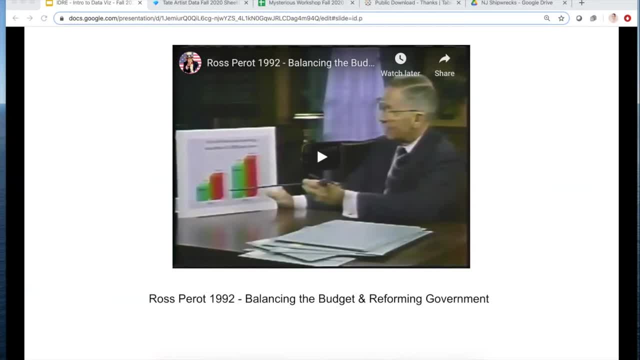 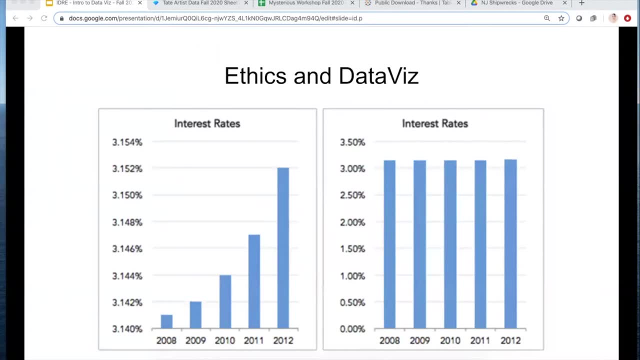 subjects and he has a certain command of the facts. But compare these two graphs and tell me what you see, or just take a moment and look at these two graphs. Does anybody catch what the difference is here? Can you either type in the chat or unmute yourself? Yeah, So. 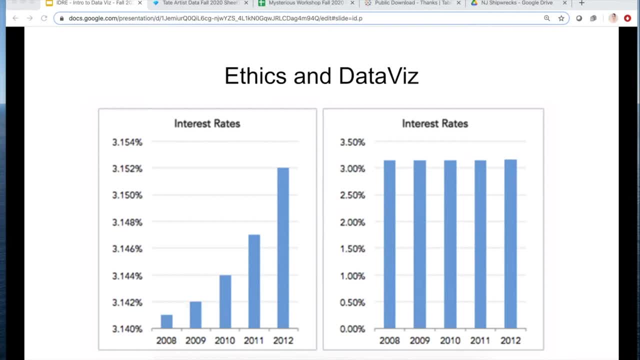 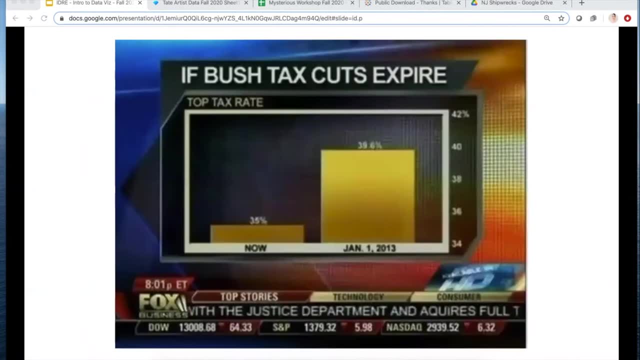 Ruben, Tony, yes, Everyone's noting scale. Scale affects drastically how we interpret this information. So, for instance in this one, what's confusing or problematic here? Well, we're topping out at 42%, which is a fairly arbitrary. 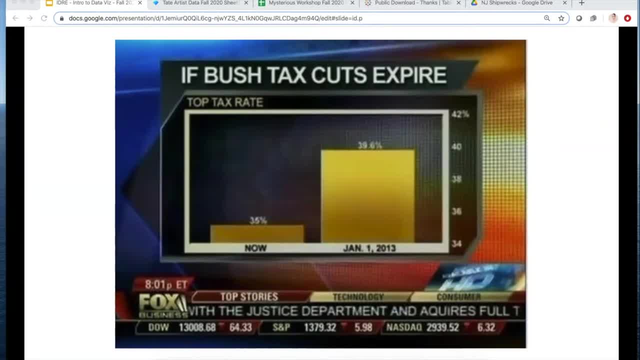 number. So we're topping out at 42%, which is a fairly arbitrary number. So we're topping out at 42%, which is a fairly arbitrary number, for a stopping point at least. Percents are normally out of 100, right? So 42% is kind of a strange point to cut us off, Even if this was simply. 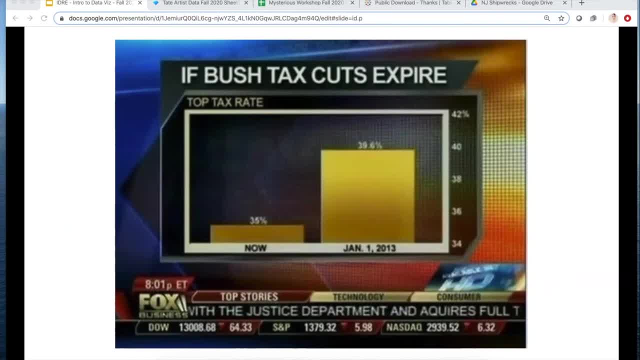 zoomed in to help us physically read the chart better. the result is that it looks like a drastic change. The other thing to note is that the use of now in the labeling is not very helpful. right, We're not really sure what the time difference is between January 1st 2013 and whatever now is, So labeling is 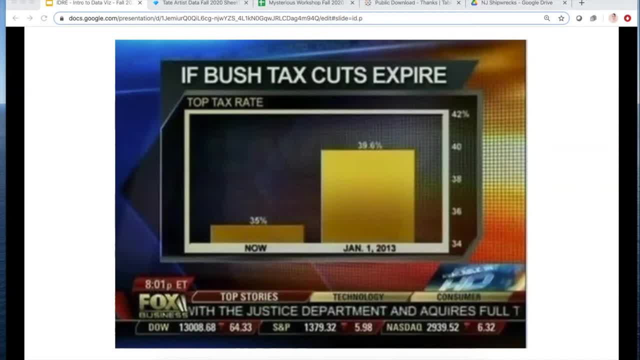 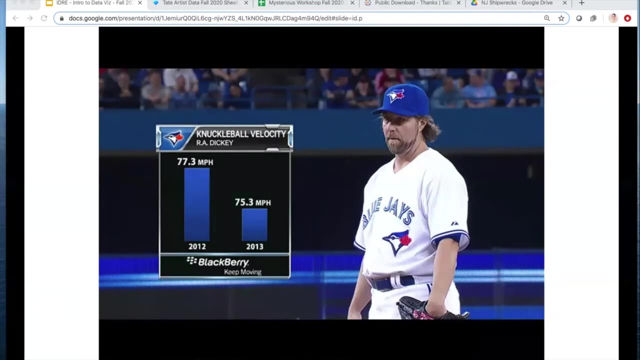 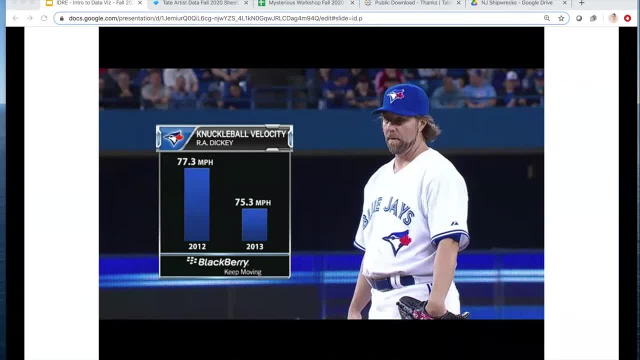 The only what we're seeing in this one is only showing us a two year span, which is a very limited window, And you want to avoid that. We can't really know, without additional context, if this is such a drastic dip in performance as it appears here. 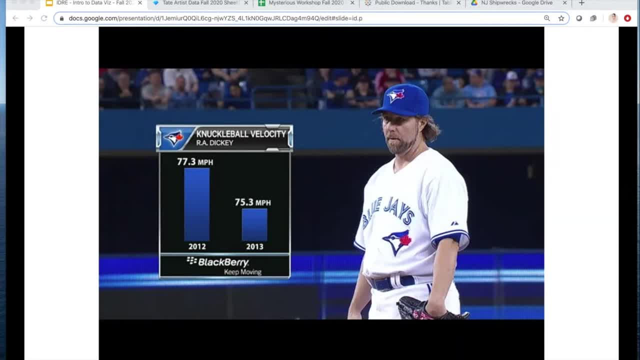 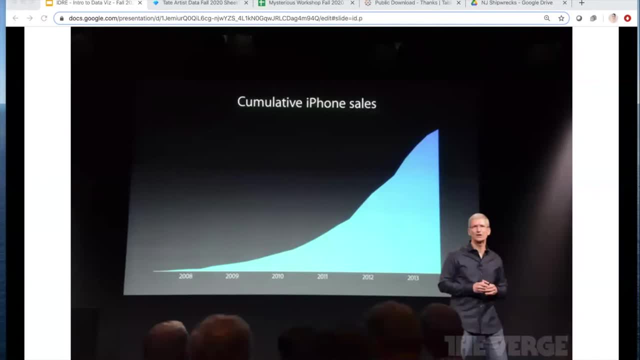 Unless you're really familiar with baseball and this particular player. you need more context to understand the significance, And a visualization is not just about the graphics. Like I've pointed out in these past couple of slides, labels and titles are really important to pay attention to. 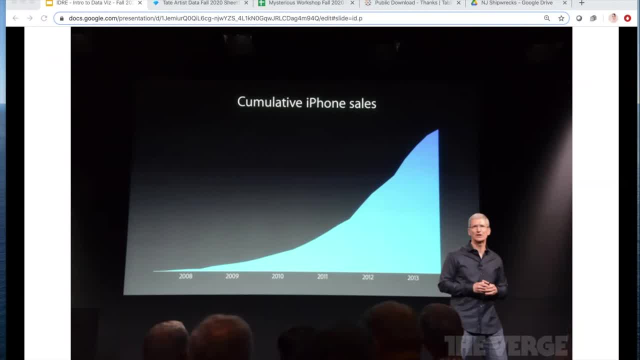 So cumulative, as you see at the top here, can shift a line graph quite drastically and obfuscate what might be the more useful information, depending on what you're researching. So this tactic is fairly commonplace, particularly in business. So when you're reading and creating data visualizations, it's important to be clear on what is being communicated and why. 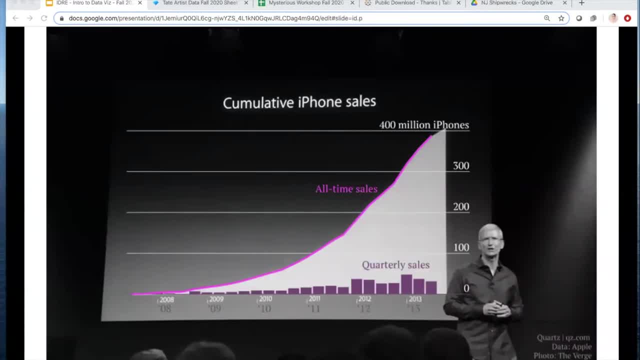 And just to show you the difference here, without the use of the cumulative approach or adding together of the numbers over the years, the graph actually looks like this: That steep slope is showing us the growth of all time Sales. so past years and present numbers added together that looks very different from the quarterly sales that are happening in this version. 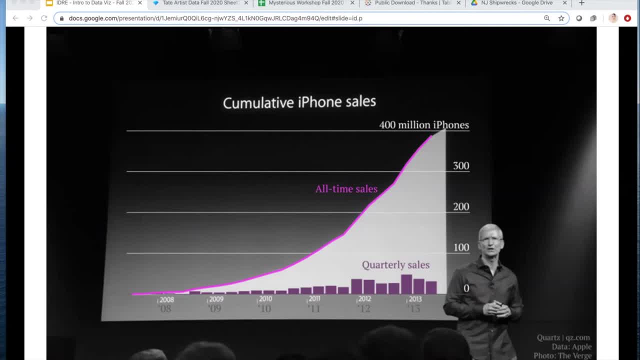 And this is the difference between looking at something from a sweeping overview position versus a more granular perspective, And I'm not putting a value on either one of these things. It just depends on what you're trying to communicate to your audience. So these contexts become critically important. 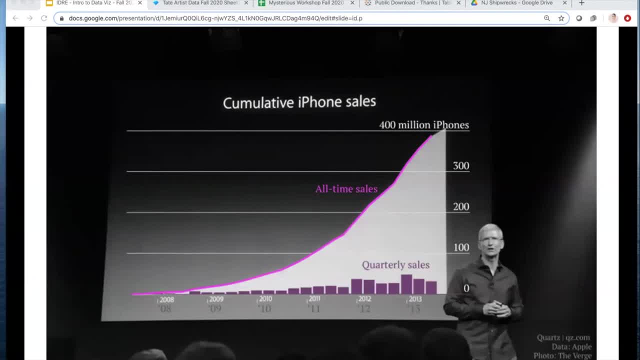 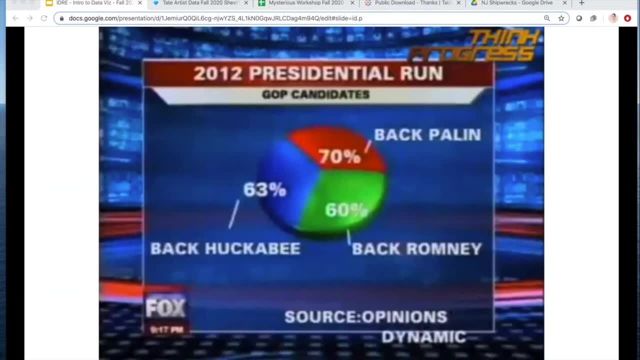 When Your data will be, or how your data will be read and understood. And then just finally, to wrap this up, before we get into our own hands on portion, there's the simple matter of getting your figures right. So you'll be amazed at how many times people just forget to sort of proofread things as you would. you know a paper that you turned in for a class. you want to have people check your numbers. 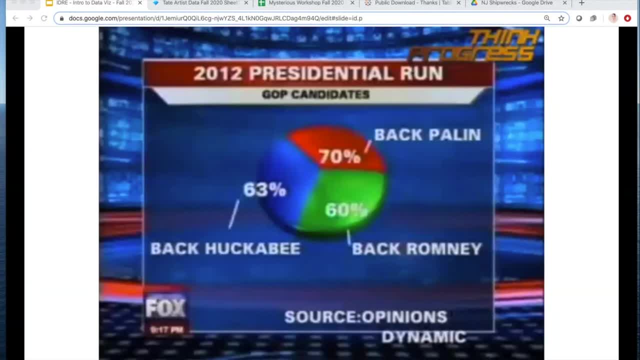 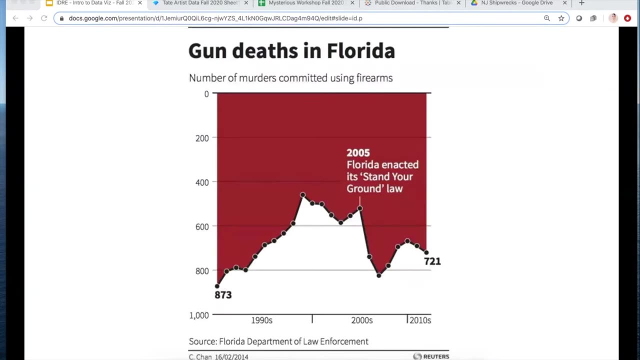 And make sure that everything's adding up correctly. This is a little blurry, but I think we can all see that a pie chart has to add up to 100%, So obviously these percentages are off and then remain always on the lookout for more dubious stuff. 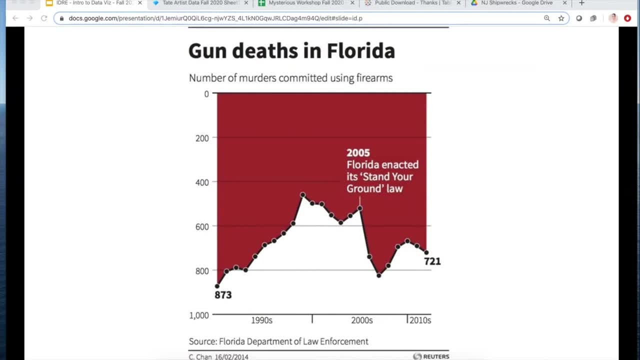 I'll give people a second to take this thing. Can anyone tell what's going on here? Yeah, sure, Yeah, sure, Yeah, Yeah. Seventy Seven, 721 is higher than eight. Yeah, 873.. It feels upside down. 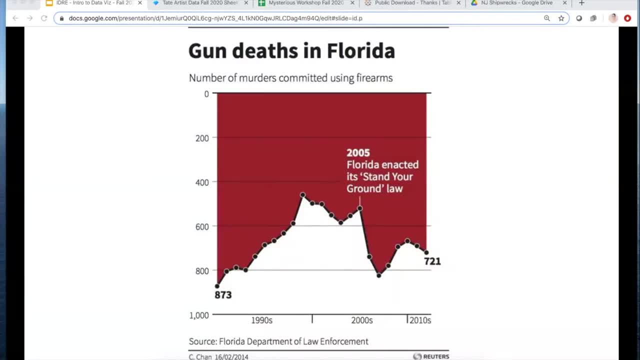 Exactly So they. they switched what's common practice, which is to put the zero down on the bottom in the left corner, and they put it at the top on the right, So it flips the graph. So best were common practices, Right. 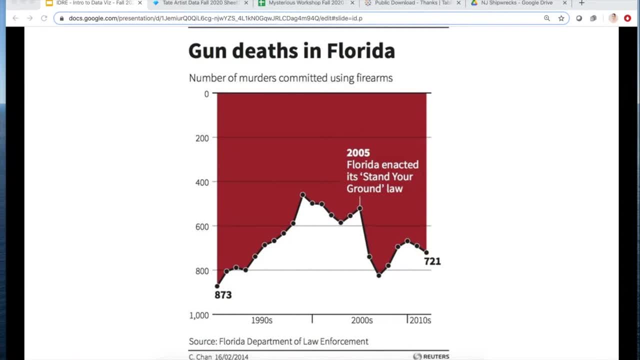 Awesome, Thank you. can be used against a less keen observer And we have standardized visualizations enough that we hold certain assumptions about how they usually operate. So these things are zero goes at the bottom, not at the top. We read from right to left. typically, People may manipulate these. 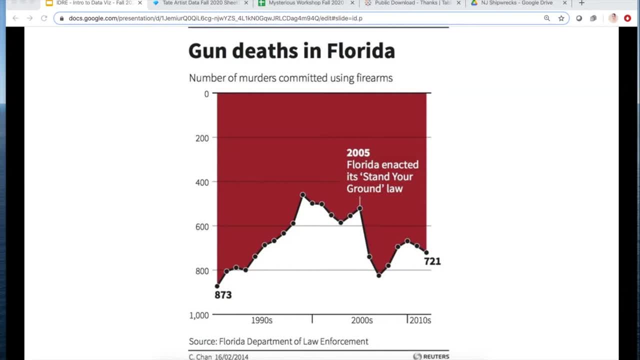 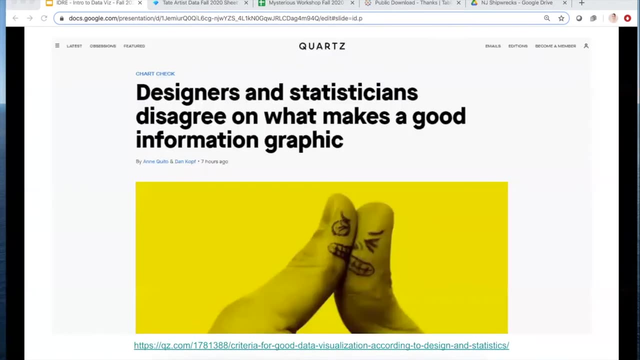 elements to suit their outcome, So we want to keep an eye out for them. A good data viz reader will always be checking these details and following common and best practices to ensure a graph is read correctly with as little effort as possible. So what I hope these problematic data visualizations highlight is that there is a 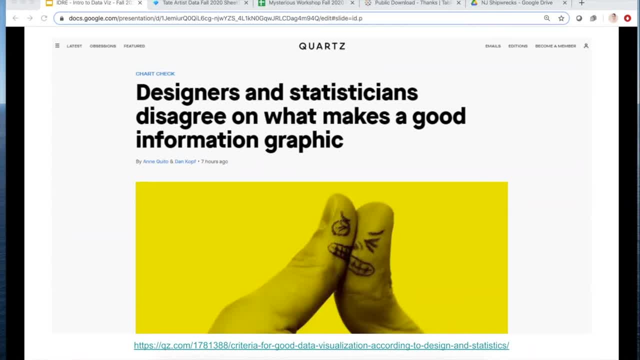 tension between design and data when representing data visually, And we don't always agree what makes a good visualization. This is a fairly recent article that covers that debate, so I recommend taking a look at it. In it, the author describes that designers often feel it's. 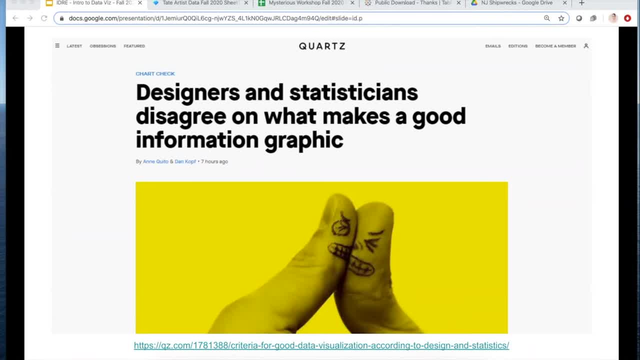 important to make sure the graph grabs and holds your attention and is intuitive to navigate. Statisticians or data scientists, on the other hand, want data visualizations to clearly communicate the data, But beauty and accuracy don't have to be at odds, And I hope that's part of what you. 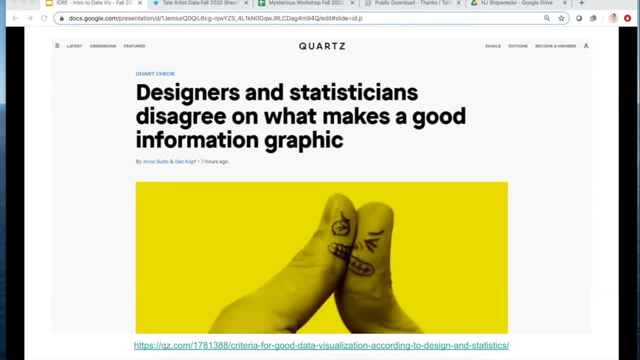 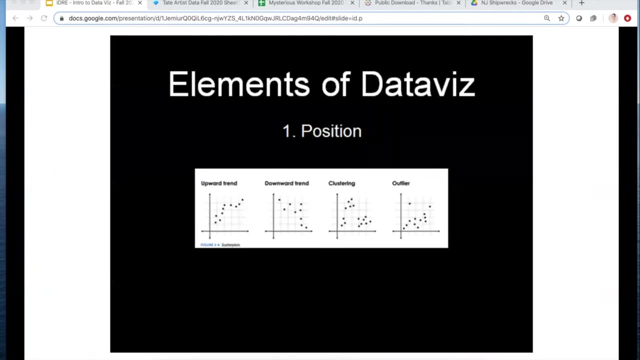 take away from today's webinar, Thank you. What we saw in those problematic data visualizations is how both design and sometimes numbers can fail us. So let's start first with some of the design elements that are critical in making data visualizations. So we've seen from some of these bad data visualizations, certain design elements. 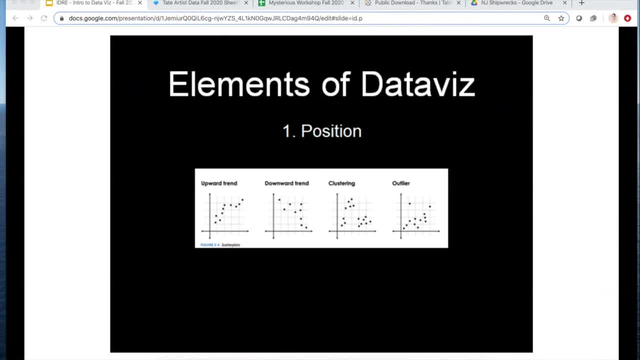 that can be very crucial in data visualization, And the first and foremost of that is position. When we talk about position, we tend to be looking for something that's going to be a value, And so we're going to look at a certain value. that's going to be a value, of course, because we're going to want to see if that value is in our data visualization. So let's start with some of the 굉장히 different data visualizations that we see in these�� GRE at a give-all consultations: finger bearings, computer line visualization abilities that we see when we talk about ground and or data visualization. 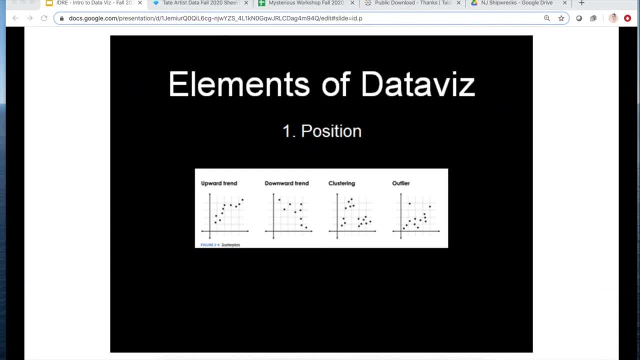 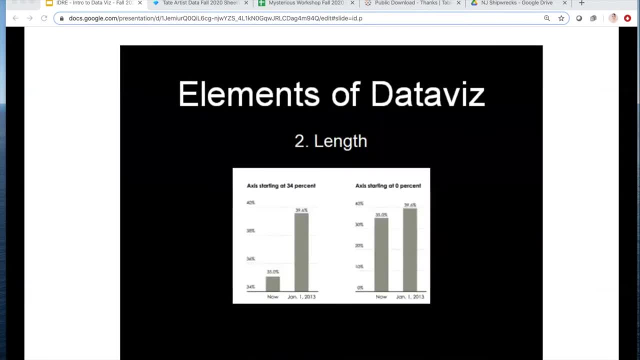 to be looking for things like upward or downward trends, clusters, or if there are any outliers. If you remember from the first comparative graph I showed, changing the scale shifted the appearance of the graph's bars, So the distance between or length was further emphasized, and we tend to 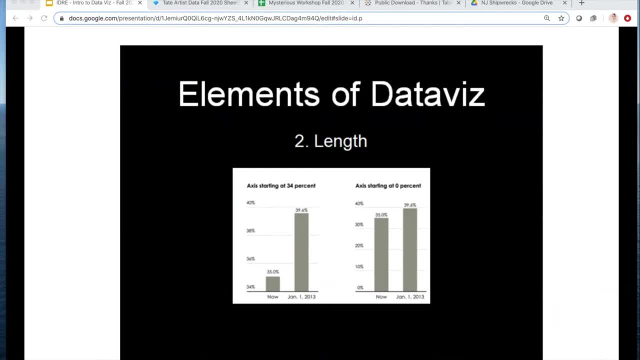 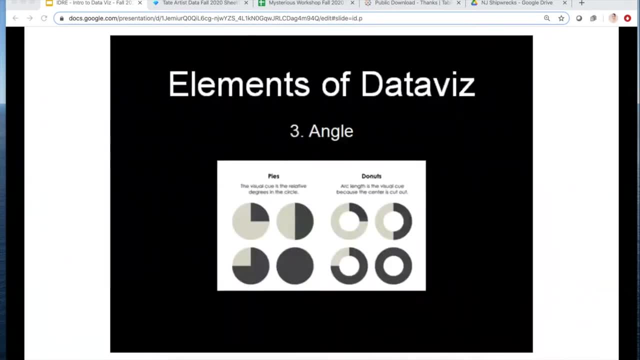 interpret that as significant. The greater the distance, the more significance we assign to the difference. Angle is very useful in communicating a part in relationship to a whole. So when you're thinking about trying to show the percentage of something, angles are really good for that. 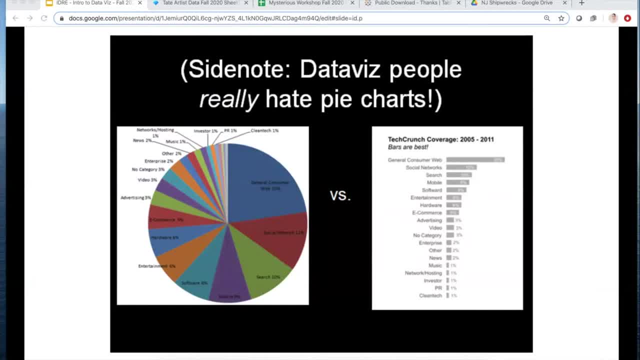 But we should keep in mind that pie charts are notoriously hated within the data viz community and are usually thought to be illegible after about five slices. So keep that in mind before choosing to make a pie chart. Even though bar charts are boring, they can communicate. 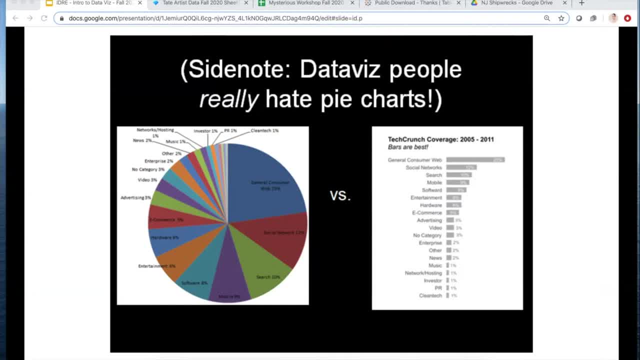 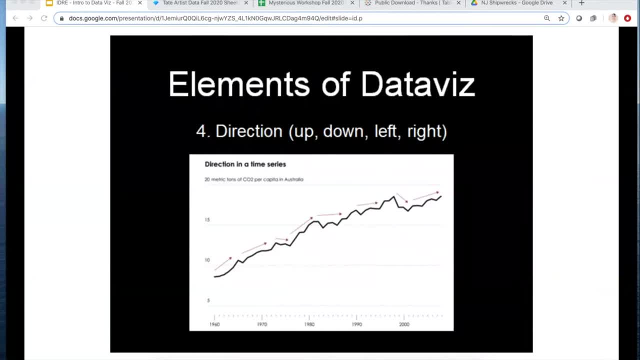 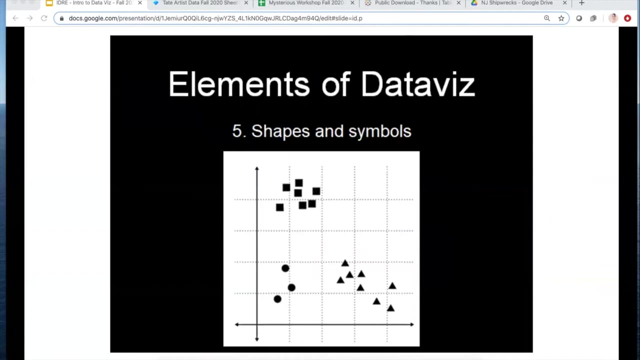 much more clearly than a pie chart with too many slices And most data visualizations are read from, like I said, left to right and down to up. So shapes can be extremely useful in representing different types of data. They catch the eye and signal difference really quickly to the viewer. 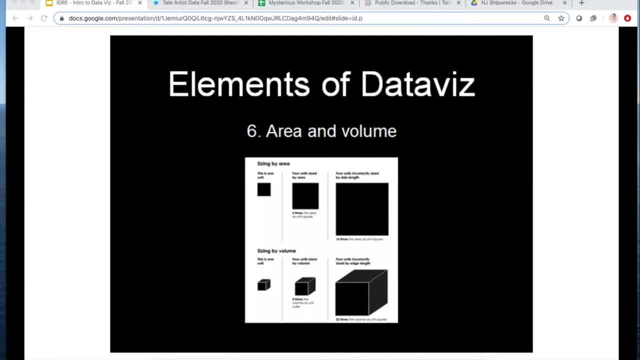 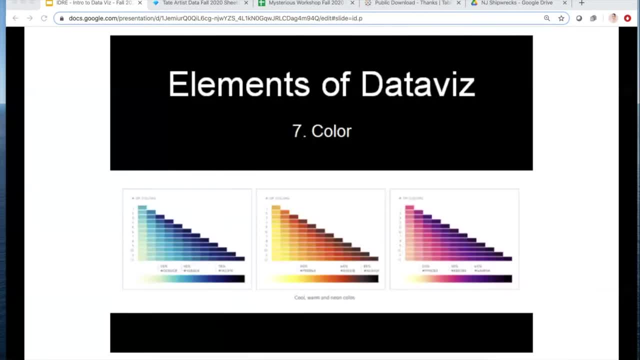 And likewise area and volume, help us compare. if something is larger or smaller at a glance In terms of color blindness, you only have to enter red for them, Because if it is too dark, that means if you're using color blindness, then you're more likely to. 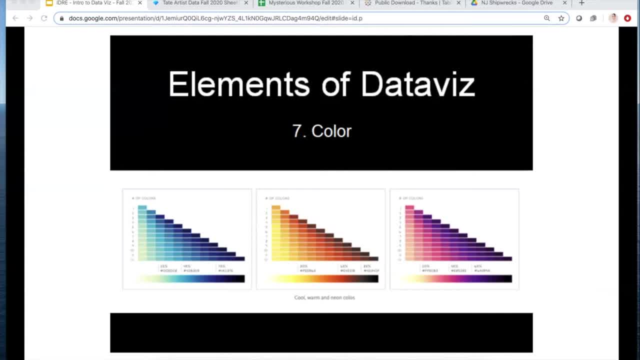 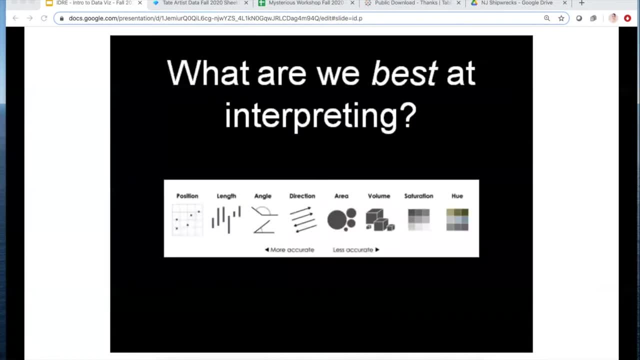 spot more of the colors- For example, this is the image start- than others. um, if you see, those things to the left of center are what we're better at interpreting. so position is something that we're really good at interpreting, whereas saturation and hue we're less good at interpreting. 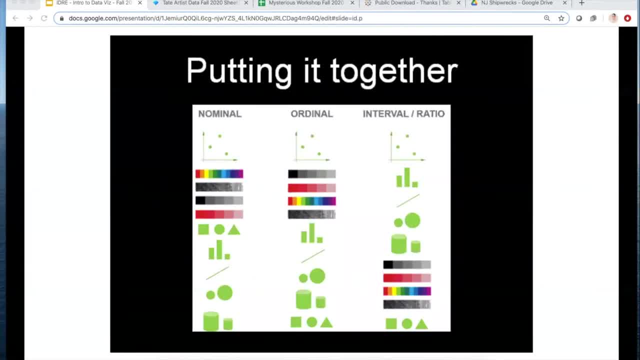 and here's what happens when we put the approaches together from a designer's- um, from both the designers and statisticians point of view, right position, no matter what is going to be critical. but when you're working with something like nominal and ordinal data, those sort of differences that are highlighted in the type of data are going to. you want to. 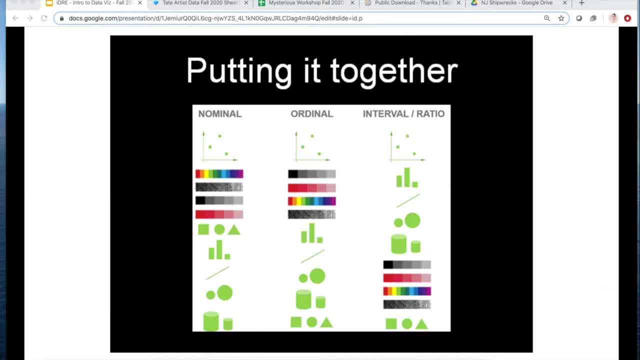 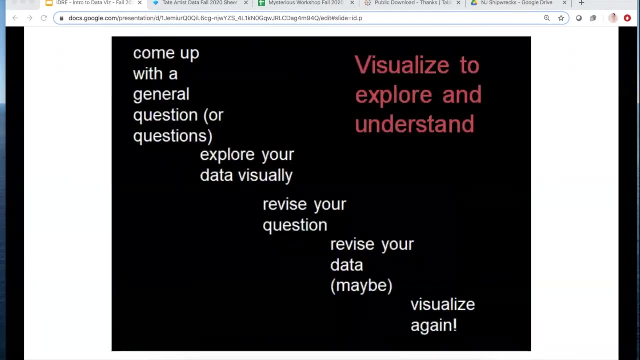 accentuate those things through things like color and hue, even though that those things are harder to read by the eye. they help communicate more quickly that level of difference, whereas an intellectual in ratio, things like length and direction become increasingly important. does that make sense to everybody? i'm gonna sort of wrap this portion up as we head into our, our hands-on, but um, 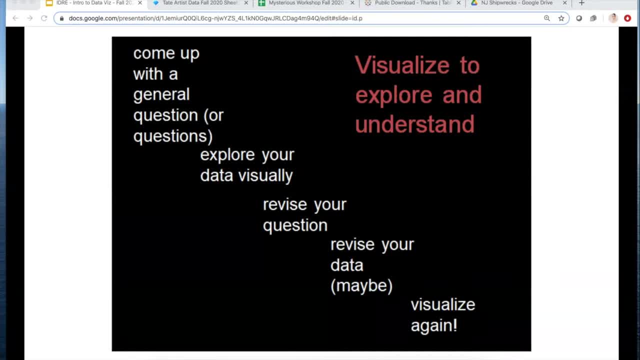 please let me know if i'm i'm going too fast. i just want to sort of get everyone on the same page here on how we combined both design and data together. and when we think about the process, um, it often looks something like this: so we come up with a general question or set of questions. 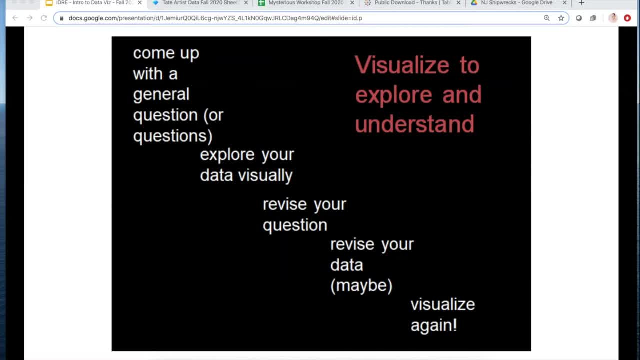 for our data and then we often explore the data visually. this is an iterative thing. you don't sort of put your data into a data tool and come out with a visualization of the data, and then you come up with a question and that's your final product right away. it's often an exploratory process. 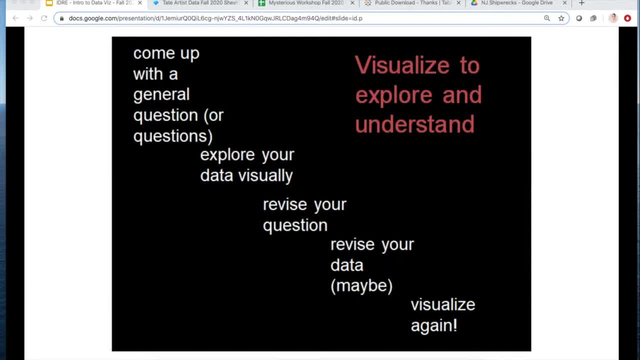 and so you may see something in those first visualizations that will cause you to go back and revise your question and maybe even revise your data. maybe there's a certain area of the data that you need to find out an additional data type to help support it, to visualize it properly. so 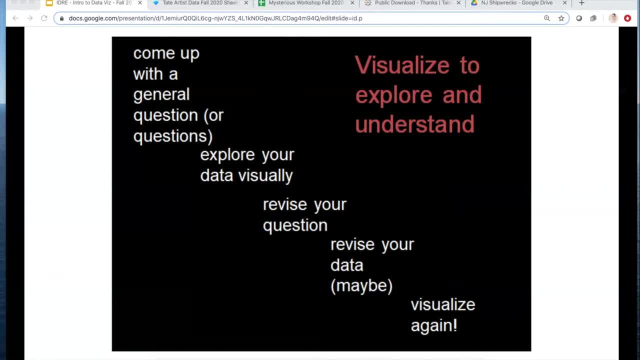 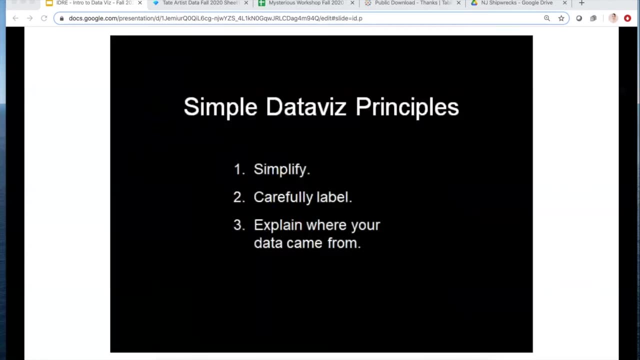 you'll want to go back in and create various data sets or versions of your data set to visualize it, and you visualize it again and you might go back and do it again. so it's it's iterative, it's it's cyclical in that way. but the three basic principles i want us to as we get into using tools is: 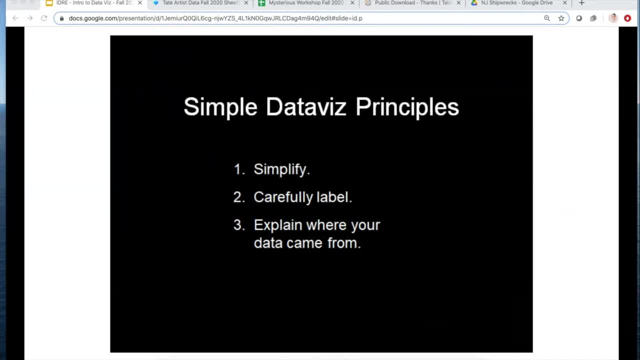 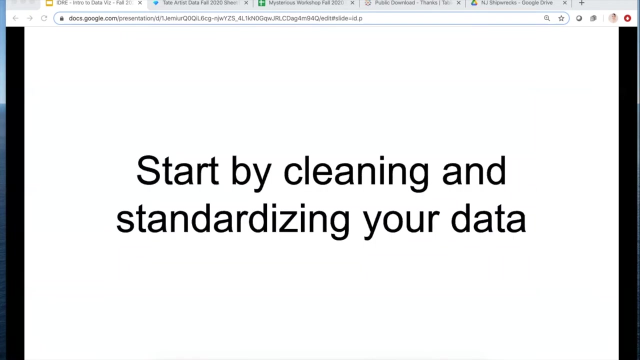 um that to make strong data sets, we need to keep things simple, carefully label and explain where your data comes from. If you do those three things, you're always going to have a fairly strong data visualization. Okay, so, as I was saying, all good data visualizations start by cleaning and standardizing your data. 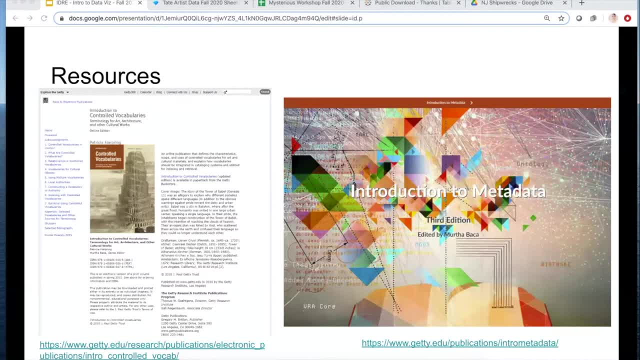 So how you organize and label your data matters- It matters a great deal. The terms you use matter. Each field or discipline in academia has its own standards, so you'll always have to do some research on that when you're getting started. But I wanted to show these examples. 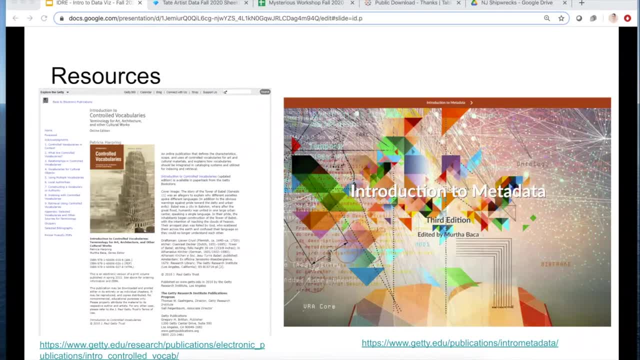 So, for example, in the Library of Congress, it has its own list of authority terms for subject headings, and those are the words that you use when you go to look up a book by subject matter. So that's one example. But these examples here and what I'm going to show you today, 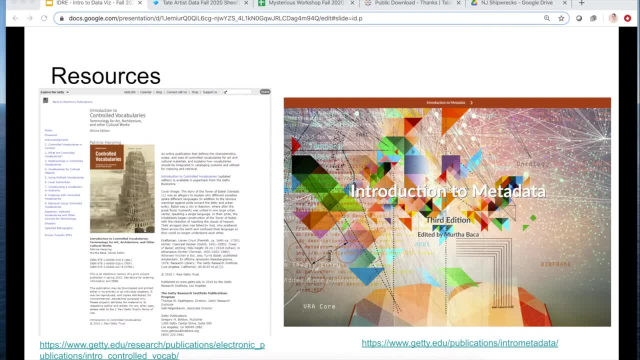 is how you can use another authority known as the Getty Thesauri or the Getty vocabularies, with a tool called OpenRefine to help you clean and standardize your data. This is really great for cultural artifacts, but you'll find these types of things in all types of disciplines. 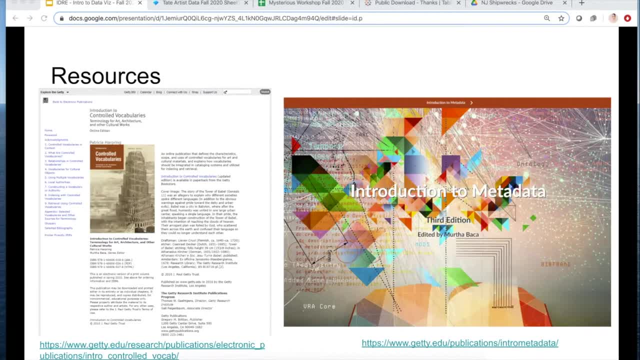 There's always going to be those who have metadata standards in your field, so you'll want to research that. That being said, these two resources are freely available and they're great introductory resources that anyone can use. You can probably get through them in about a day or so. 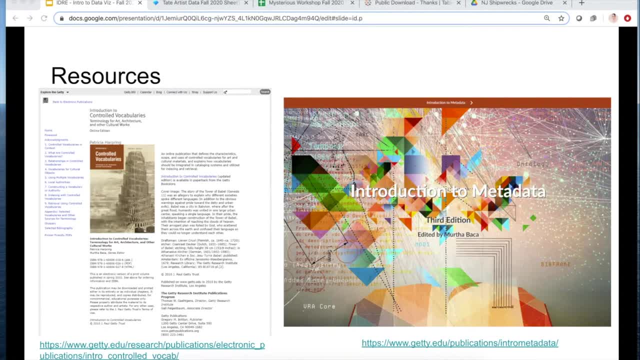 They're quick reads, but they're really great for understanding best practices around structuring and standardizing your data. So one is introduction to controlled vocabularies and the other is introduction to metadata. They're both freely available online, so definitely check those out. 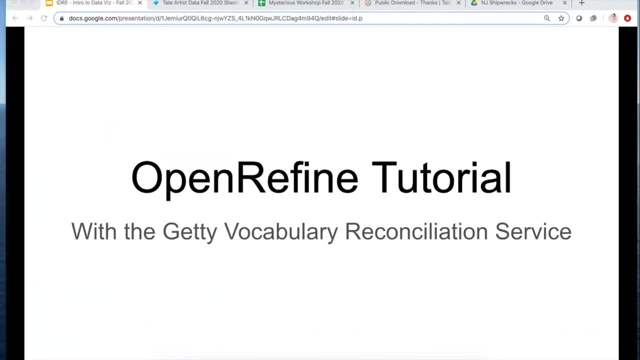 So with that, we're going to jump into our tutorial portion. If you haven't had a chance to, we're going to download some software if you need to do that, but there are many different ways to clean and standardize your data. 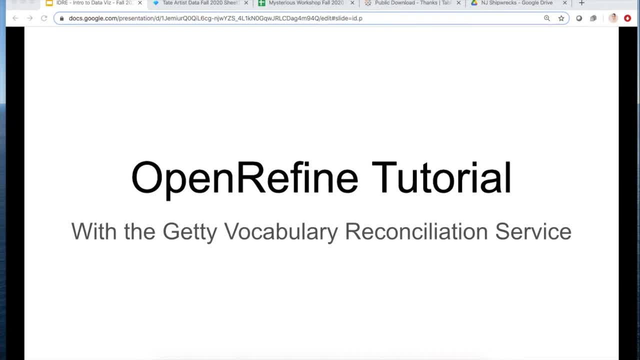 Excel and Google have some things built in, but I want to recommend OpenRefine, which is free and open source. like I said before, It can help you do transformations on data in a few clicks and it's very powerful in that sense. 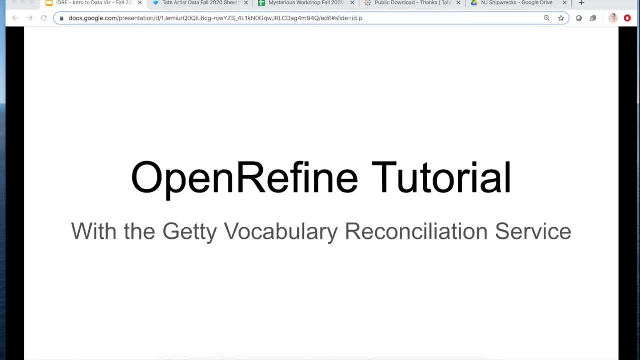 especially if you're working with large data sets. There's a bit of a learning curve, so we'll just familiarize ourselves with some of the basic functions and then do a test on how we can pull from an authority source to do some more powerful stuff. 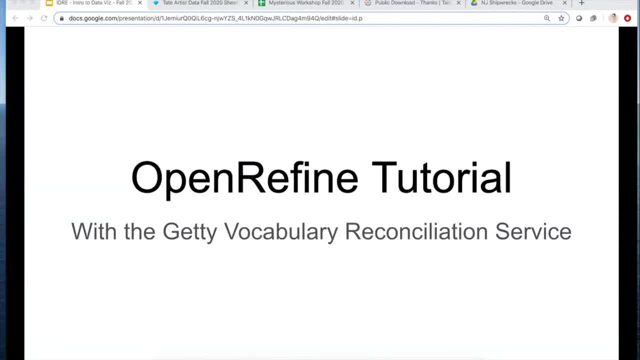 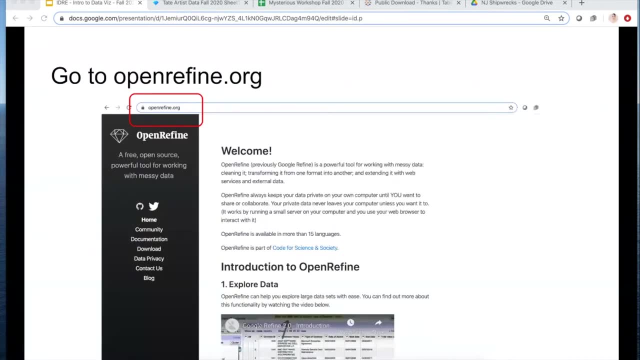 But again, this is more of a visualization workshop than a data cleaning workshop, but I just wanted to sort of expose everyone to this so you know what's out there. So if you didn't get a chance to beforehand, or if you didn't see my email, I sent out in advance of the workshop. 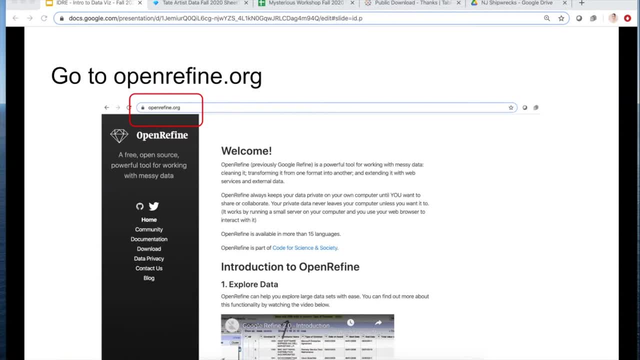 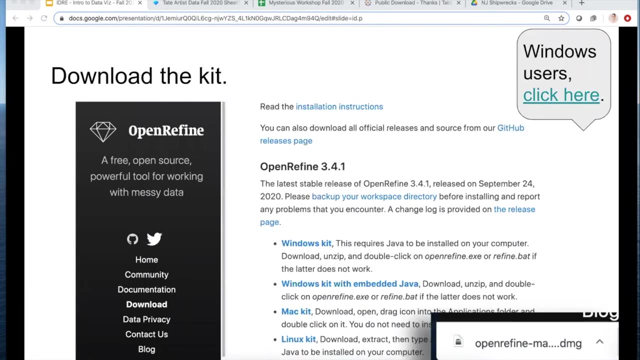 please feel free now to go to openrefineorg and download the software, So I'm giving everyone a second to do that. Once you're there, you'll select the download option from the left column and choose a version for either Windows. 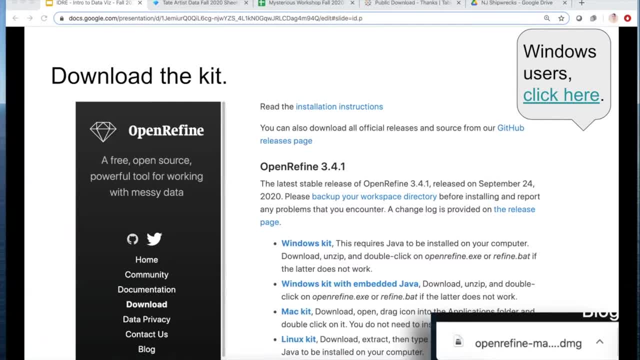 Mac or Linux, depending on your operating system, And for this demonstration I'm using the latest Mac kit, which is version 3.4.1.. And just a side note: while you're doing that, for each project, all users should always use the same version. 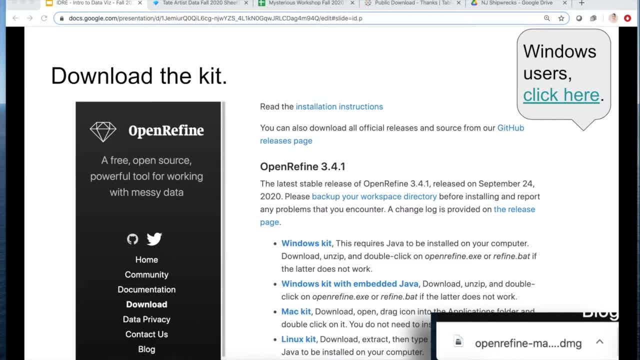 of OpenRefine. For example, if two people are editing a project using OpenRefine, one person should not use version 3.2. If the other person is using version 3.3, that's going to cause you some issues. 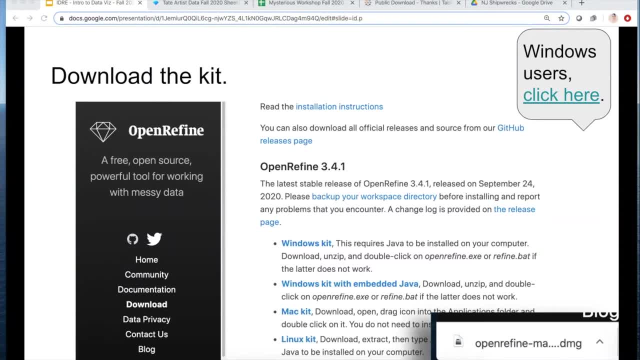 So you want to make sure that you're always using the same type or same version of OpenRefine, especially when you're switching or working on a shared project together and sharing files. So download from there, And this is just a side note. 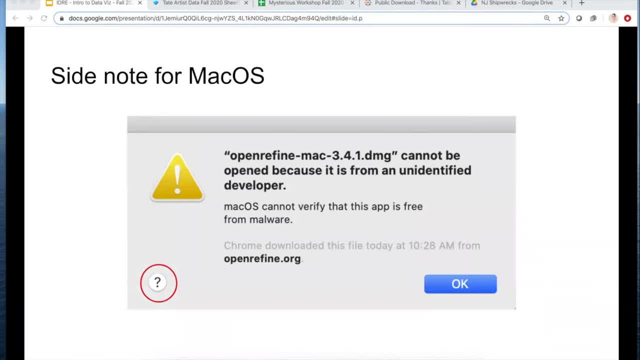 There may be a security pop-up that you encounter on Mac OS. Since it's a public software, you'll have to go into your security and privacy settings on your machine to enable it. So select the question mark icon in the warning message to be directed to instructions on how you can allow the software through your security settings. 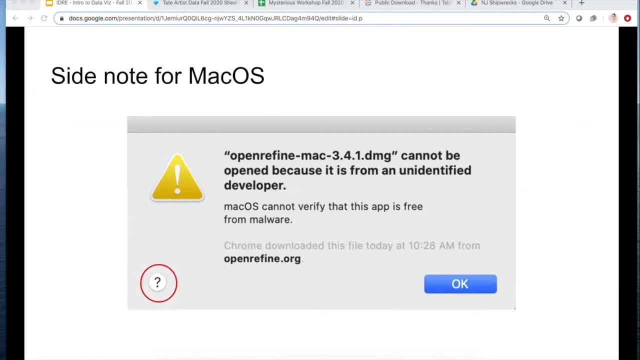 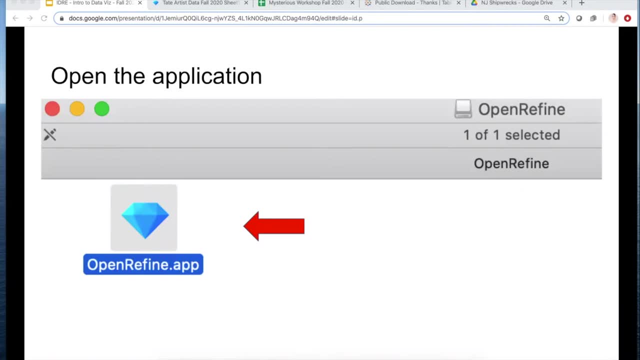 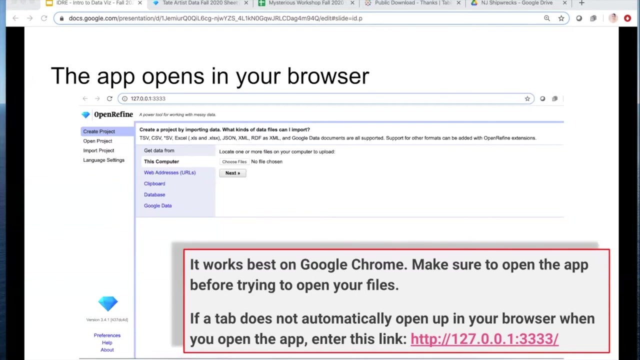 And that's it. Thanks for watching. I'll see you next time. And once you've done that, double-click on the icon to open the application. Does anyone need a second more to download things? Are people feeling that they've got a good handle on that? 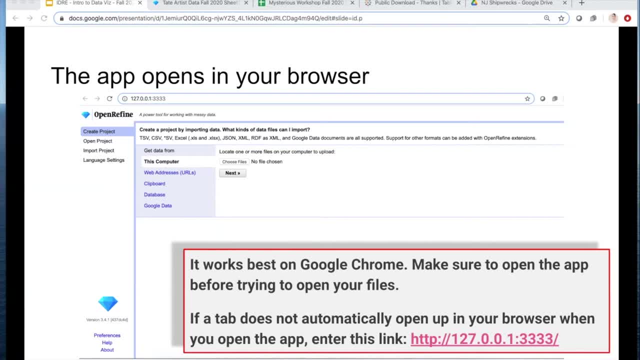 Yeah, Okay, great. So once the app opens in your browser, you should see something like this: And just to note, it works best on Google Chrome. So make sure to open the app before trying to open your files, If a tab does not automatically open in your browser when you open the app. 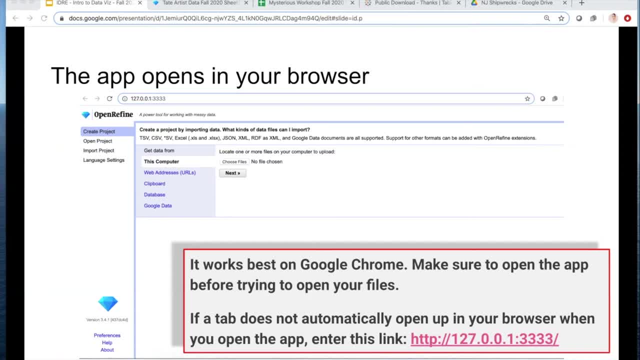 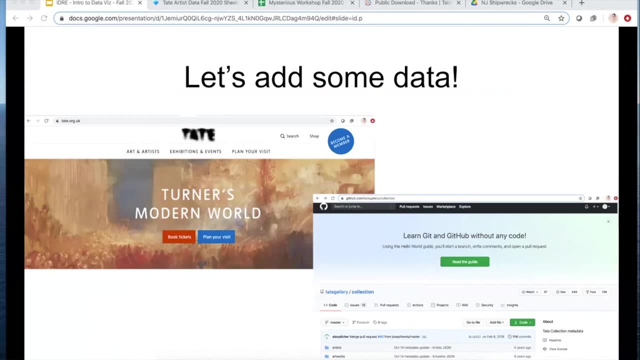 you can also enter this link or I'll show in another slide an alternative. But it's a browser-based application, So you're going to see it in your web browser. So let's add some data. The Tate Museum in London has put much of their collections data online. 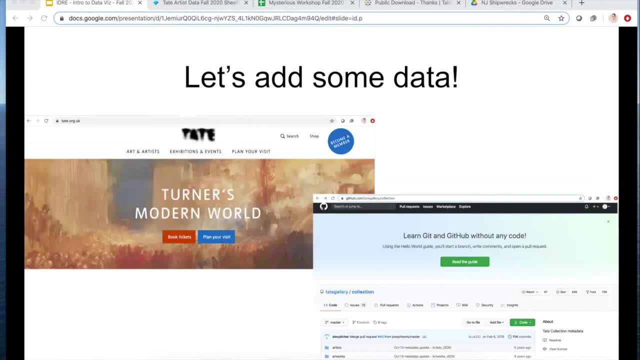 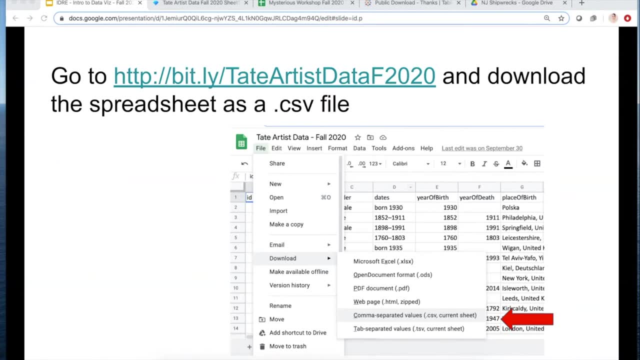 which is great. So we're going to use that for today And you can get to that data by going to bitly slash Tate artists data F2020.. And that will allow you to download the spreadsheet. So once you're there, you'll be able to. 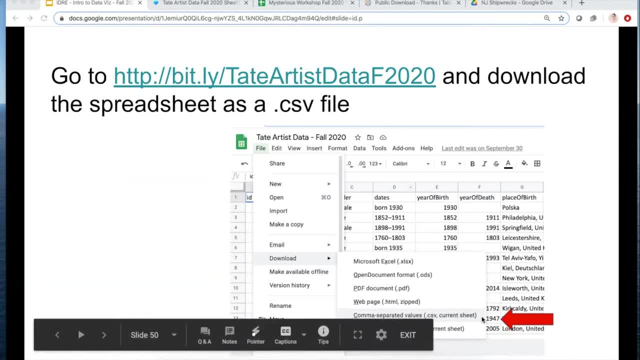 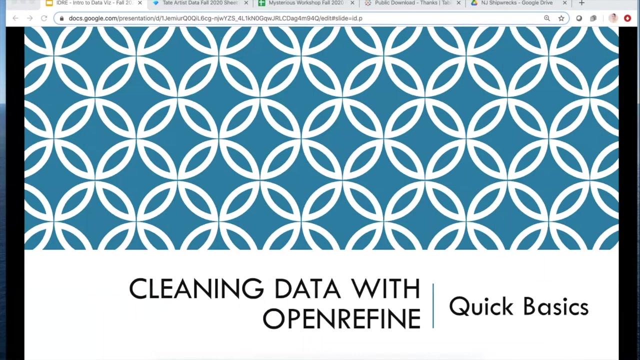 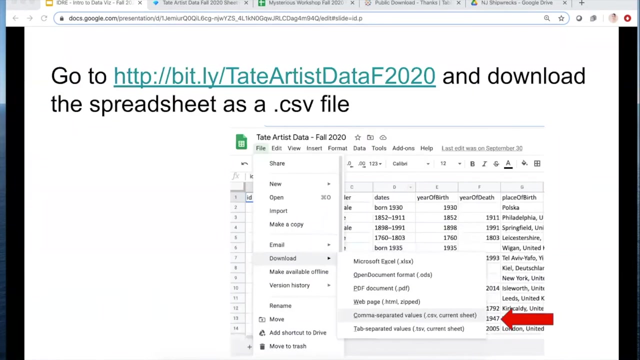 put a file and then download. And you want to download it as a CSV file. Is everybody able to do that? We should say: is anybody not able to do that, Everybody's good, Okay. So while you're doing that, just in case, 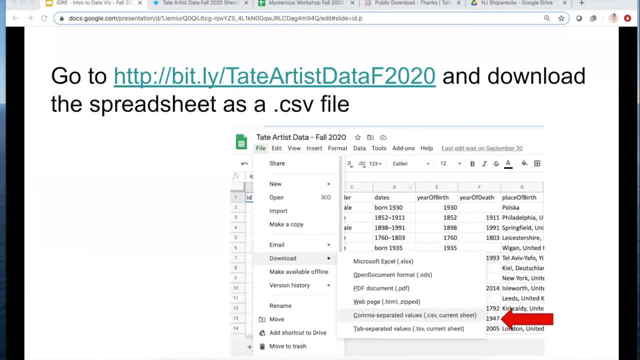 I'm going to run through some quick basics of OpenRefine before we jump into the tutorial on how to reconcile parts of your data using the Getty vocabularies. But this is just sort of a whiz through of the functionality that's available in OpenRefine. 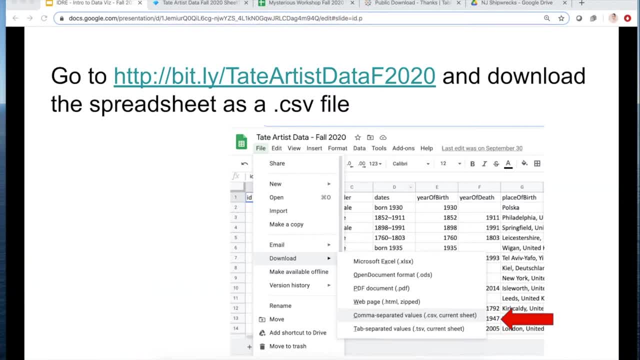 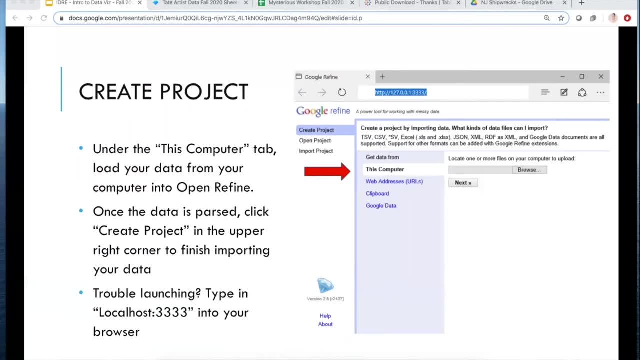 So you can start to envision how you might use it for your own projects. So you'll start by creating a project and inputting your data, like most other programs. You will do this together with your, we'll do this together with our data in a minute. 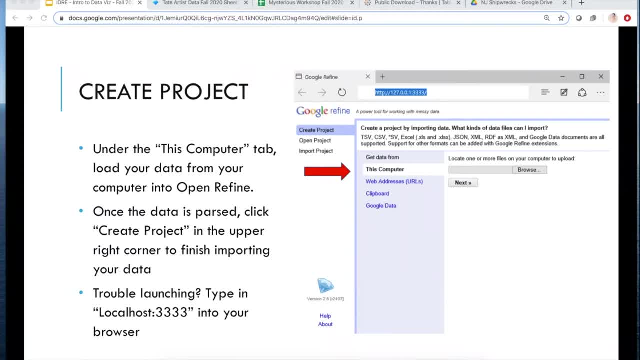 So you don't have to do it right now. But if you ever have trouble launching your program, like I said, you can always type in localhost colon 3333 in your browser and the program should open if you have it downloaded. And what Google Refine or OpenRefine is great for? 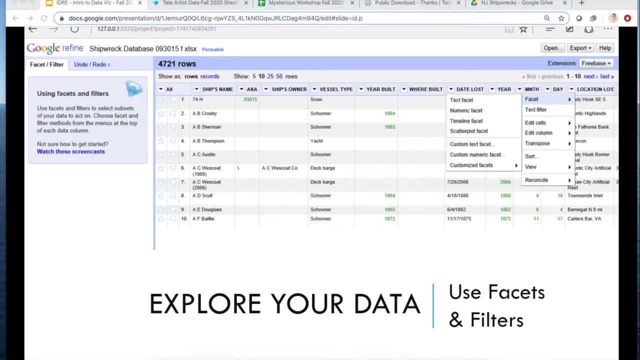 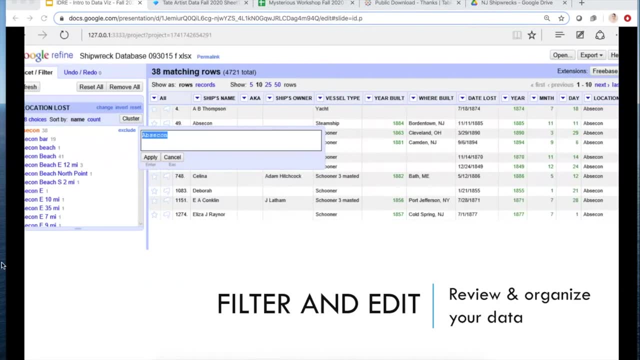 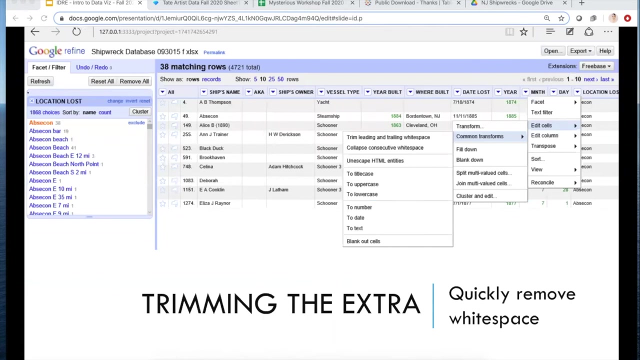 is that it allows you to facet and filter your data quite quickly. This is an example. You can use a cluster function and review and organize your data and apply changes to a large set of data types really quickly. You can trim any extra. So removing white space is always a great place to start. 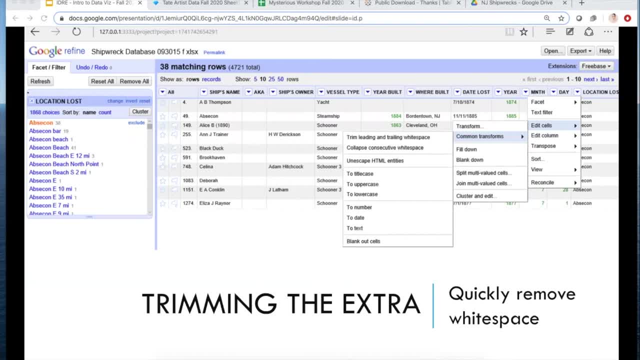 when you're cleaning up data sets. If you've got a new data sheet, the first thing I would tell you to do is make sure that you've removed it's leaving and trailing white space, And that's really easy with OpenRefine. 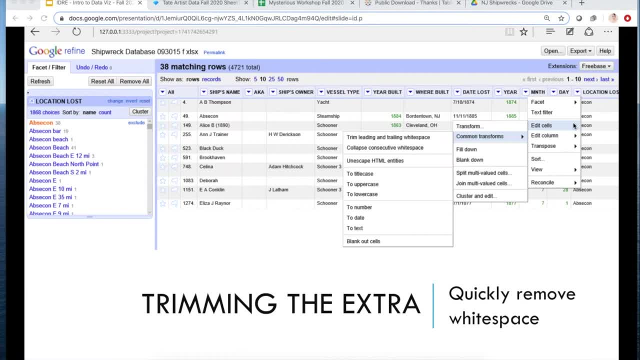 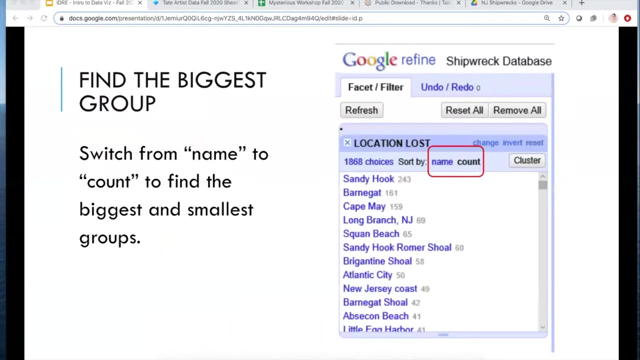 As you can see, you select on these dropdown arrows, you edit slides or edit cells, common transformation- and then you just trim leading and trailing white space. That's how easy it is. You can also find the biggest group quite quickly. So this is again great for getting to know your data and what's there. 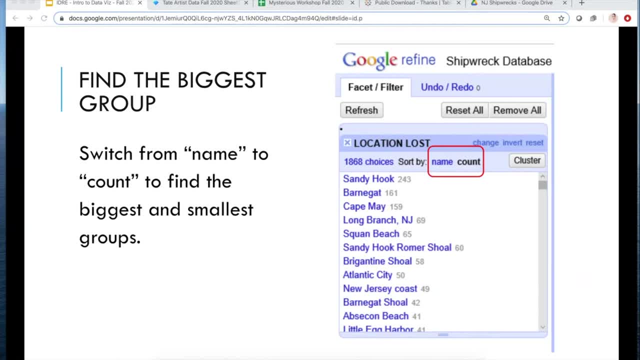 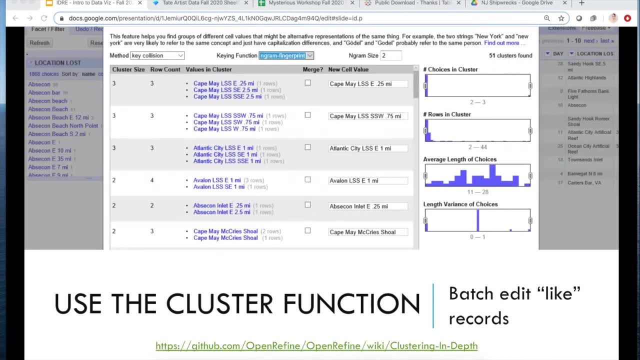 You can switch from name to count to find the biggest and smallest groups And you can batch, edit like records. So if you find things that are similar, OpenRefine groups, these things together for you so that you can assess them And if you would like to merge those things. 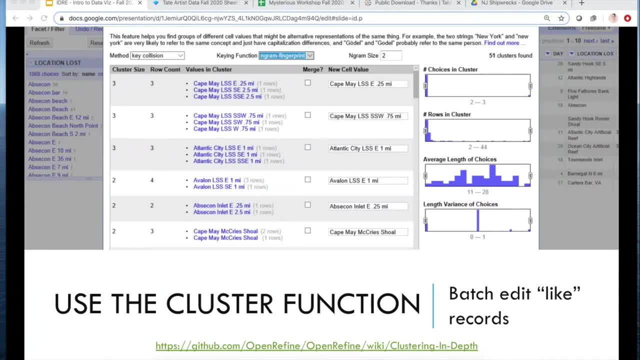 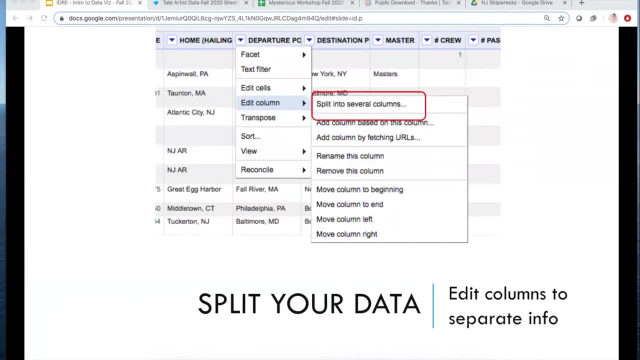 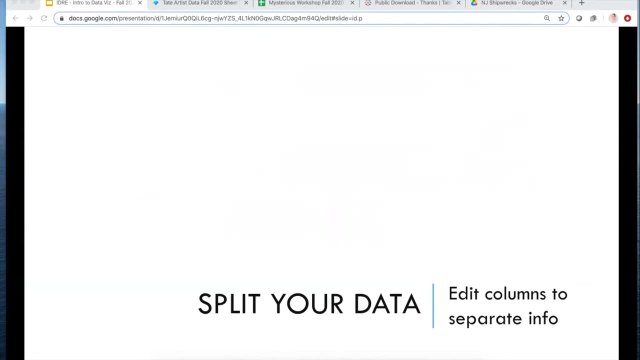 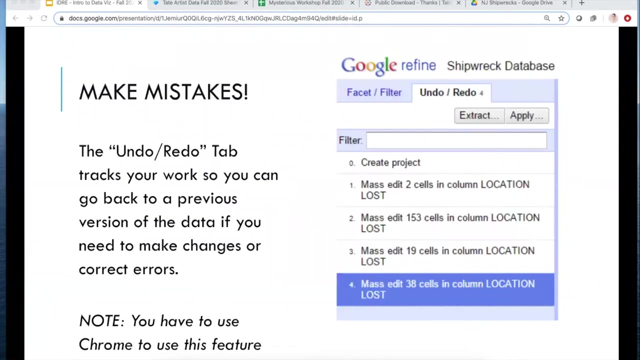 so that all your terms are the same. you can do that really quickly. You can also, like you can do in Excel or Google Sheets, you can split columns into separate info And you can use custom separators to do that. And, like Excel and Google Sheets, you can make mistakes. 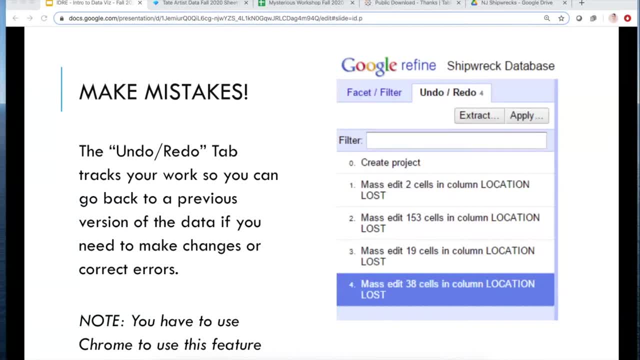 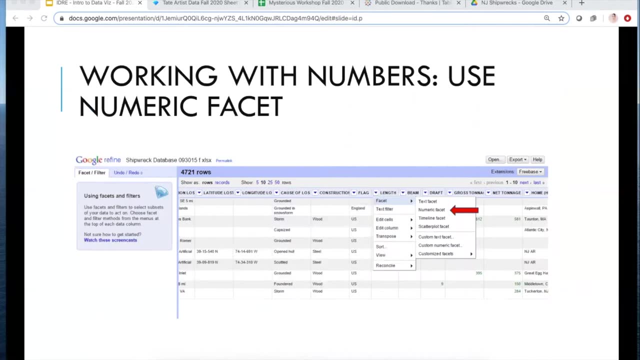 There is an undo redo function, but I believe this is still the case that you have to be in Chrome to use this feature, So you want to keep an eye out for that, And when you're working with numbers, you'll use the numeric facet. 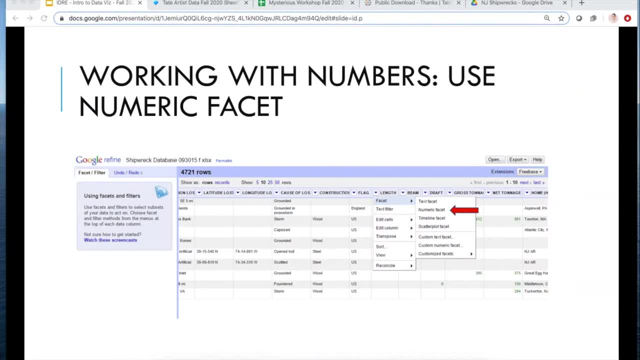 We'll talk about this a little bit more when we get into Tableau, But most visualization programs are going to require you to tell them what data type you're using, And so if you do this with OpenRefine, it saves you a step later on. 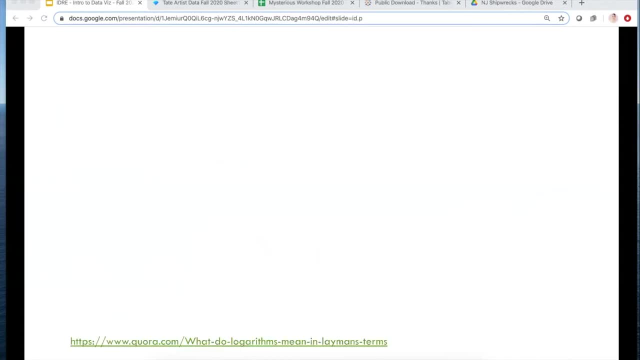 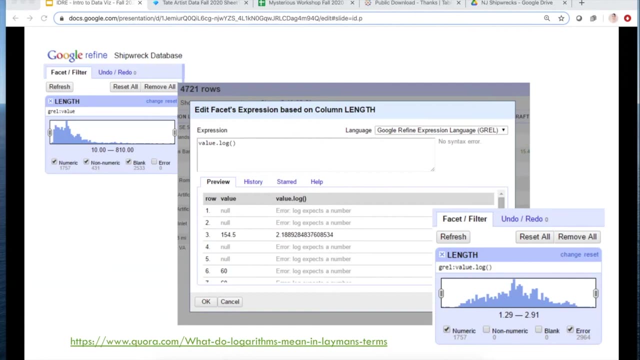 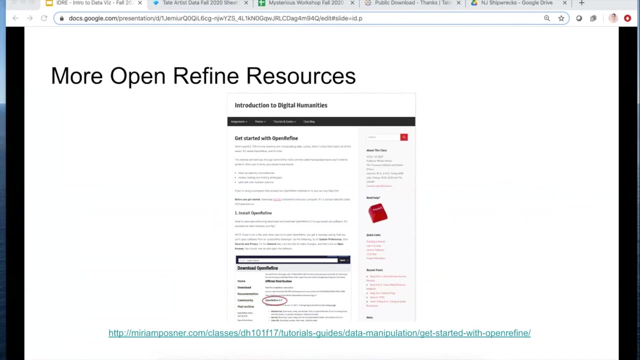 when you move your data into a visualization tool And then getting into the more advanced sort of things, you can use expressions to focus on specific areas of your data. And again, like I said, this is just a sort of drive-by of the functionality of OpenRefine. 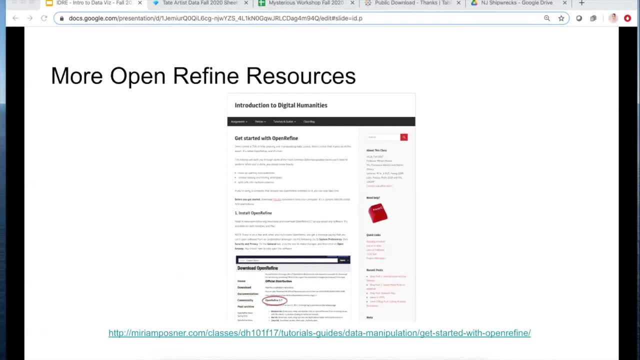 We'll actually get to do something in a minute with it, But the point being is that there's a lot of resources out there. These are some that I've helped put together with Miriam Posner, who's in the Information Studies Department and also teaches in the Digital Humanities Program. 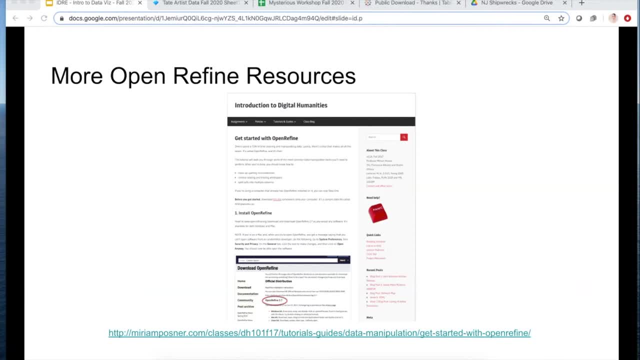 Her resources are phenomenal, So I highly recommend, if you want step-by-step on how to do any of the things that I just showcased in terms of functionality, these resources will show you. These resources will show you how to do that, And I'm happy to meet with anyone also outside. 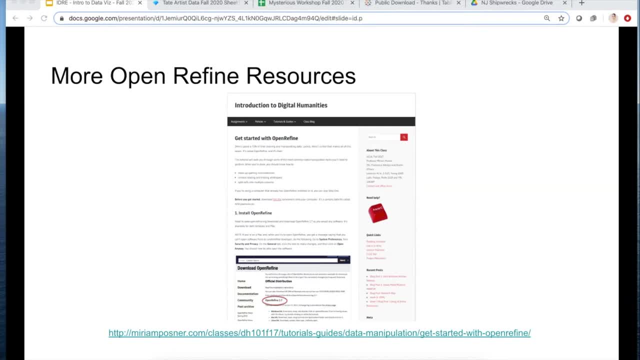 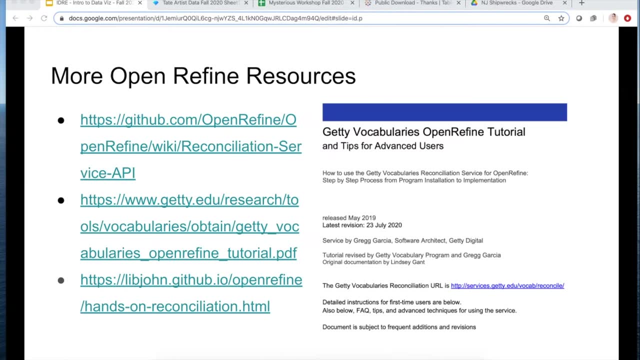 if you're interested in learning how to do these things. So for what we're about to do, I'm pulling from a Getty Vocabulary's OpenRefine tutorial, and it also has tips for advanced users, So I'm giving you that full link to that documentation. 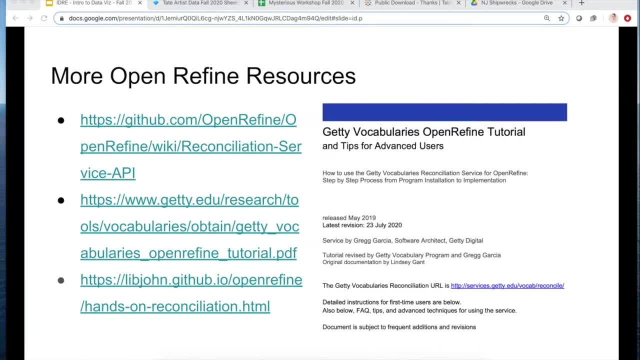 in case you want to check it out yourself- And I'm also providing you with a couple other links here- And what I'm about to show you is based on, like I said, an OpenRefine tutorial by the Getty, which will allow you to reconcile your data. 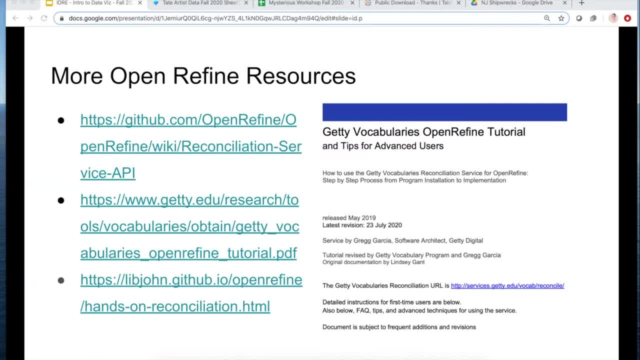 with their linked open data to help you standardize your data much more quickly. A reconciliation service is a web service that, given some text, which is a name or a label for something, and, optionally, some additional details as well, returns a ranked list of potential entities. 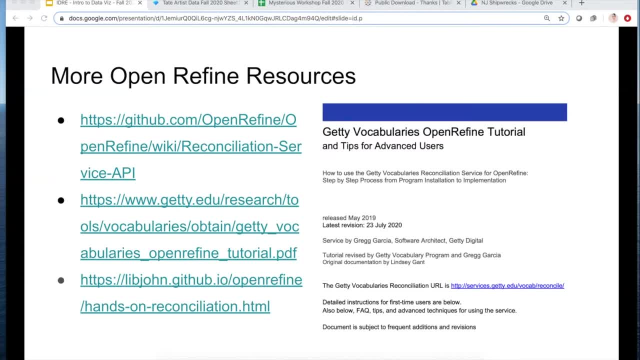 matching the criteria, So the candidate text does not have to match each entity's official name perfectly. and that's the whole point of reconciliation. to get from ambiguous text name to a precise identifier entity, For instance, given the text Apple, a reconciliation service probably should return. 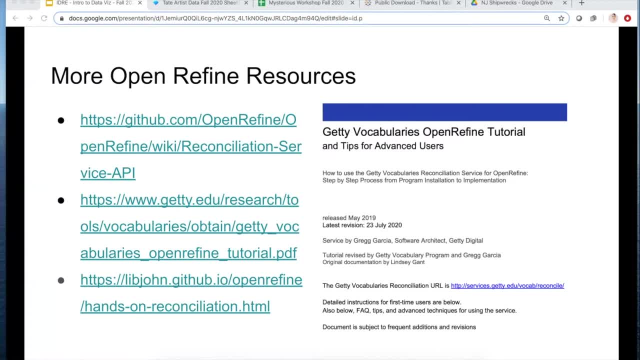 the fruit, Apple, the Apple Incorporated Company, and New York City right, which is also known as the Big Apple. Using the API, you can do this for a variety of data services, For example. the last link in this list is for how to reconcile data with Wikidata. 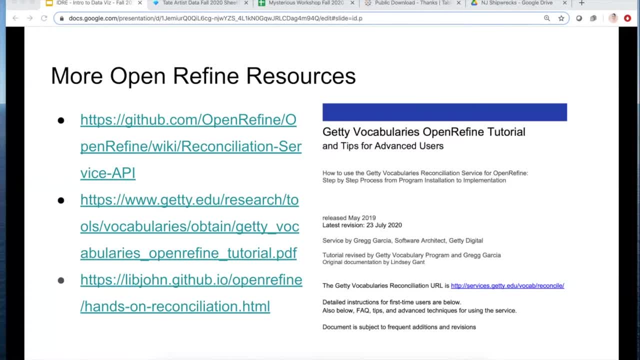 and the IAF services, which is for libraries. So there's going to be a lot of different types of authority data files that you can use as part of this, but I'm going to show you how to do it for the Getty vocabularies. 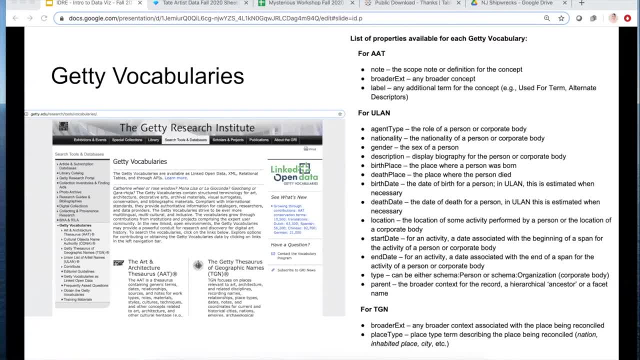 And the Getty vocabularies include the Art and Architecture Thesaurus, or the AAT, the Getty Thesaurus for Geographic Names, the TGN, the Cultural Objects Name Authority, or CUNA, the Union List of Artist Names. 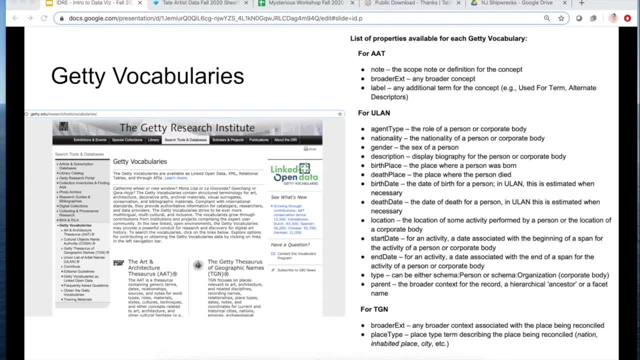 which is what we'll be using today with our TATE dataset and the Getty Iconography Authority or IA, And the three most popular are available in OpenRefine, where you can reconcile your data based on these elements here on the right. 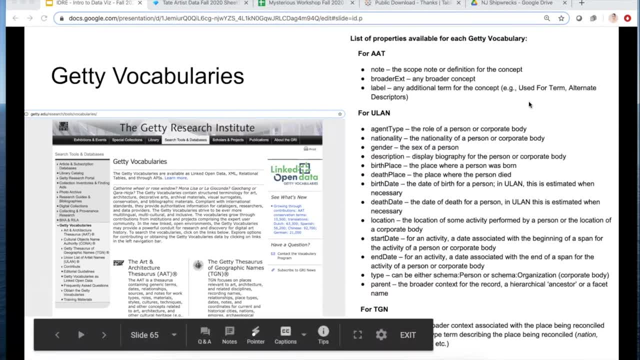 So if you see this list on the right-hand side over here, these are the types of things that you can, the characteristics you can reconcile in OpenRefine. So we're going to do this for our list of TATE artists to make sure we have their most. 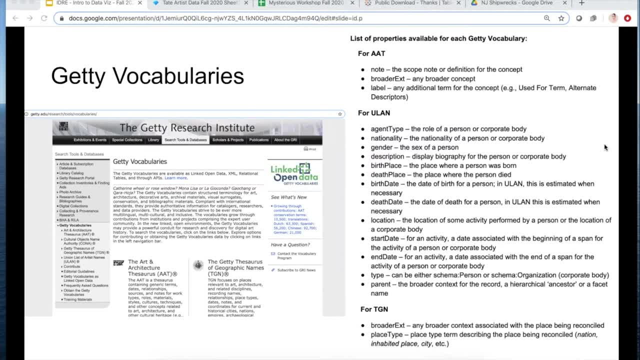 make sure that we have their ULAN authority file attached to our data. But you could also do this with TGN- not TNG, that's Star Trek, but that would be cool- and get their location data right. So, if you use the Thesaurus for Geographic Names, 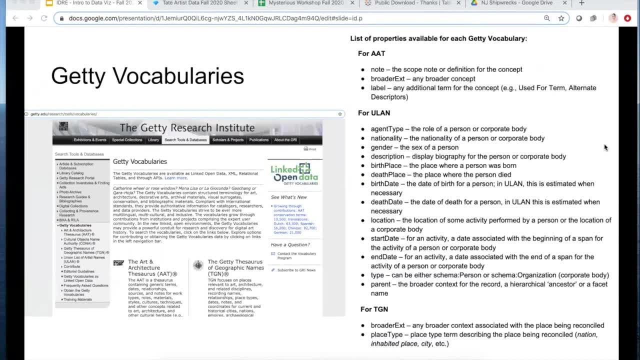 you could get the lat-long coordinates for places, which is actually a really great thing to know how to do, because many GIS programs- this is part of their paid services- is to provide you with lat-longs and you can get them for free. 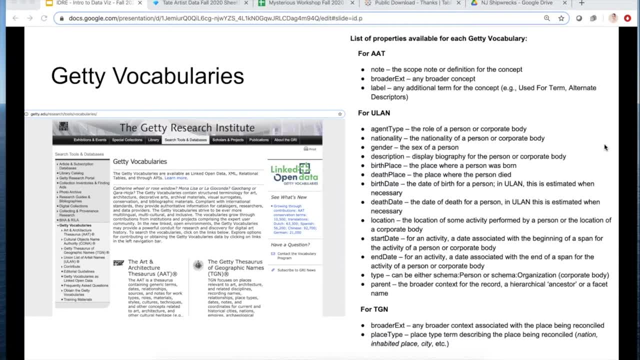 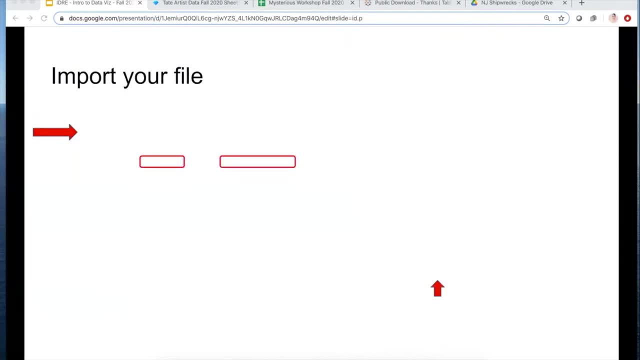 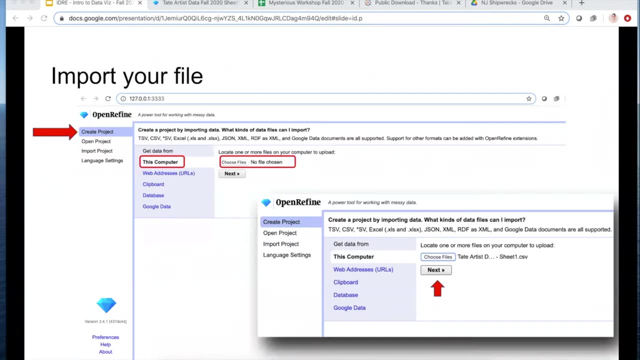 through the Thesaurus of Geographic Names. So that's one thing to keep in mind. So if you all have your OpenRefine open, you're going to want to go to Create and under this computer, you're going to choose a file. 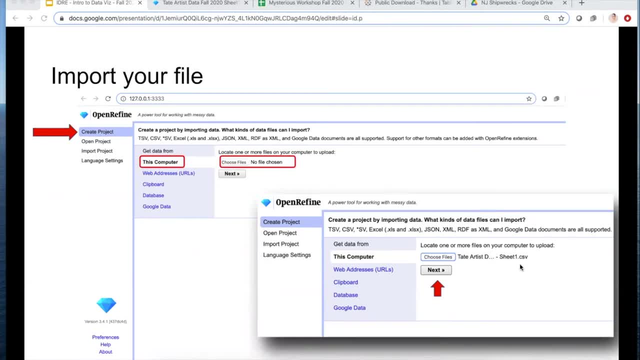 and you're going to choose that TATE artist data sheet that you downloaded and you're going to import that spreadsheet so that we can edit it. Alternatively, you may choose to open a project or import a project to continue work on and in project. 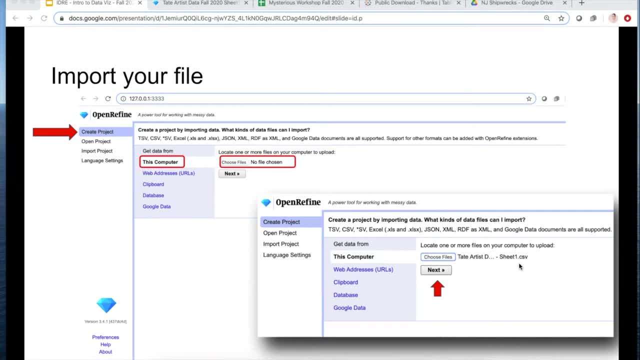 and obviously you can see here from the choices at the top. you have a lot of different data types that you can use in OpenRefine, or different file types, I should say, And once your file is uploaded, click Next. Let's give everyone a second to do that. 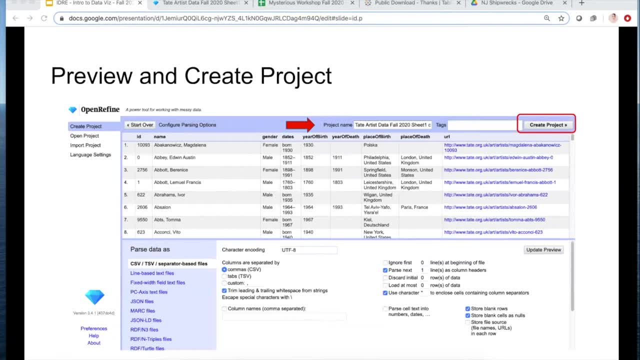 So once the file is uploaded, you will see a preview window that looks like this: Does anybody not see that preview window? Please let me know in the chat or unmute yourself and let me know. Everyone's following along. Okay, great. 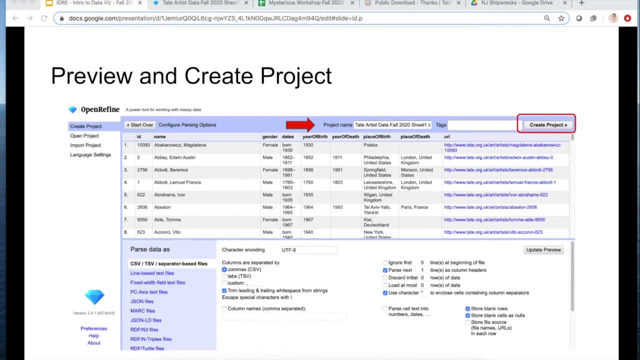 So give your project a name in the Project Name field or use the default name. So that's right here. So that's right here. Select Create Project at the upper right of the page. You can keep all these settings. These are all fine. 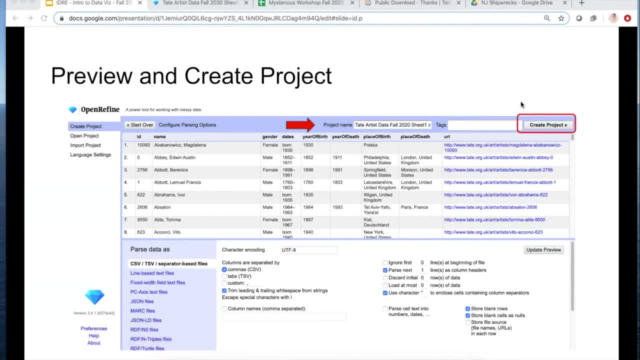 This is how the data is getting parsed. That should all be automatic and you can just click Create Project. You'll be taken to another page from which you can edit the cells and columns on the spreadsheet and use the reconciliation service. So we'll do that in just a second. 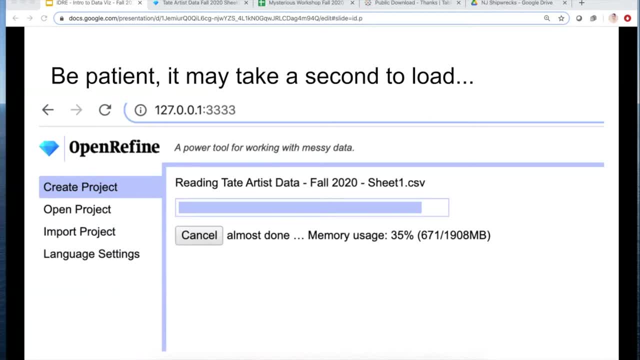 So this may take a minute to do, Depending on how large your data set is. it may take a few seconds, if not a little longer. Is anybody having trouble getting their data into OpenRefine, or is everyone okay with that? No, No issues. 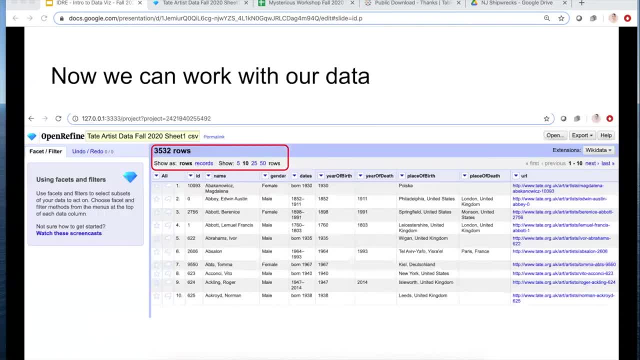 Okay. So when it's done loading, you should see something like this: At the top. you will see the number of rows, which is 3,532, in your sheet, and you can adjust how many are displayed. But OpenRefine doesn't show you. 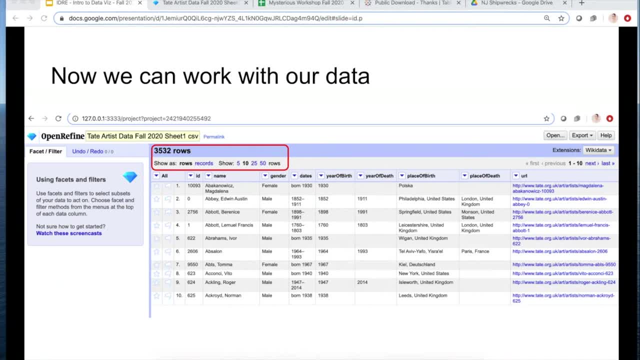 all of your rows at once, like in Excel or Google Sheets, and this is because you're really meant to be using it to clean your data, So you're going to be performing things in batch more than you are on individual rows. You can work with individual rows. 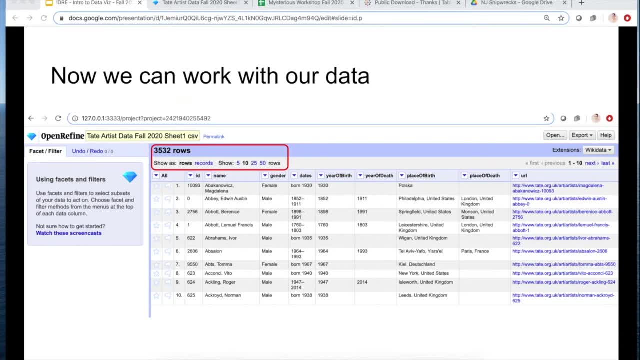 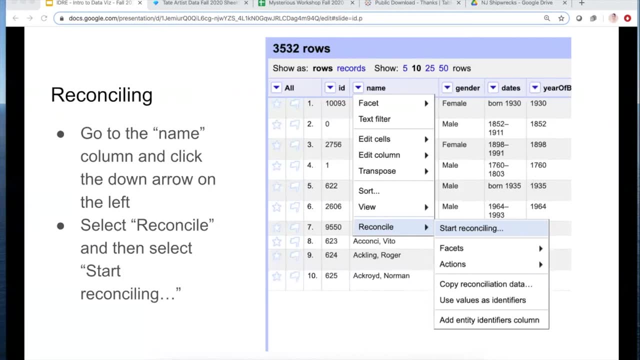 but it's really designed for doing sort of batch transformations, big transformations within your data. So to reconcile, you're going to go to the Name column and click the down arrow on the left. You're going to select Reconcile and then select Start Reconciling. 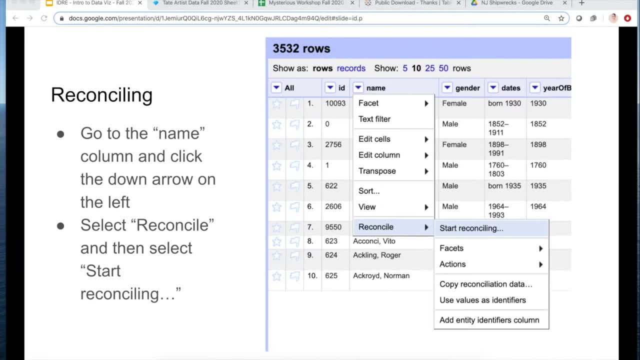 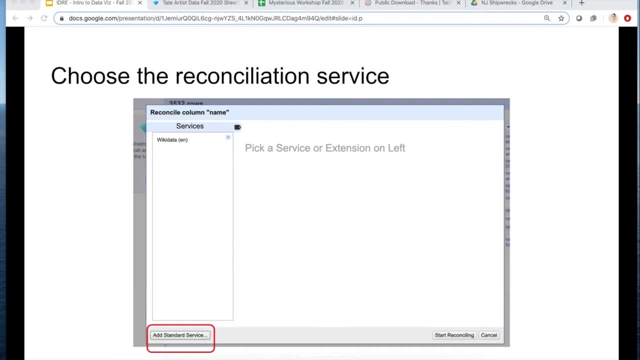 Now, the reason why I've canned all of this is because reconciling can take a really long time, And in fact, well, I'll walk you through this process here. but once we hit Start Reconciling, it will take about an hour. 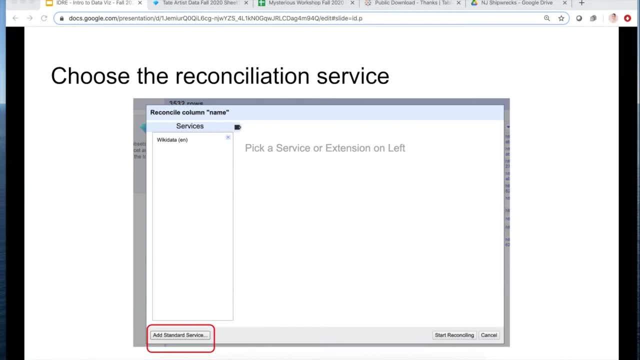 to an hour and a half for this data set. So if you have even bigger data sets, you're going to want to factor that in. You're going to want to be able to like go have a cup of coffee with somebody or a remote cup of coffee via Zoom. 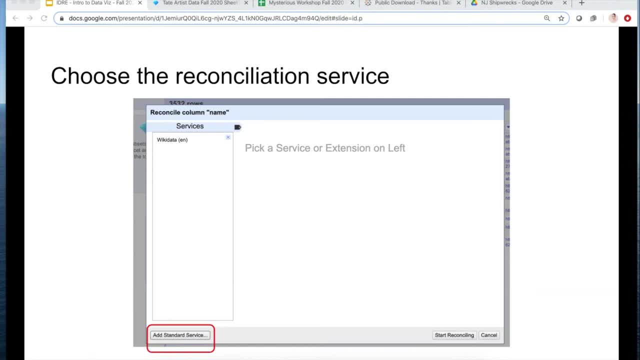 since we aren't getting together all that often anymore. But you'll want to take a break and come back And that'll keep going in your browser and you'll see it ticking away in your browser so you will be able to track the progress. 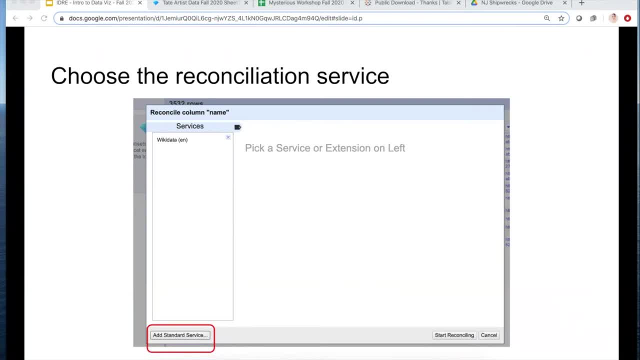 and know that it's still working, But it does take a little while. So, from the page Listing Services, select the Add Standard Service at the bottom left of the page and this is how we're going to. I don't know if you can. 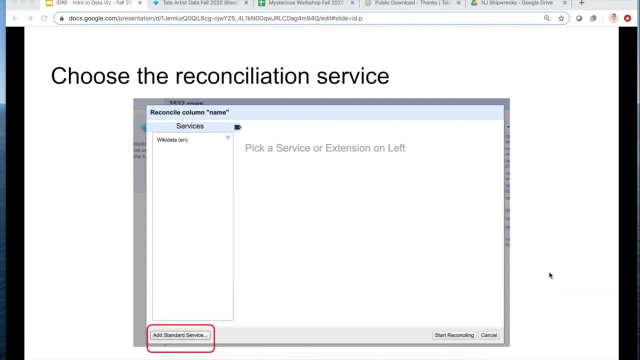 My bar came up in front of my slide, But you can, In that bottom left corner you'll see Add Standard Service And this is how we're going to add the Getty vocabularies. So to connect the Getty vocabularies, 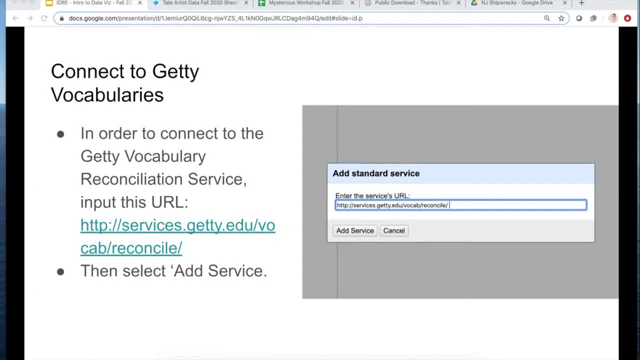 you're going to input this URL, So http//servicesgettyedu. slash vocab, slash reconcile, And once you've done that, you're going to select Add Service, And it's as easy as that. The Getty Vocabulary Service will now appear in your service list. 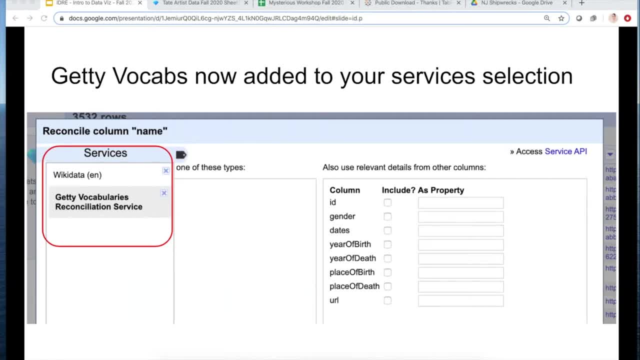 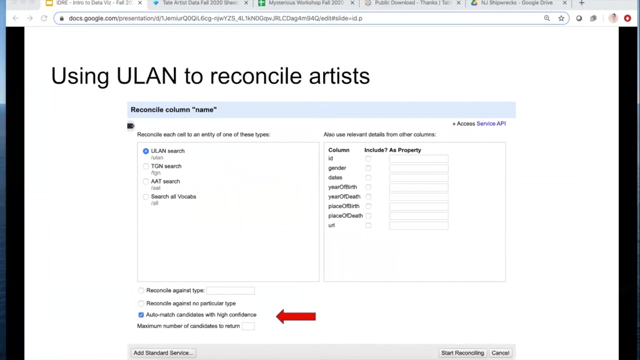 And every time hereafter that you use this same version of OpenRefine on this computer, the Getty Vocabulary Service will be on your list. Is everybody able to do that, Or anybody not able to do that? Still with me. Okay, So in the service list now. 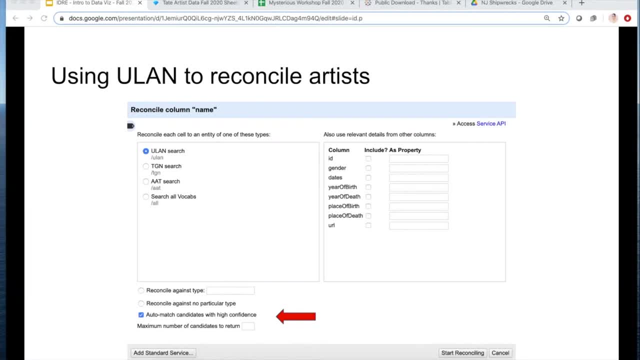 click the Getty Vocabulary Reconciliation Service and select one of the vocabularies. In this case, we're going to use ULAN And we're going to use auto-matching if there's a good correspondence between your source data and the set. 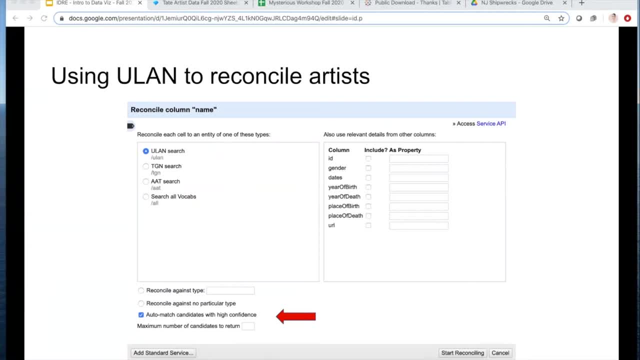 in the target Getty Vocabulary. You may wish to use auto-match candidates with high confidence, which is in the lower left corner. You may want to turn that on. In this case we do, because ULAN does match up really well with the state data set. 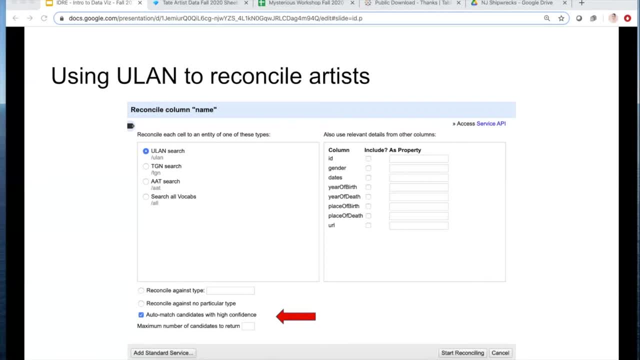 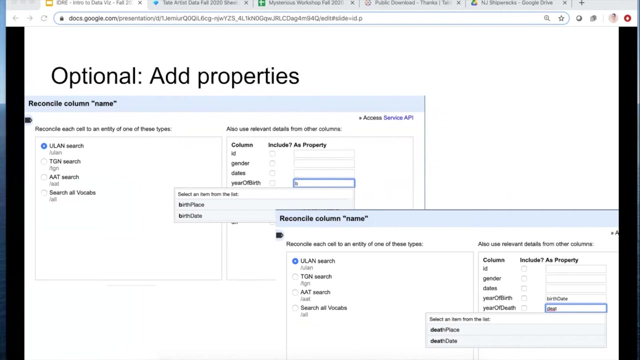 So we can leave that on. But auto-match tends to work better for ULAN than the the Art and Architecture Thesaurus or the Thesaurus for Geographic Names due to the typical variables. so properties in the source detail In most cases. 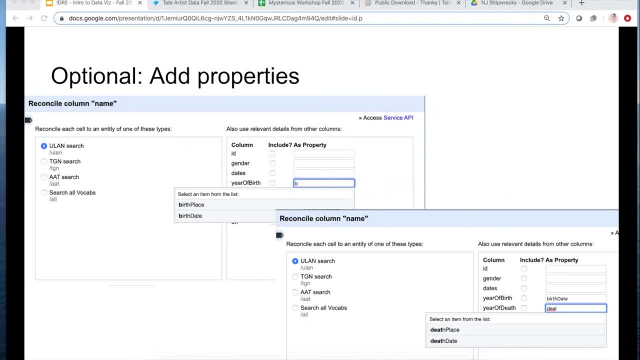 you will have better results in matching if, In addition to matching on the name or term, you can compare properties in the source data to properties in the Getty Vocabularies, If your data set contains columns that can help identify or qualify the entities. 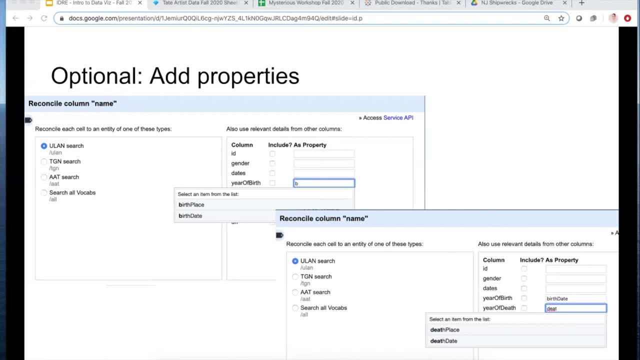 during the reconciliation, OpenRefine, Reconciliation Results will take these columns into account in the matching scores. So, for example, if for ULAN we have the birth and death date, we can add because we are going to have similar columns or data types in our data sheet. 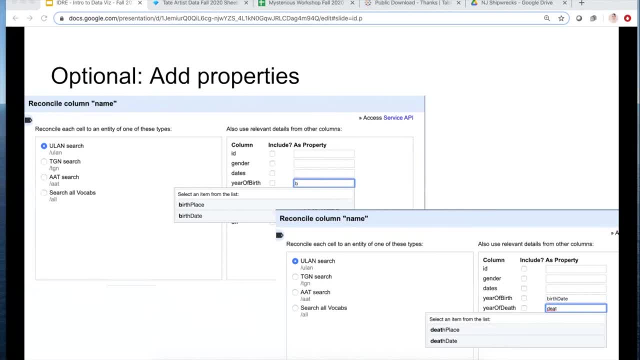 right, We can input the property selections under the column as property. So you can see, here for ULAN we can actually type in. we have in our own data set year of birth and we know from that property list that. I showed you several slides back. 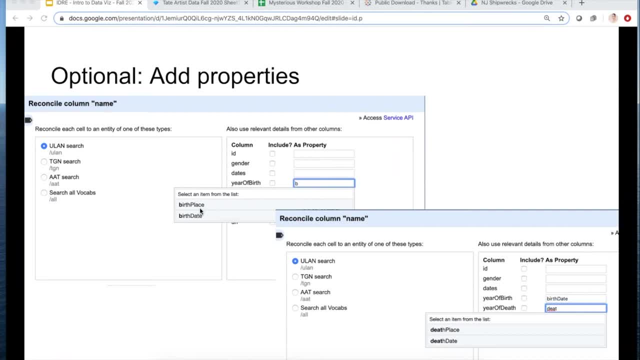 that birthplace is one thing that ULAN has, So you'll want to. you can match those things and that'll that'll be. that'll help you make those matches more confidently. So if you just start typing a value, you can autofill by choosing. 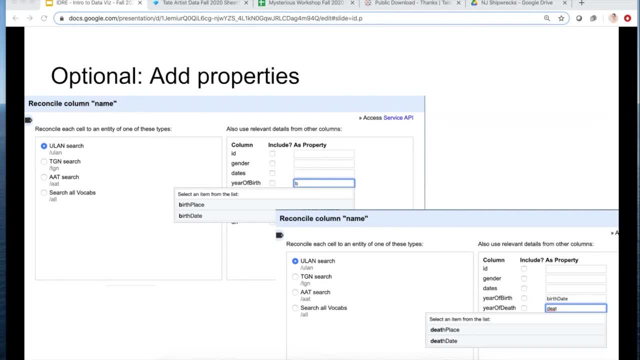 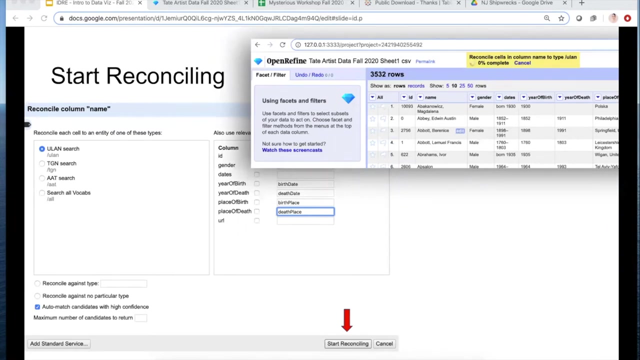 sections provided for ULAN. Make sure you also select the include box so it knows to use those fields. So this include box here. I want to make sure that you do that as well. And when you finish adding properties, you'll click start reconciling and you'll be taken. 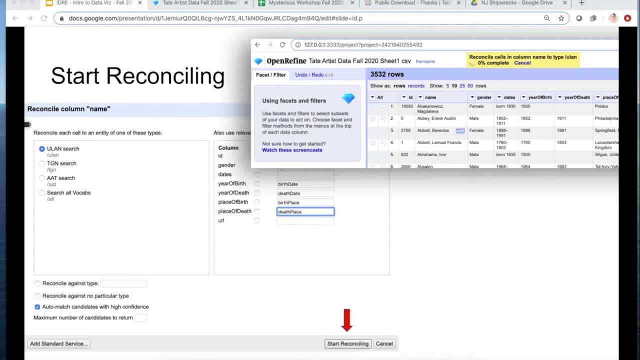 back to the spreadsheet view where progress is tracked And, like I said, this will take some time. for this sheet It took about an hour hour and a half, So I'm going to show you the next part, so you know what to expect. 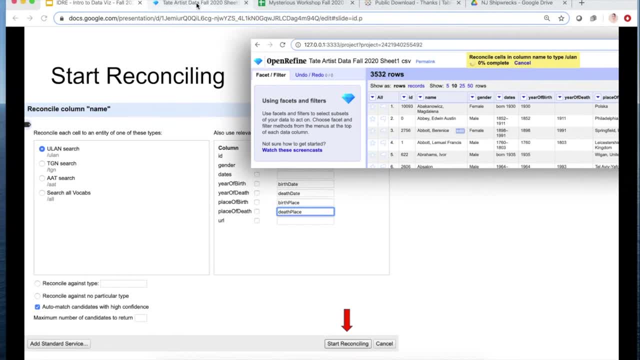 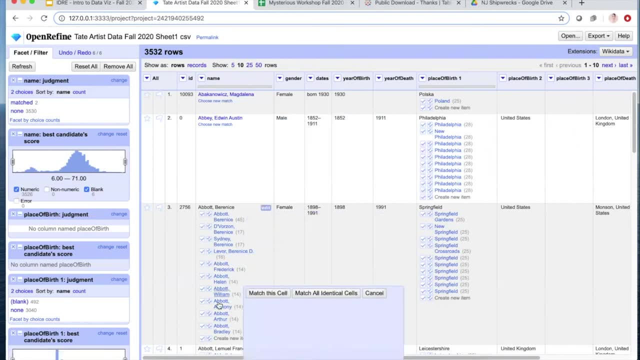 And you can see it over here. I actually have my open refine data sheet open here. So this is an example of what happens when I've used it for the artist names. So, for example, I've gotten a match here for Bernice Abbott. 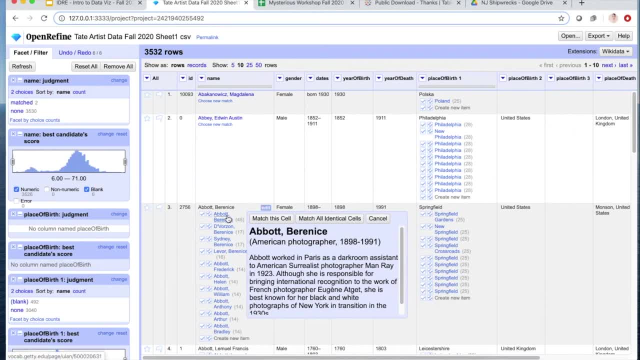 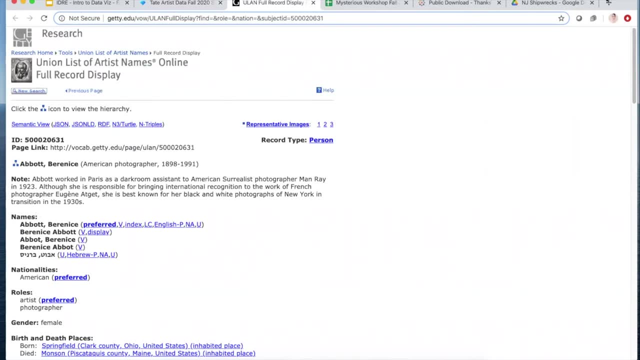 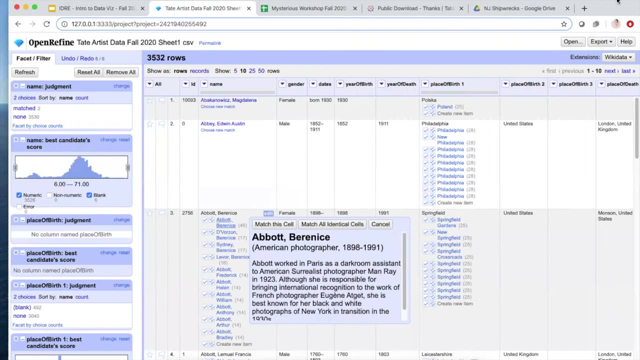 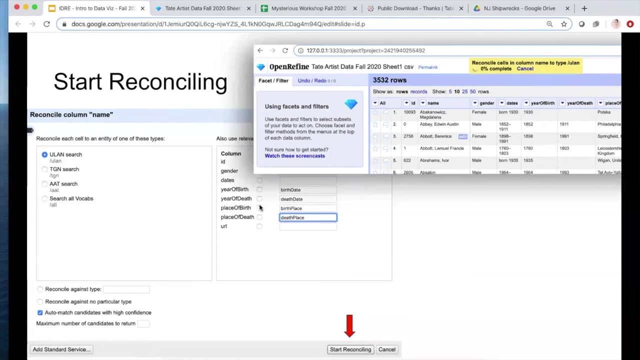 and I can actually click on this and it'll take me to the Getty record. so I can check the Getty record. if I need more information, I'll bring this down for a second Zoom bar got in the way, So when you finish adding properties. 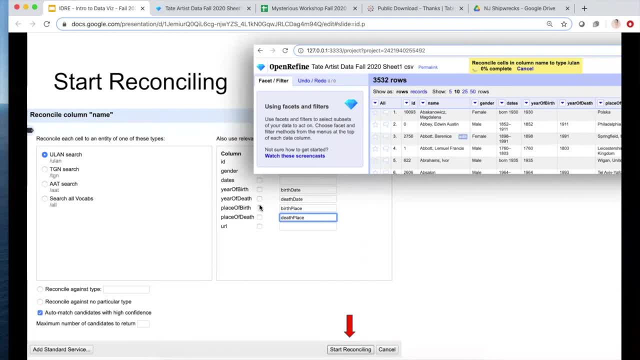 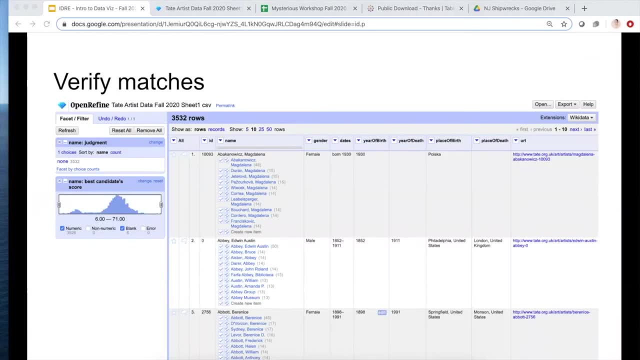 I'm going to. oh yes, So let me move to the next slide. Did we want to check include for all of them or just the ones that we? Yes, great question. Just the ones that you're able to match within your columns. So that would be in this case. 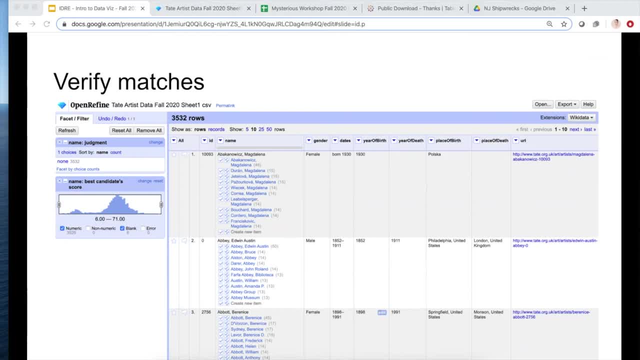 birth, birth date or birth year and death year. You can also do- which I'll show in a minute in these slides- place of death and place of birth, if you have that information, which we do as well. So after the reconciliation process ends, you'll want to verify these matches And you may wish to 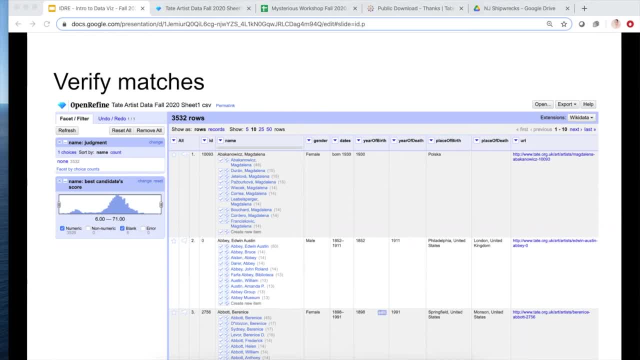 check these matches by hand if possible, particularly if the ranking is 40 or lower. However, the possible matches, in this example to Ulin, appear in the column in the blue under the source value being matched, which is the name of the artist that we had originally. 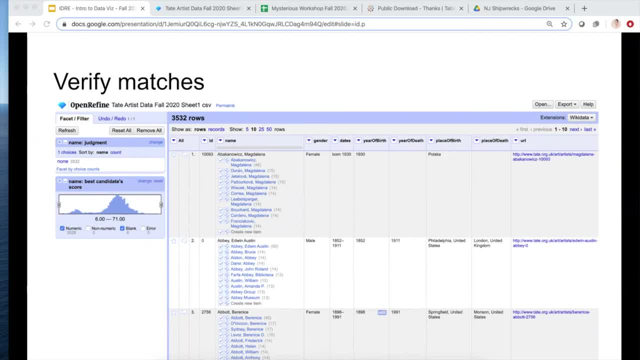 and sorted by ranking in parentheses. So these things right here. this will let you know sort of the percentage, how likely of a match it is. So obviously this first one is the name of the artist that we had originally and sorted by ranking in parentheses. 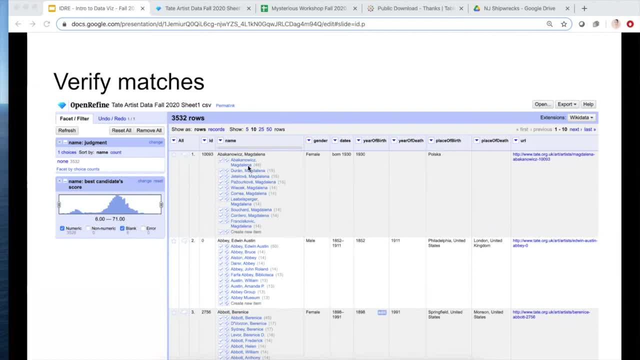 A pretty good match. It's above 40.. So we know that that's the likely candidate. Same here: All these lower numbers are indicating that it's not as likely of a match And this one's a 50%, So we know that's likely going to be a solid match compared to the information that 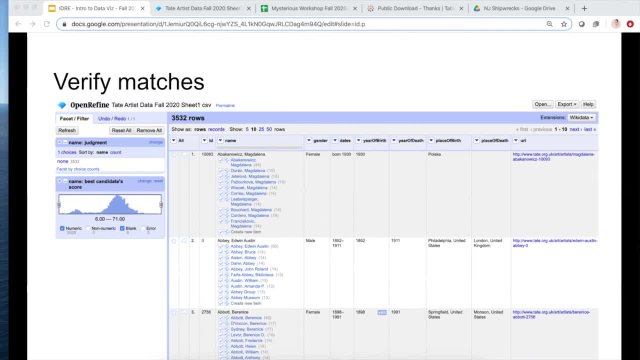 we have in the other columns as well. But just a note on the scoring the Vocabularies Reconciliation Service for OpenRefined does not use normally. It's a service that is used to analyze scaling for matching results. The search gives relative. 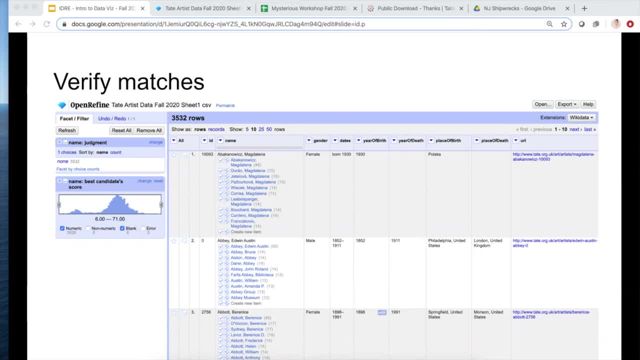 results based on how many data points match Vocabulary's data. So text matching, broader context, birth and death dates, things like that. So the things that we've included, In general, the better matches have higher scores and it's up to the user to determine what. 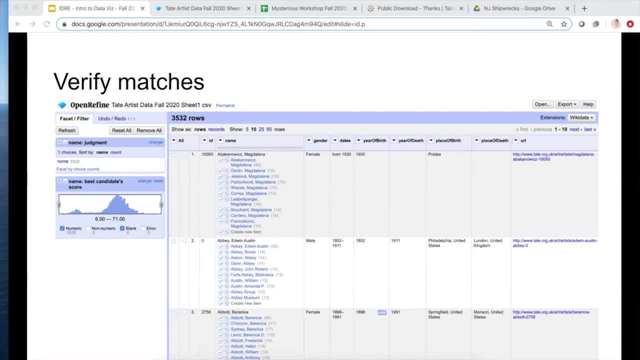 the acceptable threshold is for an actual match. In the same manner, the service intentionally does not do auto matching because they don't want to assume any kind of expertise about the source data and create bad matches. So, for example, if you're working with a special 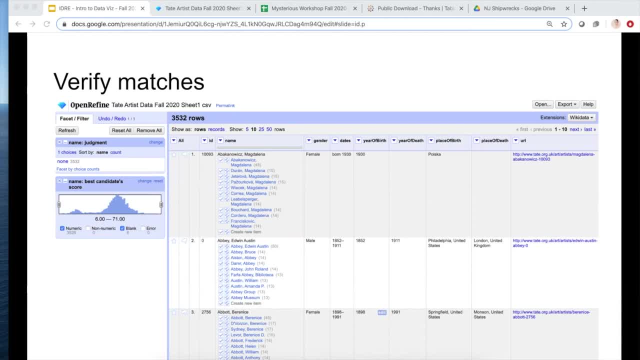 collections, a new set of data that you formed, based on special collections material. maybe you have a date that precedes the date that they have in ULIN, And that's actually an important research find, right, That's not something that you, that you're going to want. 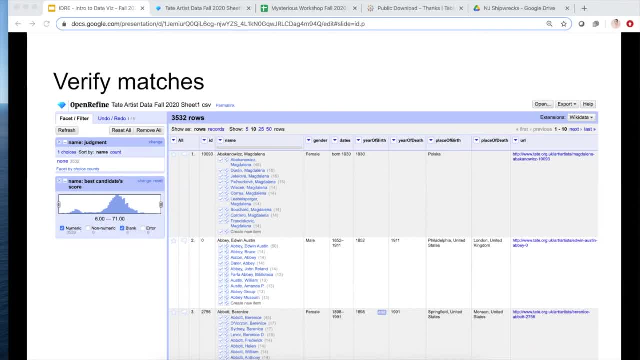 to erase And overwrite. you're going to want to see and acknowledge that. So that's why, when I talk about data cleaning being a part of your process and this being an iterative process for data visualization, these are the exactly the types of things that you're going to run. 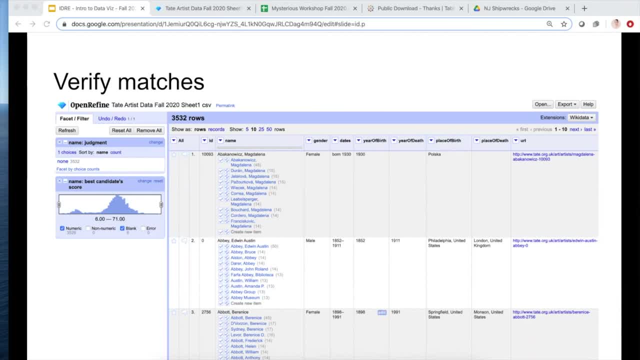 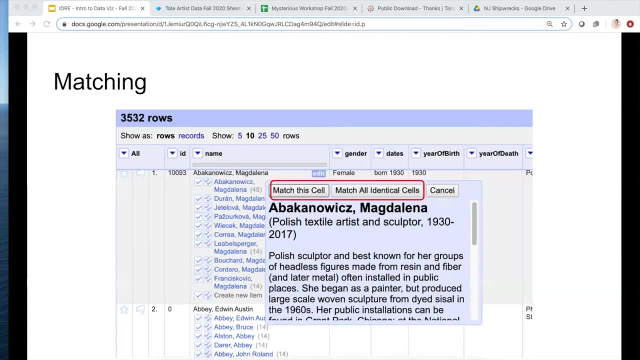 into that are going to help your research process and help your discoveries happen. You can see information from the ULIN match by hovering over here. You can see information from the ULIN match by hovering over the blue name. Hovering inversions 3.2 and higher works. 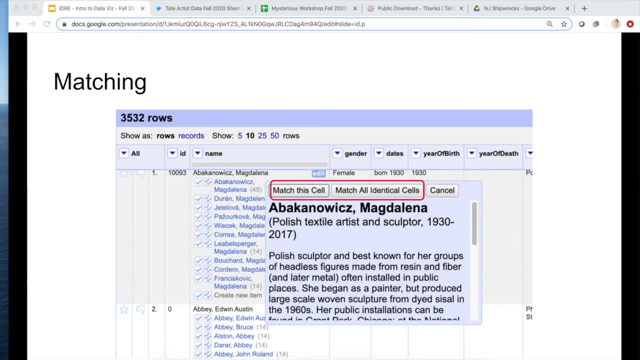 If you have 3.1, you must click the ULIN record to actually see that information. But I think all of us should be on 3.2 or higher at this point. When a window will display the ULIN data, then you can click from there. 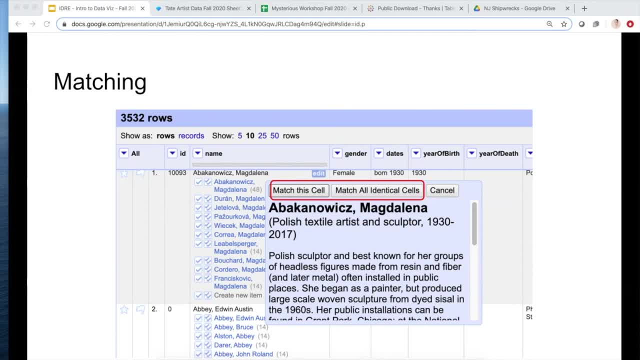 Okay, Okay. So basically you can see your data and data groups that are in the ULIN match And you can choose if you want to make a match based on the birth and death dates that are there as well, And you can match this cell, So this particular item, but if you have multiple, 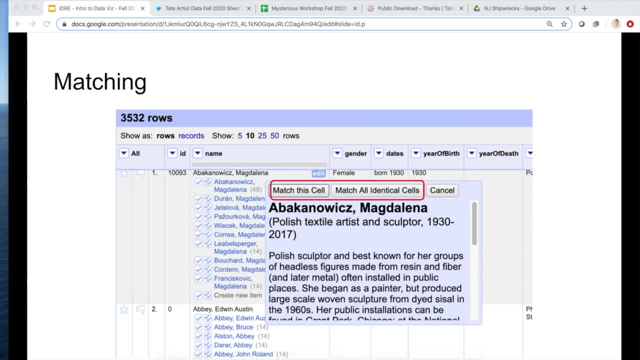 values in this column that should be reconciled to the same vocabulary record. you could click match all identical cells. So those are things like the birth and death year, right? So if you wanted to change, transform it across that record, you could. based on the information that's coming from U-land. 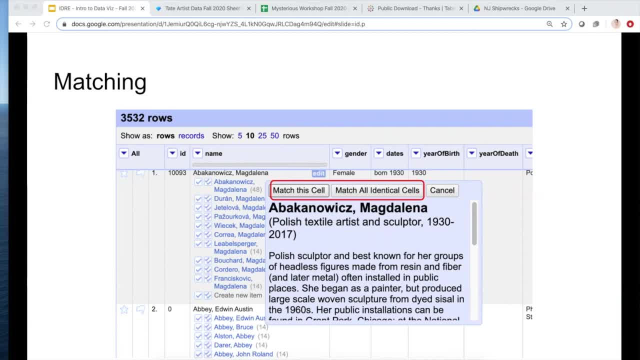 I'd advise that you use this option with caution, given the high probability for homographs in the vocabulary data. but also, perhaps you've formed your own data, like I was just saying, and your sources provided an alternative set of dates, and you want to compare this to the authority file. 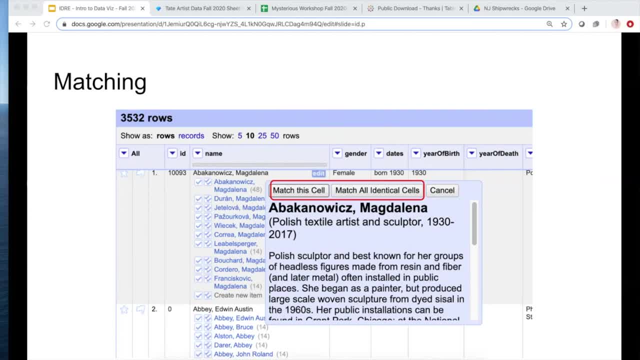 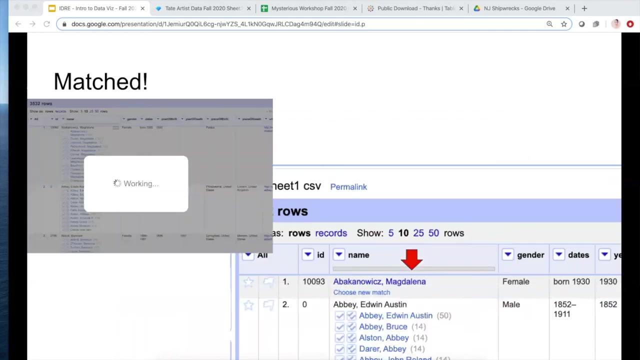 as part of your research. So if you need more information before deciding, you can, like I said, always left-click on the blue name and go to the full web record to see the Getty vocabulary entry. And so this is. it may take a second once you click match, but once you do you'll see it's. 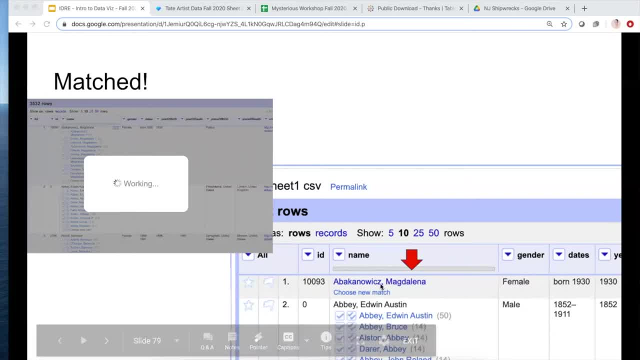 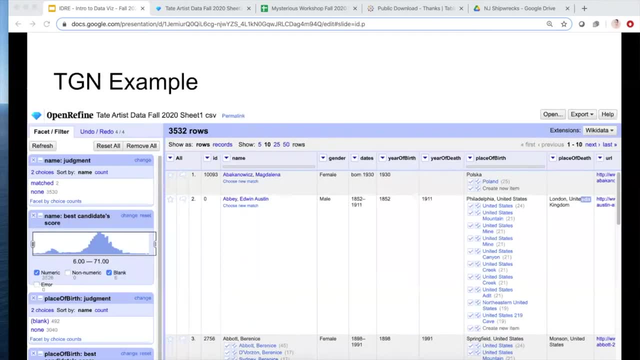 given you a, this is how a match will display, And then I've shown you how to do an example for U-land, And the reconciliation service also works in the same way for AAT and TGN matching. I just want to point out, though, that in reconciling, using 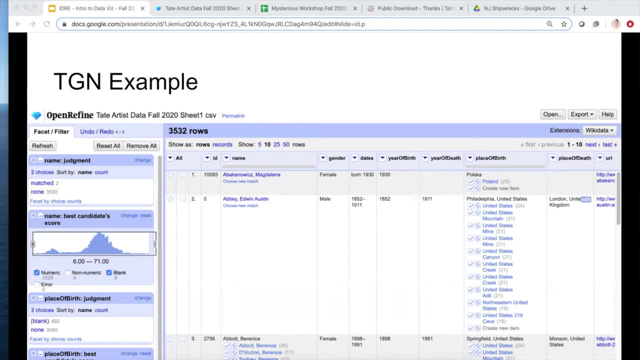 the thesaurus for geographic names. several you know the thesaurus for geographic names. the full homographs have nearly equal ranking, So you can left-click to go to the full records online in order to see if the geographic coordinates and other information can help you assist in making that. 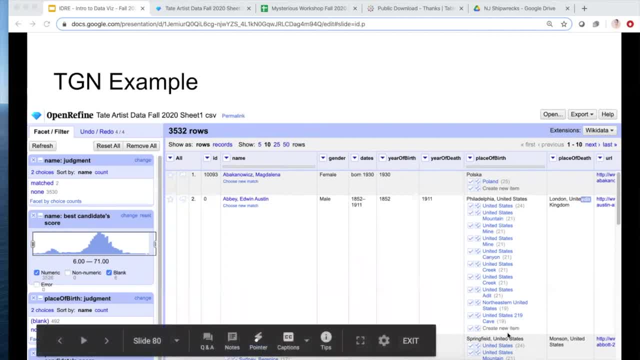 decision. So, because these things are all in the same column, you can see, here most of these things are coming out. It's not quite sure which one to choose, And this is probably because we have city and country, and and this is probably because we have city and country and we're looking at communities. So it's a. it's a little, it's a small piece, but it's an. it's a pretty small piece, but it's an important piece. we want to, you know, to make sure that they're comfortable with where they are and what they're doing on. 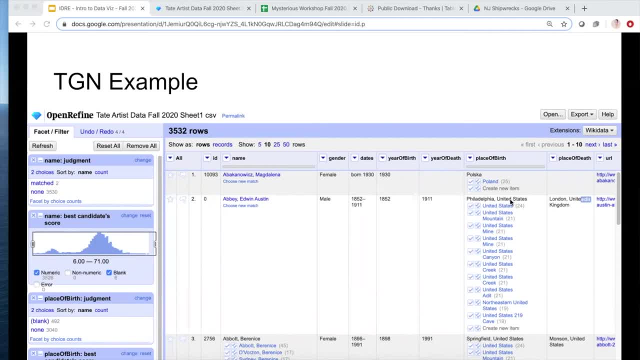 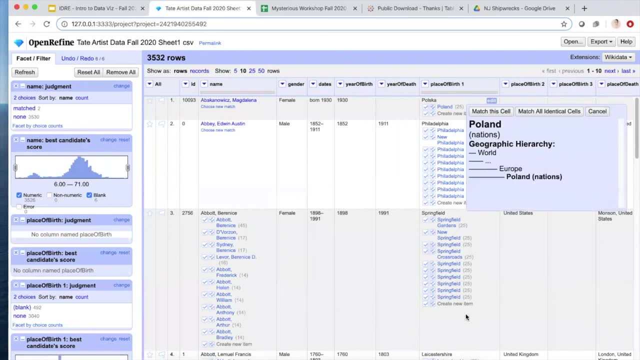 have city and country in the same field. So I'm just going to quickly go over here and show you on the fly how to do this, if you wanted to separate. So I had already separated these things here, but let's move to place of death and I can show you again how to do that. 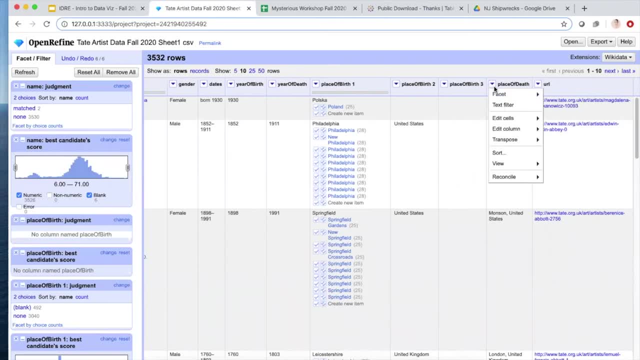 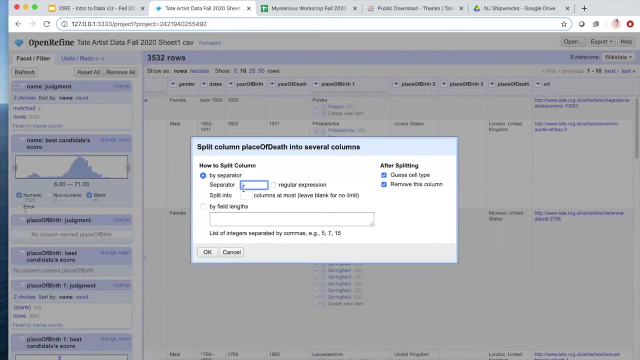 So if you go to place of death, you can click to edit column and split into several columns, and we want to use a comma. right, That's how they're separating the difference between country and, in most cases, cities. So we'll say okay and then OpenRefine will do its thing. 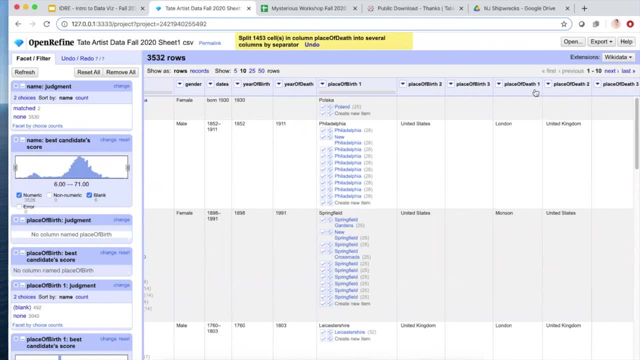 And now we We have additional columns, So we have place of death one, place of death two and we can run the reconciliation services on these things independently to get slightly more accurate connections with the source of geographic names. Does anybody have any questions on that? 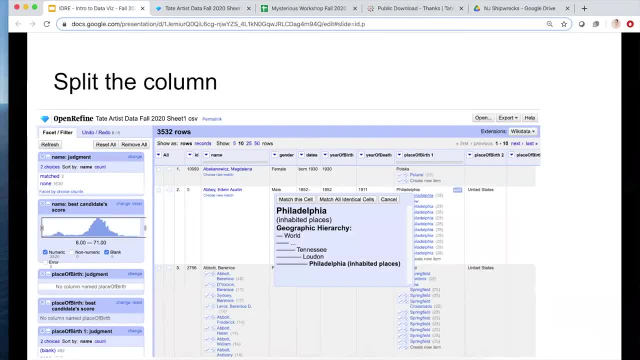 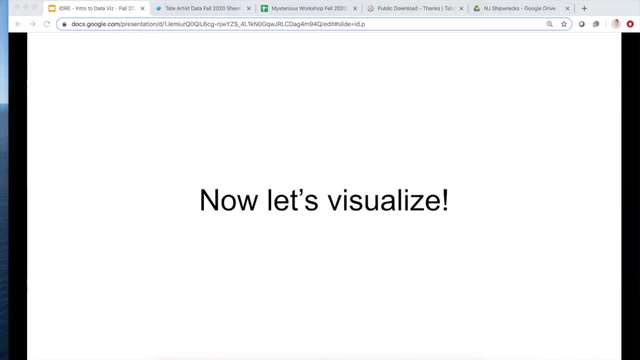 Okay, So we'll leave it there and move on to visualizing our data, but I wanted you to know what tools are out there to help you get a handle on your data, because it needs to be organized and cleaned before you can create strong visualizations. So definitely check out those other. 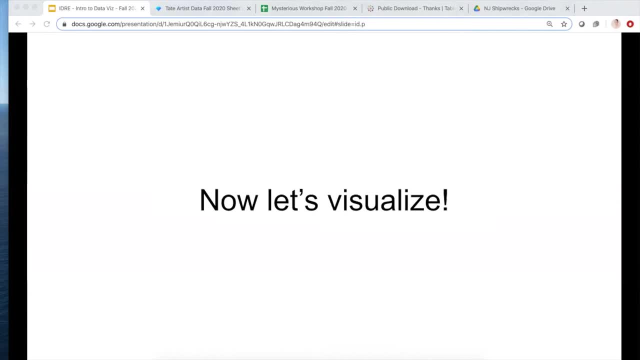 resources I included if you're looking to learn more- And I'm going to just pause for a second here because I saw a question come in in the chat, But we have to go through a couple of things. So is it true that every single record has a match in every single record? 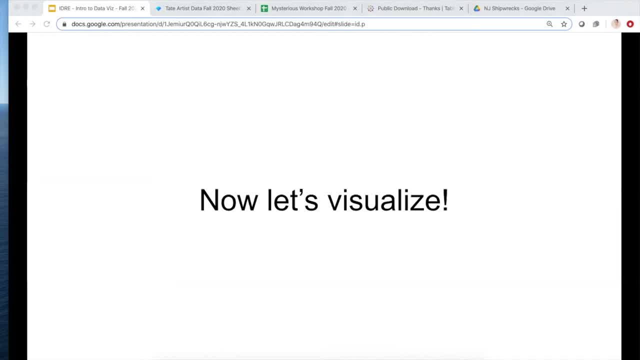 Yeah, And we do have a representation, a notification on every single record, in every single row. So they've created that information for us in the open and in those locations. but it needs to be clear that every single record that you're using there that you want to include is that through. every single row. So in the advanced documentation there are ways that you can do this transformation slightly more quickly, But the point is that they have made it more difficult and they haven't made it automatic, because they want you to look at every single record to verify that you're okay with that match. 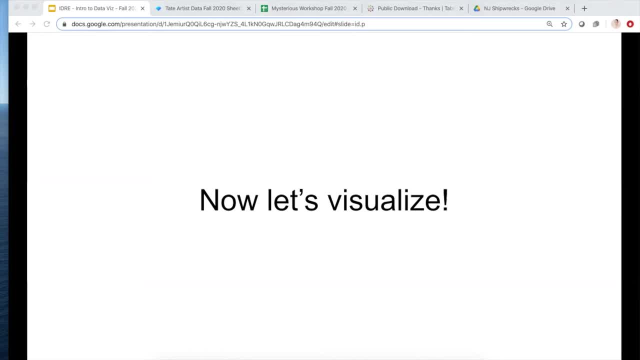 Yeah, I think this is a really good question And I think we have a question I'll give to Gertie about. So, if you have any question that you'd like to ask me, I would like to ask you a question with that match, But in theory, anything over 40 should be a good match for you, So you can set up. 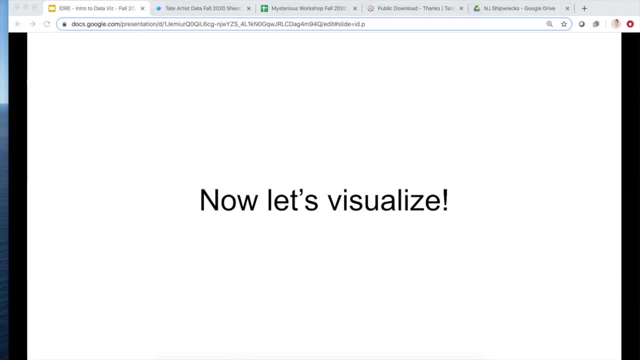 I believe, an automation way that will automatically accept anything above 40, if that's what you want. But check out that advanced documentation for exactly how to do that. Okay, so let's jump into visualizations, because I know we only have about. 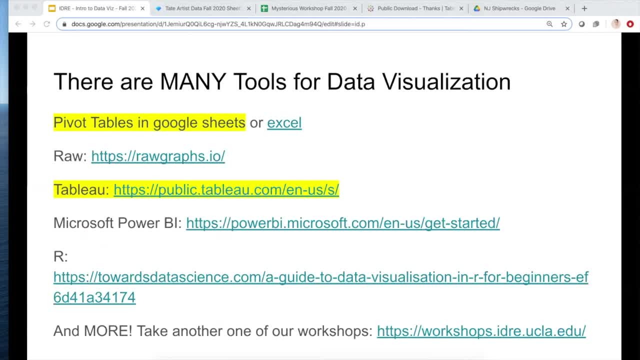 an hour left and I want to make sure we get through actually visualizing data. So pivot tables and Google Sheets are going to be the first thing that we work on And then we'll look at Tableau. But there are many tools for data visualization, So I'm going to go ahead and 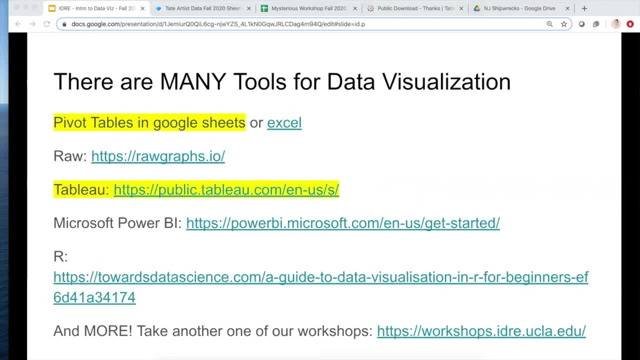 these are just a few that I'm noting here. Excel is great If you have Excel and you're already working in Excel. there are many ways to visualize with Excel, But there's also things like rawio. Microsoft Power BI has its own set of visualization tools- R, if you're in statistics. 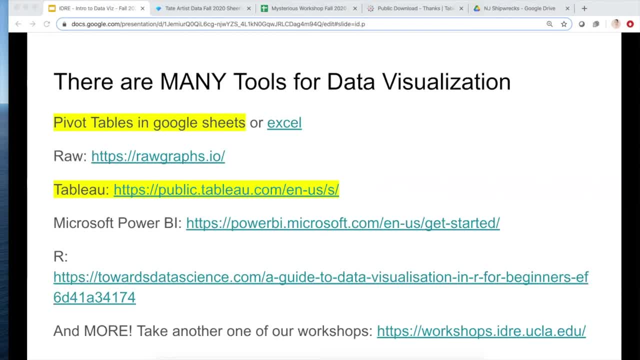 and R is becoming a really popular language, not just to work with data but also to visualize it, And I again highly recommend taking a look at the workshops that Idri offers. There are always new ones coming out on different visualization. tools. 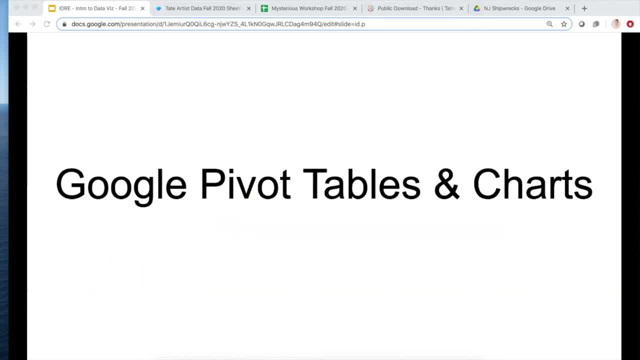 so definitely check those out. So we're going to quickly cover some basics of Google pivot tables and charts and demonstrate some easy ways to throw together useful data visualizations with lightweight tools. Think of this as your appetizer. like I said before, Getting into Tableau will be our main course. There's more of a learning curve with Tableau. 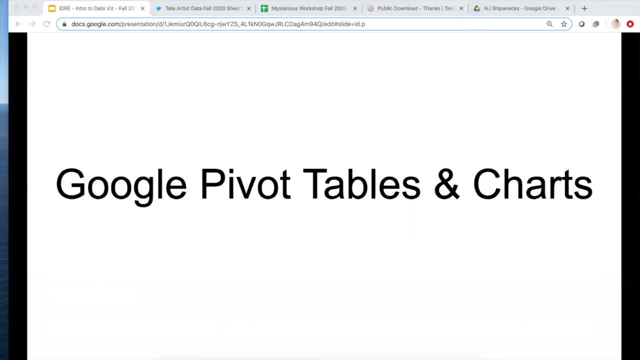 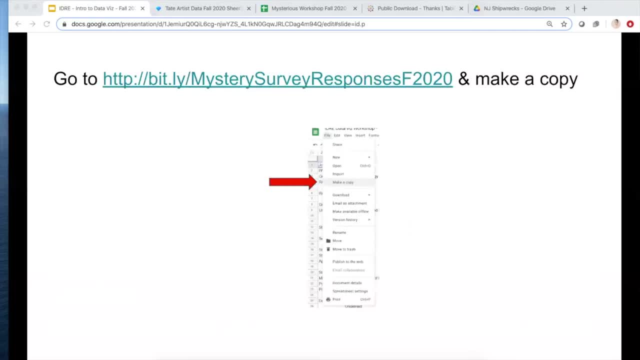 and you can take Tableau a lot further if you're doing more complex data visualizations, as you'll start to see in a bit. But pivot tables are convenient and a great place to start and can get the job done pretty well. So what I want you to do is go to 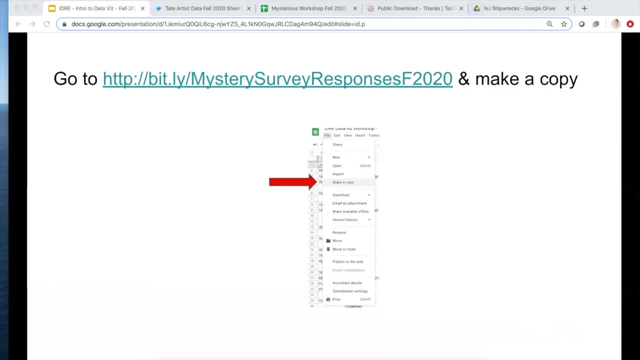 this bitly link for the responses from your mystery survey. So we're all going to be using a data set from that mysterious questionnaire and you're going to make a copy. So if you didn't take that mysterious questionnaire, I hope you go back and quickly take it. 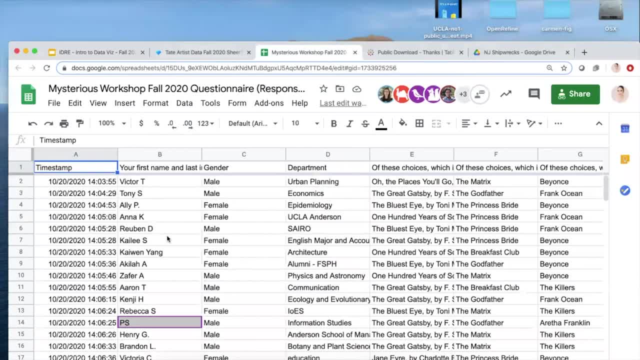 I can see if we've got it right here. Let's see. Yes, we have answers. Yay, wonderful, So this is going to be what we use. I want you to go back and quickly take that question, And I'm going to. 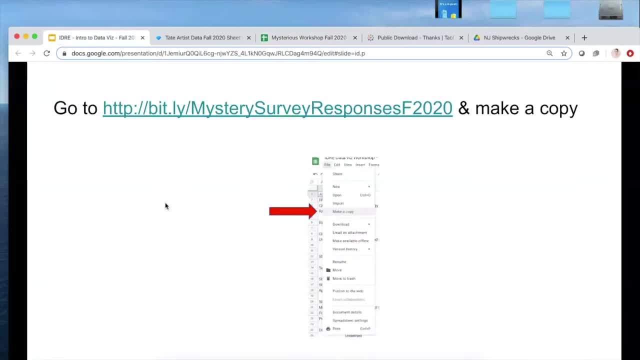 take that question And I'm going to take that question, And I'm going to take that question. So we do have a sort of canned version that we can follow along here with. I may jump back and forth between these slides and doing the live demo, So bear with me on that. 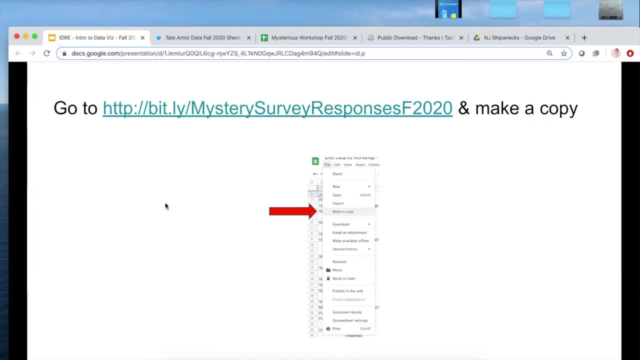 Also, the images in the slides are from another data sheet, since they knew I wouldn't have your data until the workshop. So keep that in mind when you're looking back on the slide deck later on. But definitely go into that spreadsheet and make a copy. 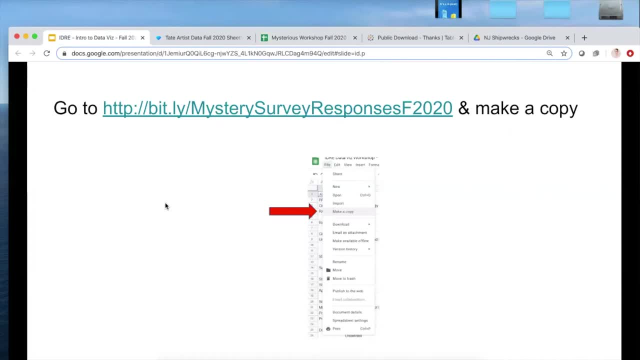 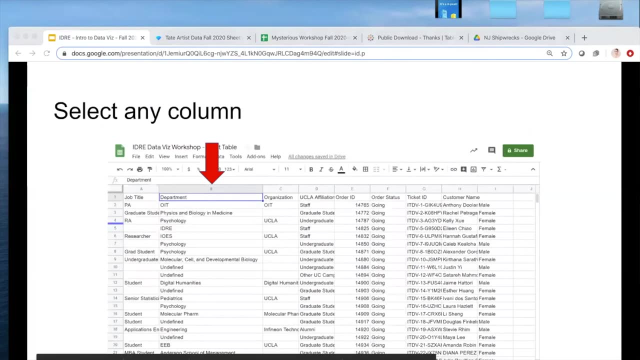 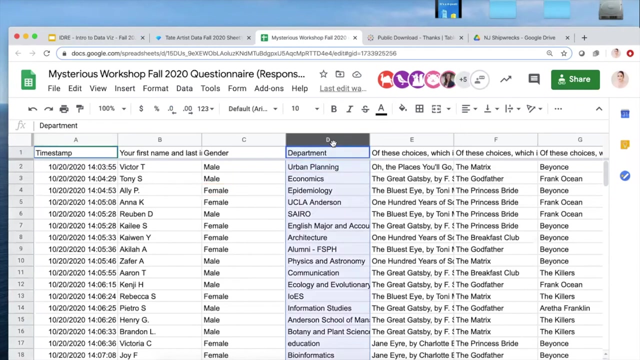 You don't want to use the same one that I'm using. You're going to make one for yourself, And so first we're going to select any column that isn't the name column. So if you want to go to department, we can go to department and select that column And you're 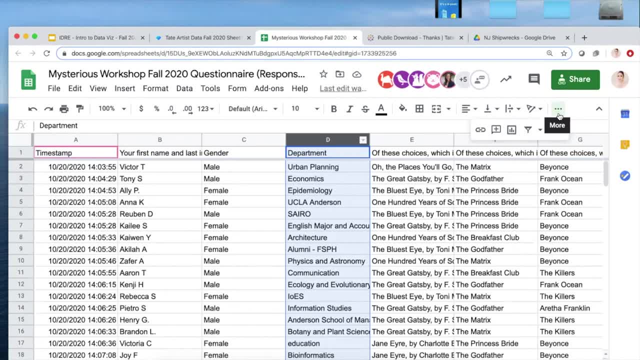 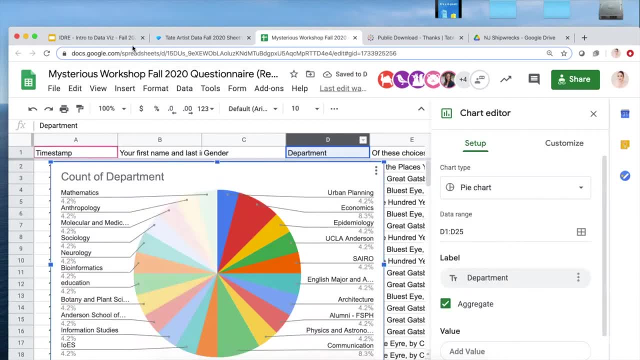 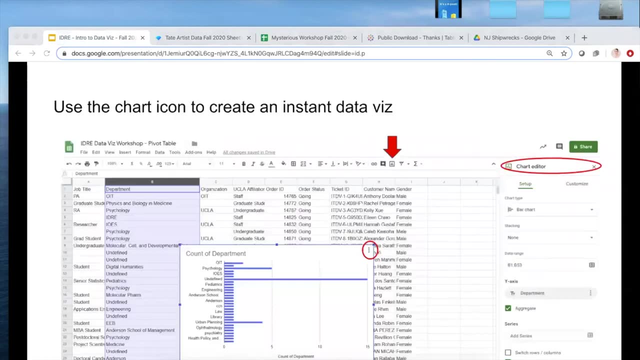 going to click insert chart And automatically we have a chart. So you hit the chart icon on your toolbar where the arrow is pointed And voila, you have a chart by count. So you also have a chart editor to the right where you can customize the chart and change. 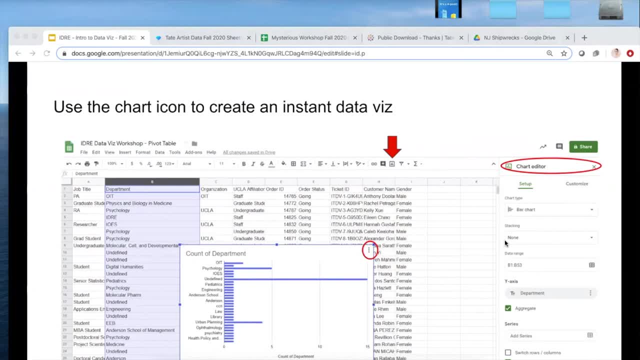 the chart type and the title and the color, all of that, etc. You also have a share. embed or export your chart in the upper right-hand corner of your chart, which is really easy to do. You just click on the three stacked dots in the upper right of your chart And that should give. 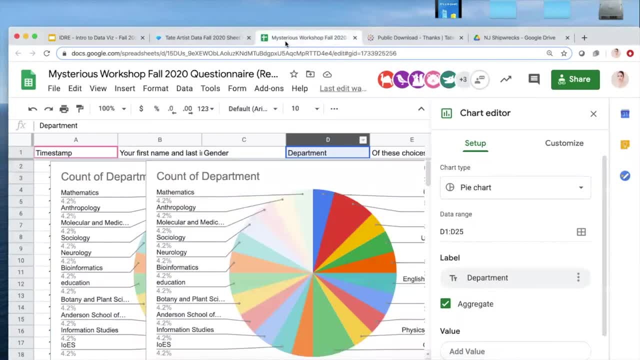 you those options. So I'm going to again go back to the chart editor And I'm going to go to the my example here. So I'm seeing duplicate charts, which means someone didn't make a copy. So you want to make a copy of this sheet in your own Google so that we're not all making charts? 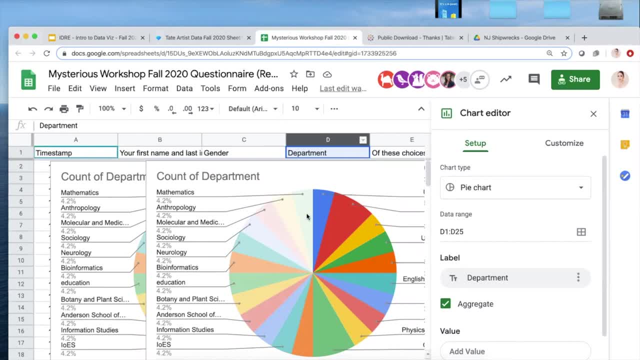 together in the same sheet. But the idea here is that right customize, If we go to customize chart style, we can change this chart style, Change it from pie slices, right chart axes, all these things. Ultimately, we don't really want to. 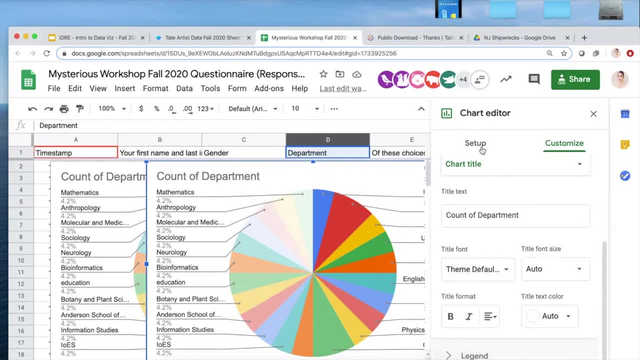 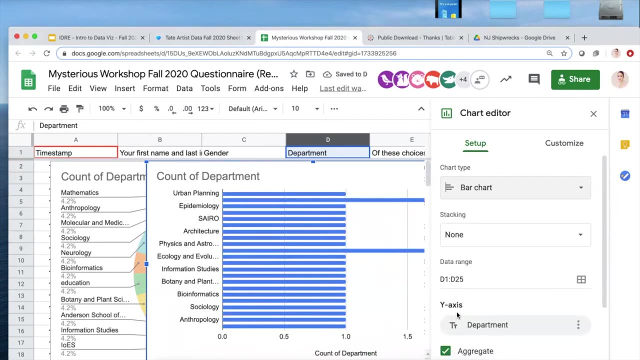 use a pie chart right in these circumstances. So let's go back see if we can switch this up. You want to switch the chart type to it's a little bit clearer as a bar chart right. And already we can see that, since everyone entered in their information on their own and we didn't. 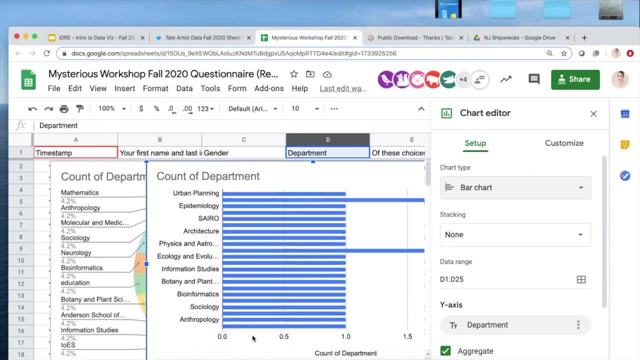 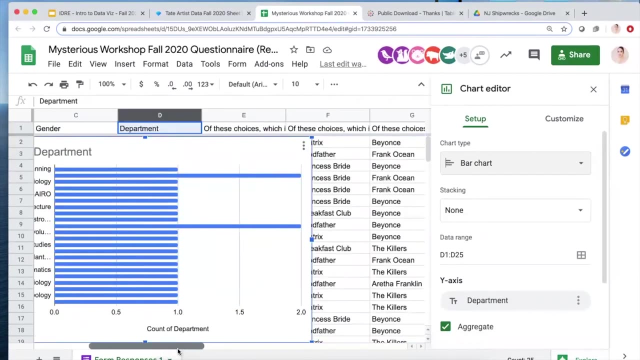 have any kind of data cleaning happening. we have actually. we have a lot of different people here from various different departments, which is great. But, point being, if I move this up for a second and scroll over, we can go to these three dots here on the left And we can see that we have a lot of 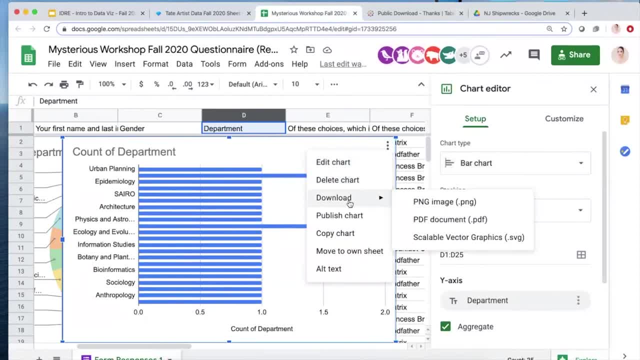 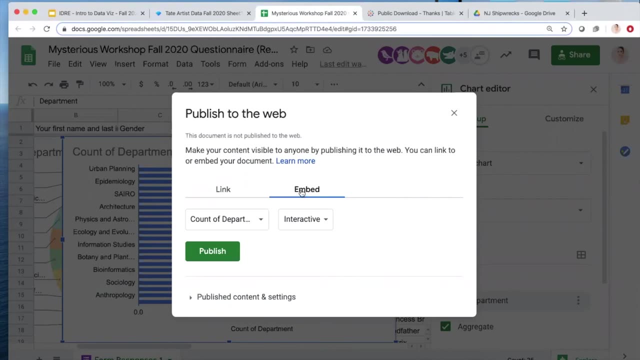 information here. So if we go down the corner and you can edit the chart, delete the chart, download it. So if you want it as a PNG or PDF, you can publish the chart, and publishing the chart will allow you to create an embed. So that's one way of being able to quickly share your chart out. 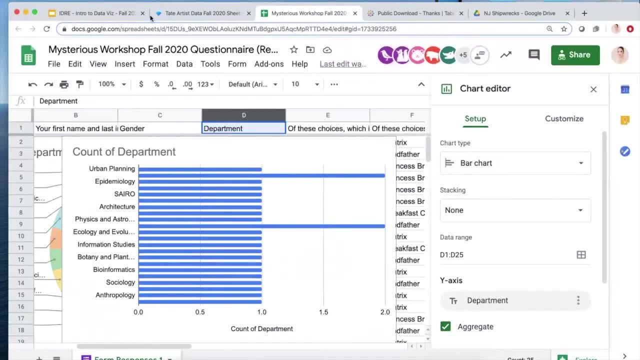 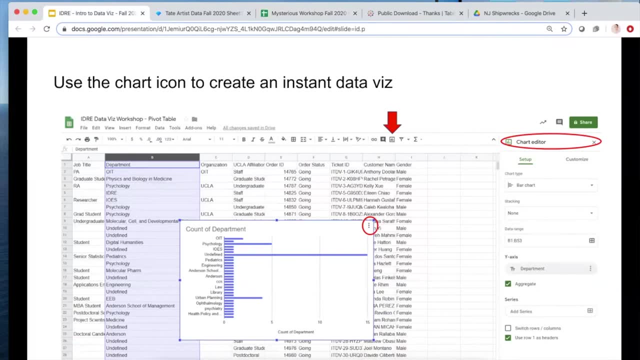 in various different forms or via link. Okay, So I'm going to go back to our slides. Did everyone log in? Was everybody able to get the copy? Yeah, Okay, Sorry, I was just seeing in the chat there was yes, Okay, great, Everybody got it Okay. 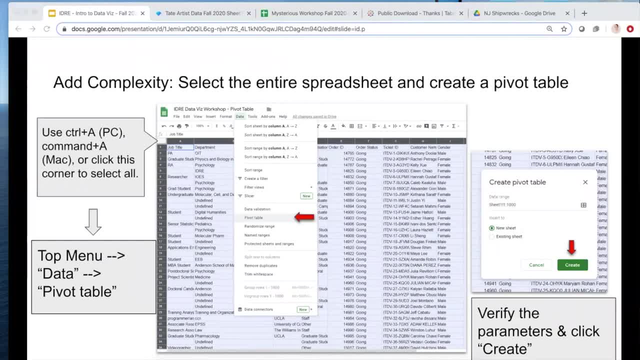 So if you want to do something a little more complex, pivot tables are really handy. So select the entire spreadsheet to create a pivot table. You can do this by either clicking this corner in the upper left or Command A on a Mac or Control A on a PC, And then you'll go to the top menu. 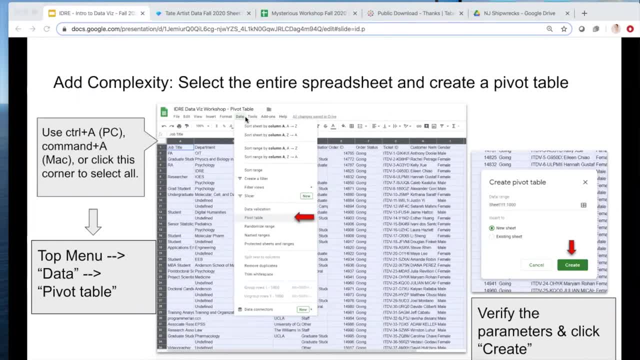 and you'll go to Data, And then you'll go to Data, And then you'll go to Data, And then you'll go to Data- Right Data- from your top menu And go to Pivot Table And when you do, you'll verify the parameters. 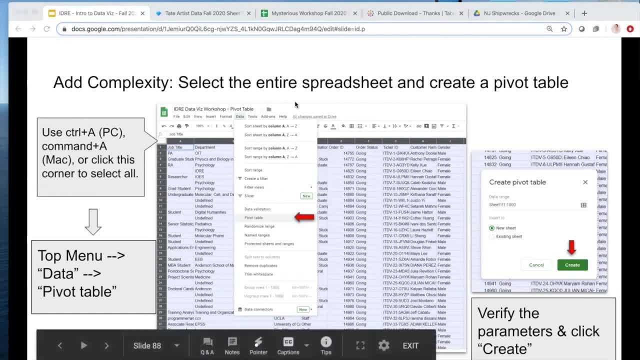 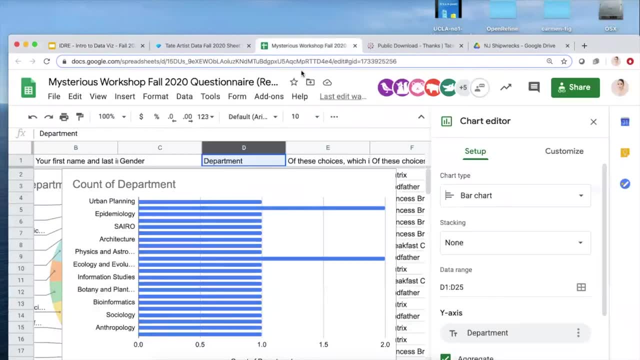 which are all fine as they are, and you'll click Create. So if everybody goes and does that, I'm going to pull my get my window down so I can access my menu here. I'm going to go ahead and delete these, so they're out of the way. 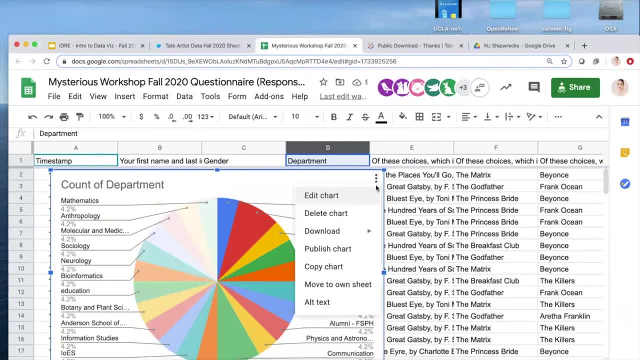 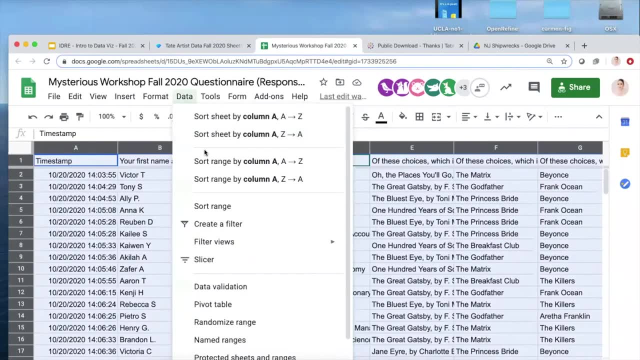 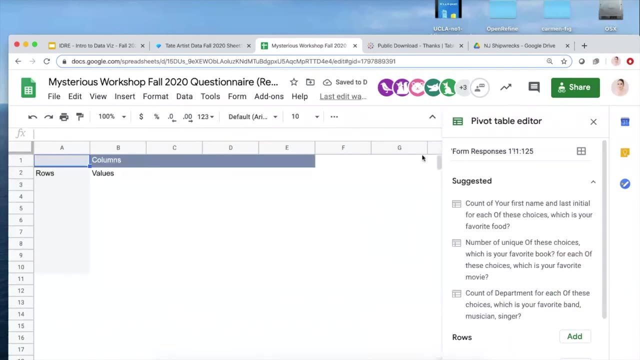 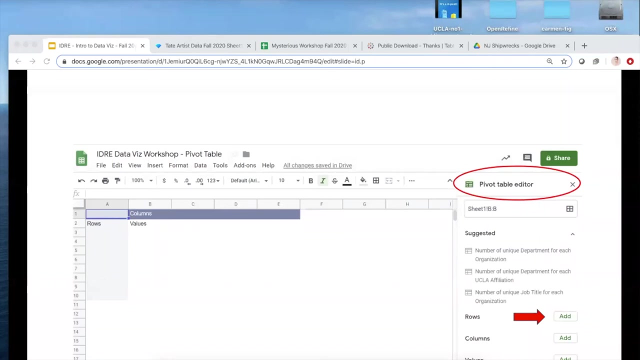 Okay, Okay. So to do this, I'll click here, select the whole thing, go to Data and Pivot Table. Click Create So it starts my pivot table in a new sheet, Right. So once you're there you'll have similar to your chart editor: you'll have a pivot table editor. 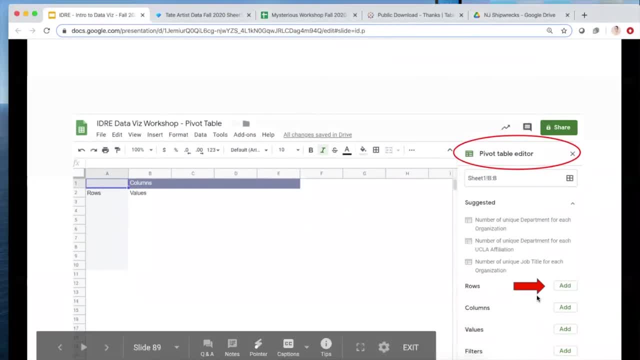 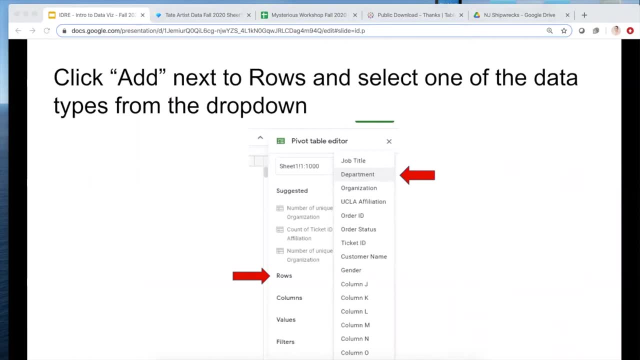 And in your pivot table editor you're going to want to go into Rows and you're going to click Add And you'll select one of the data types from the dropdown. I recommend you can start with Department, but you can really do whichever one you want. 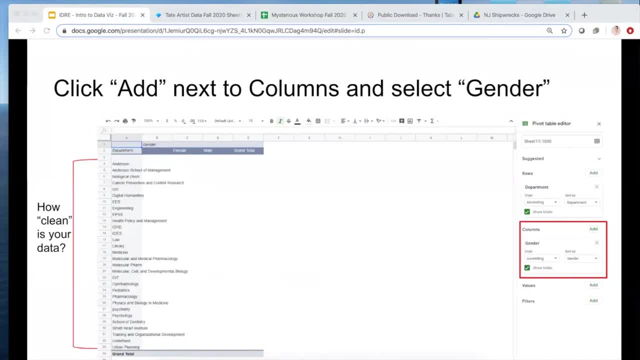 And you click Add to the columns and select Gender- Let's try Gender right Or something of the like- And if you have used the department content type under Rows, you may see that your data probably needs some cleaning like this. Likely you will see something where there's in this example we have right here, Anderson & Anderson School of Management. 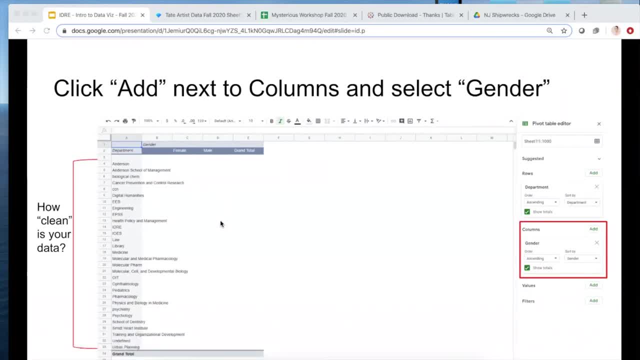 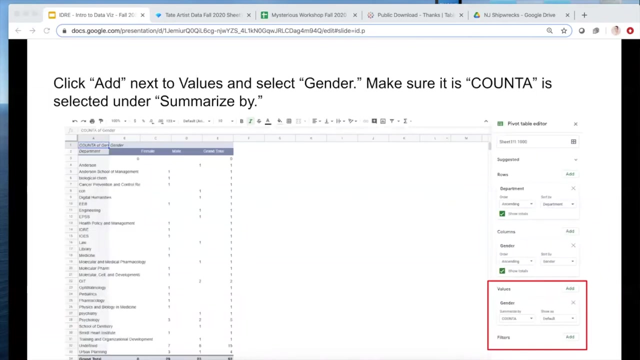 Or molecular farm and molecular and medical pharmacology, So we really should combine those things, because these are referring to the same departments. This is why it's important to clean and standardize your data right before visualizing it. So click Add next to the values and select Gender. 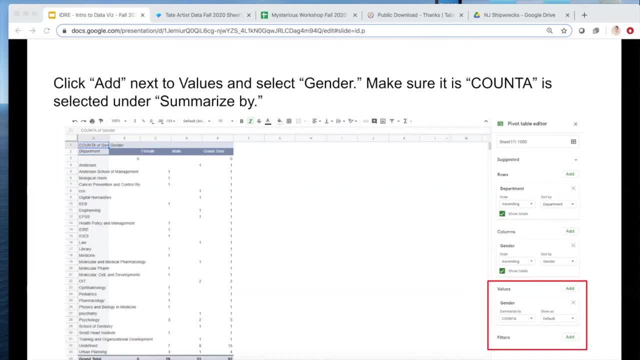 And make sure it's a count A is selected under Summarize By. So, in case you were wondering, the difference between them is that count only counts cells containing numbers, But count A counts all cells that aren't empty, So think of it as count anything. 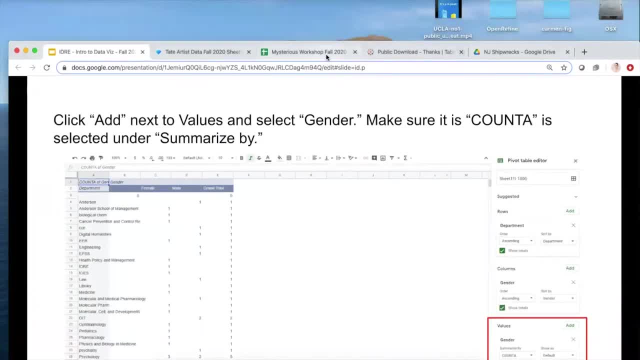 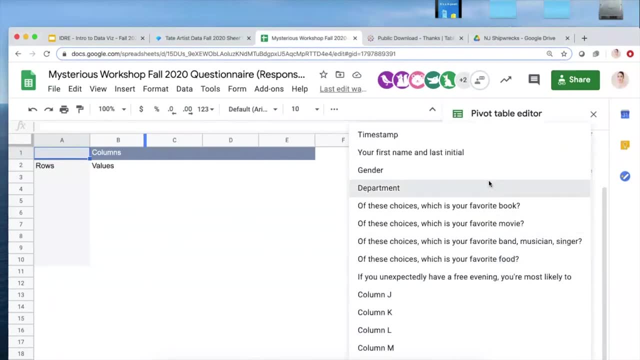 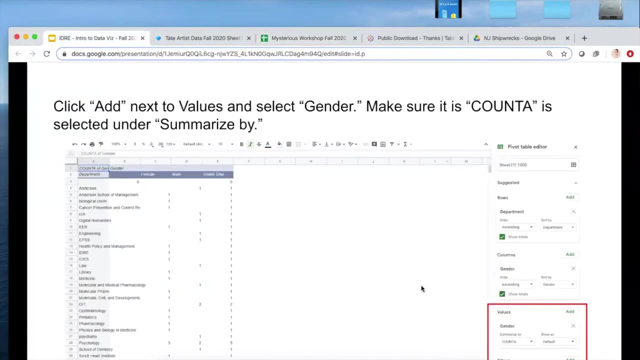 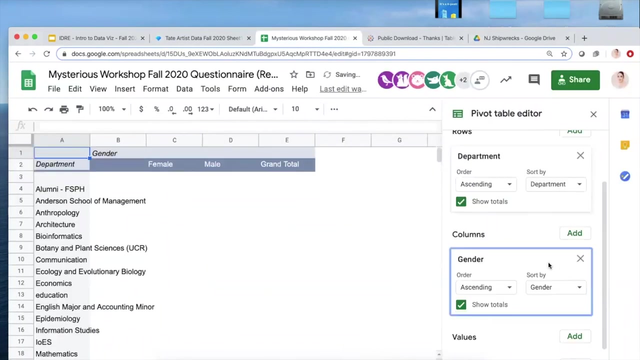 So I'm going to quickly go over to my sheet and try to do this with you all. So Rows, Department, Right Again, Columns: I'm going to add gender And then values: I'm going to add Right count A. 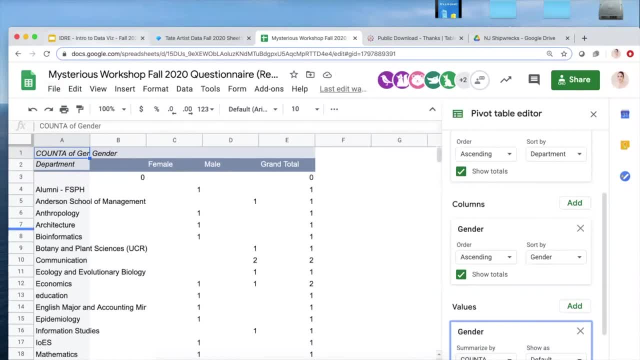 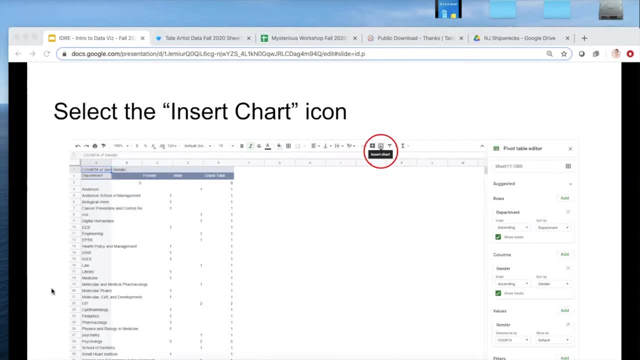 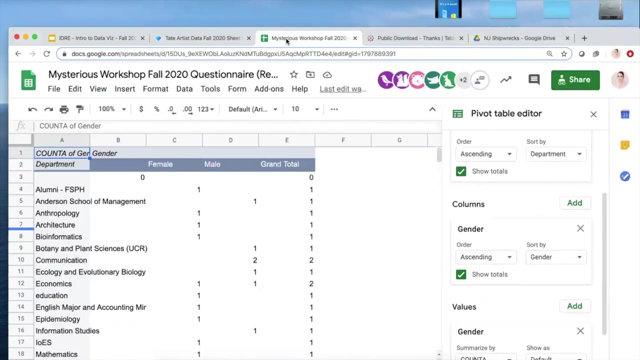 Okay, So we have those things. So once we have that, we're going to select the Insert Chart icon again And you'll have a stacked bar chart as a result. So here I'm going to use the dot dot dots because my screen is kind of squished. 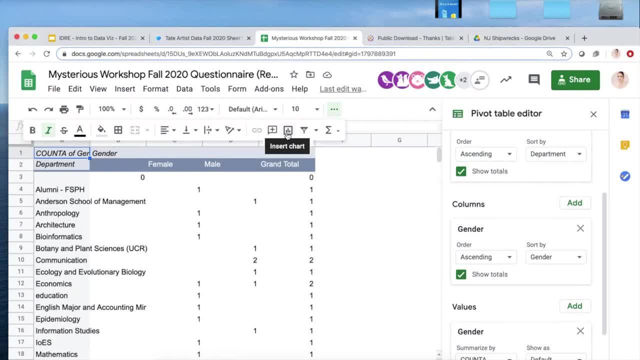 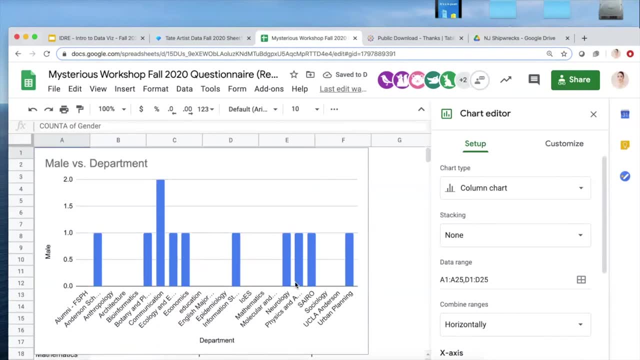 So Google has put it all under the second level. I can do Insert Chart. Oh, no, Not yet. Oh, and I'm not getting this. Why is that? Is anyone else having an issue with this? Oh, I'm sorry. 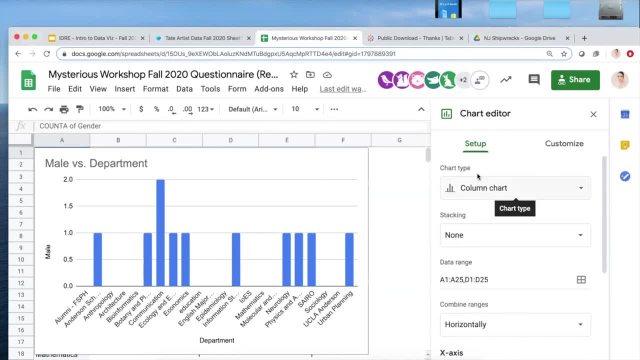 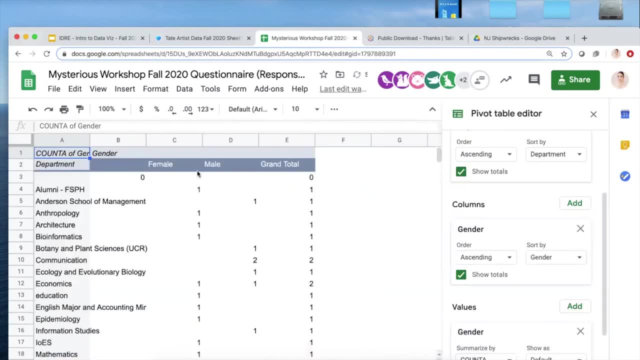 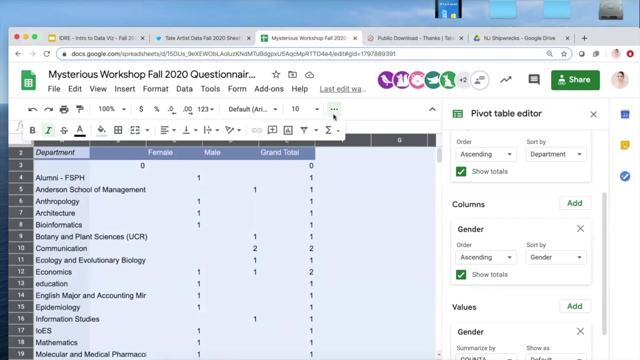 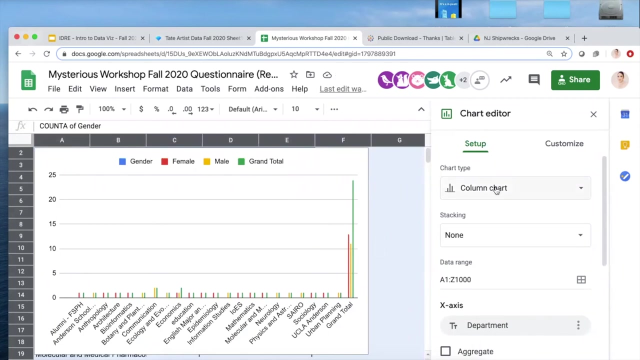 This is because I picked Mail One second. Let's go back. Let's do this again. Law of demos. All right, So I want to make sure that the whole pivot table is selected, So I'm going to leave some of these. 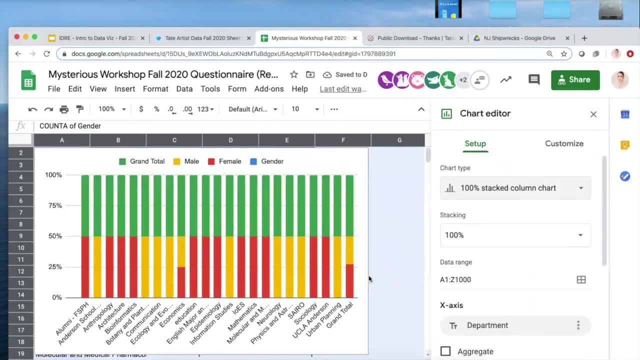 And then I can select. There we go. So I also have my grand total here, because I've selected everything. But you can see, it just depends on what you've selected and that's how it will create a stacked bar chart for you. 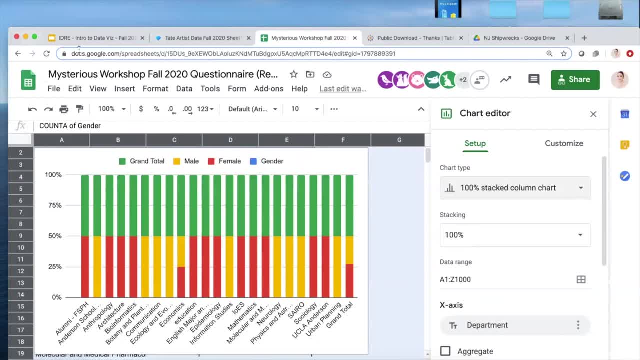 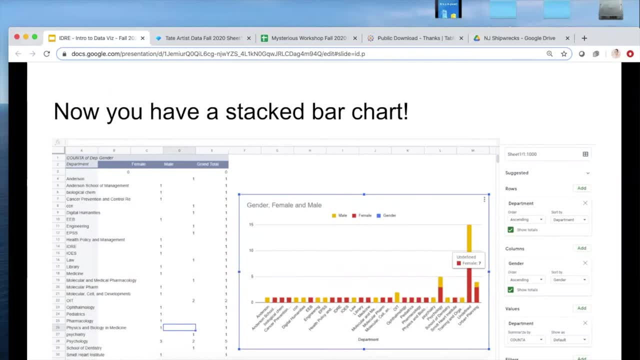 Is that clear? Yeah, Any questions on that? before we move into Tableau: Awesome, I'm glad you guys are enjoying. Okay. Well, let's move into Tableau, because if you think this is cool, Tableau is even cooler. 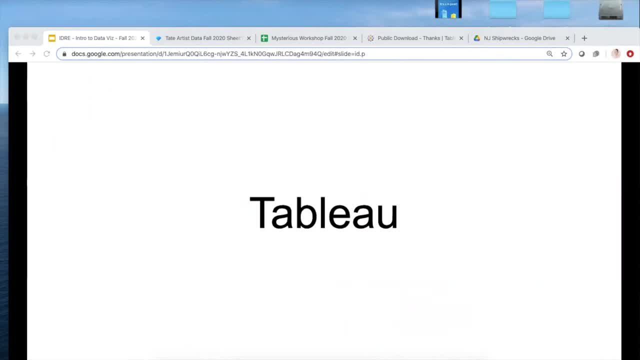 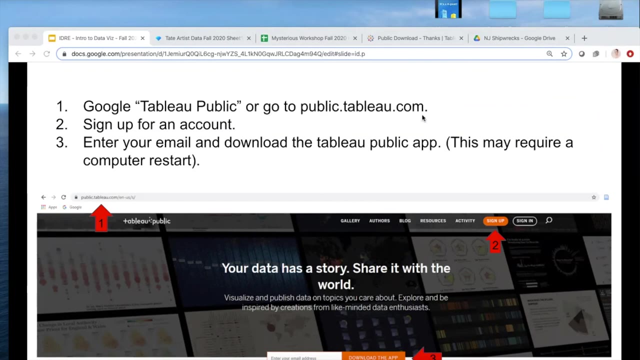 So Tableau is an industry standard for data visualization, So it's really a good one to be familiar with. If you haven't had a chance to yet, go to Tableau Public- Google Tableau Public- or go to publictableaucom. 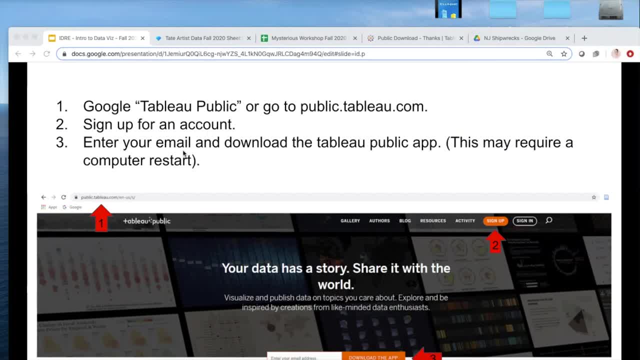 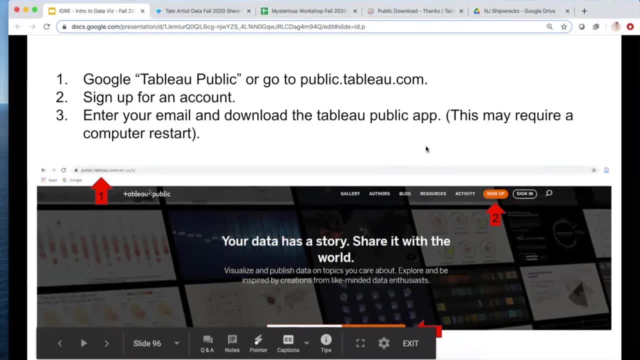 And you can sign up for a free account and enter your email to download the Tableau Public app. This may require a computer restart, So if it does prompt you to do that, you can do that. If it does prompt you to do that, you're welcome to just follow along with me. 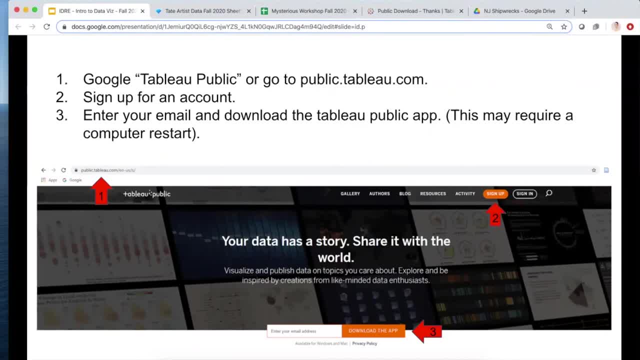 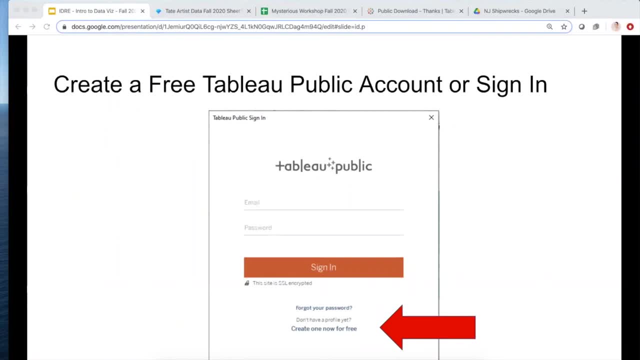 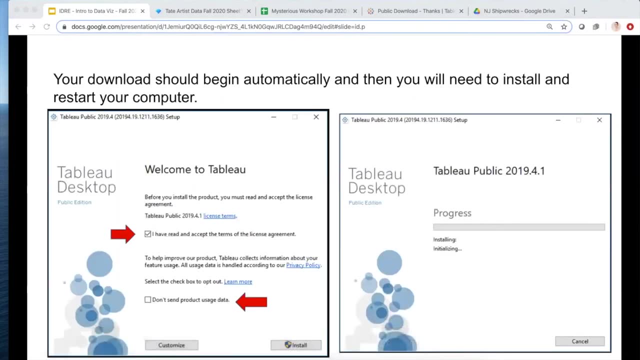 I'll give everybody a second to go ahead and do that. So when you create a free account, you can also do it down here, And your download should begin automatically, And then you'll need to install and restart your computer. So does anybody need a few more minutes to do that? 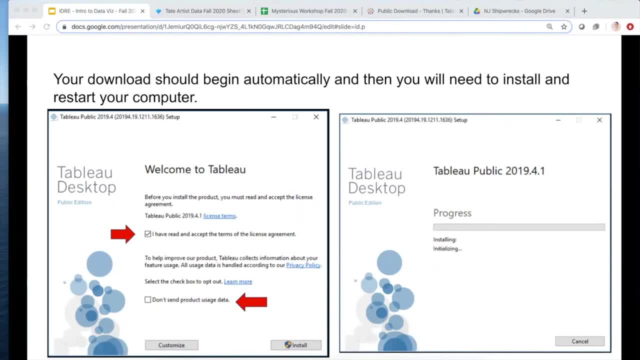 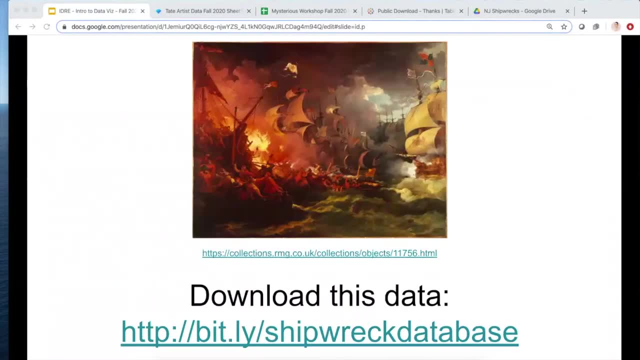 I just want to check. If not, I'll move forward. Everybody's good, Okay. So if you are still installing, go ahead. If not, let's download this data set. So this link will take you this bitly link which is blocks. there we go bitly to Shipwreck Database. 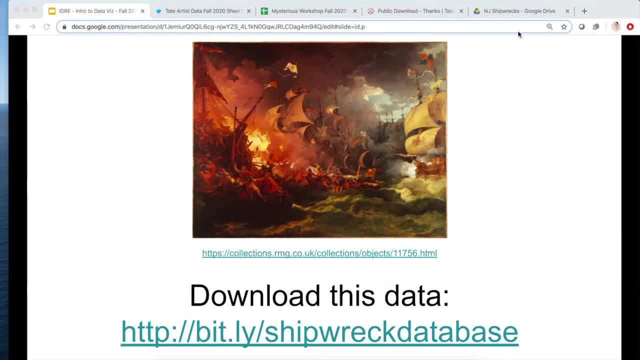 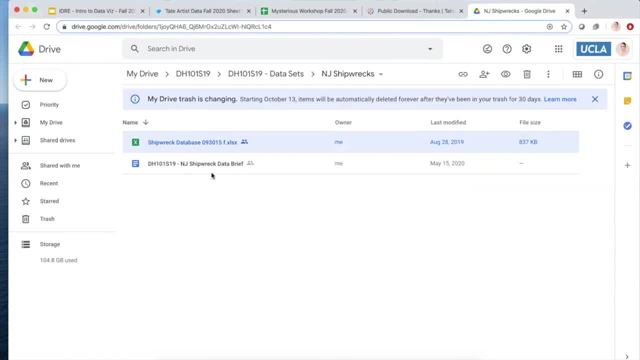 This will take you to a folder that will have a sheet that you can download, as well as a brief. if you want to know a little bit about this New Jersey Shipwreck Database, which is very, very cool. Does anybody need the link to this? 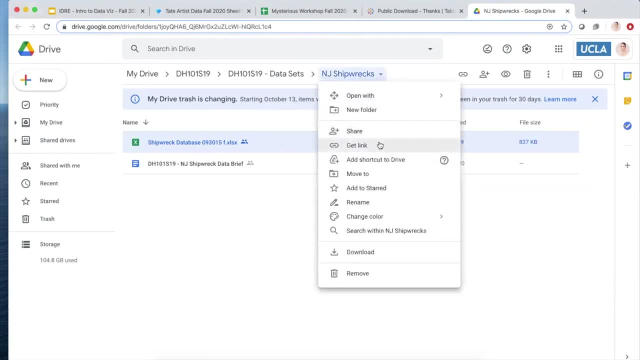 I can send it to you if you. I'll do this and I'll put it in the chat. Okay, So you can go ahead and download that Shipwreck Database. That's what we're going to be using for our Tableau tutorial. 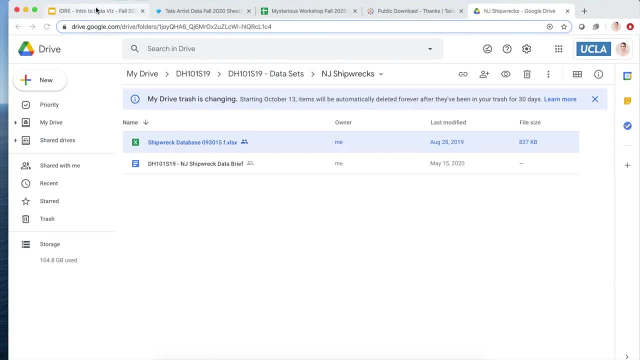 And again, I've canned all of this on slides. I will try to navigate back and forth between Tableau, but I know that we're running low on time so I may move kind of quickly through the slides. allow you guys to follow along with me via the slides. 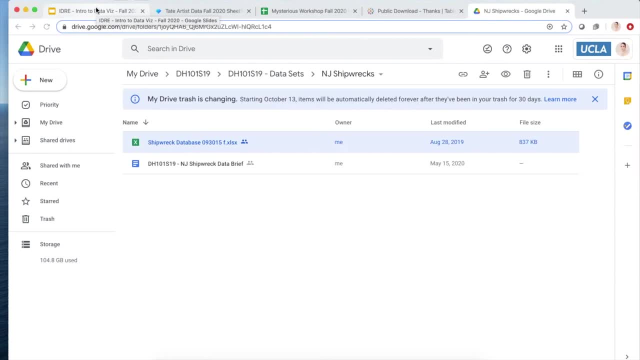 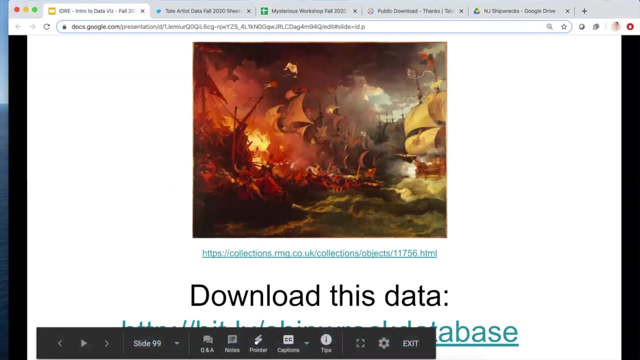 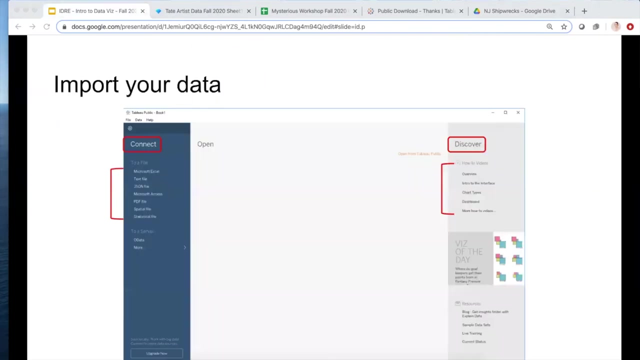 and let me know if you have any questions as we go. And if I have to jump into Tableau and do it, then we'll do that if we're running low on time. So You're going to start once you have Tableau. 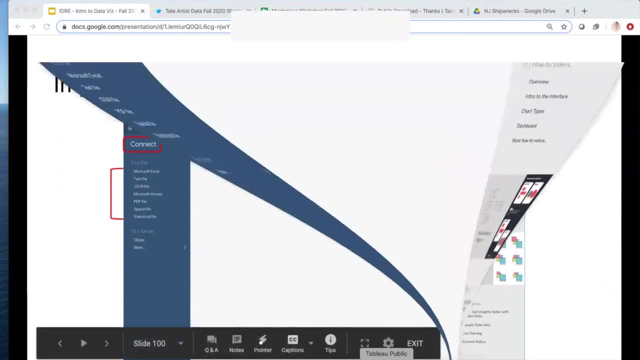 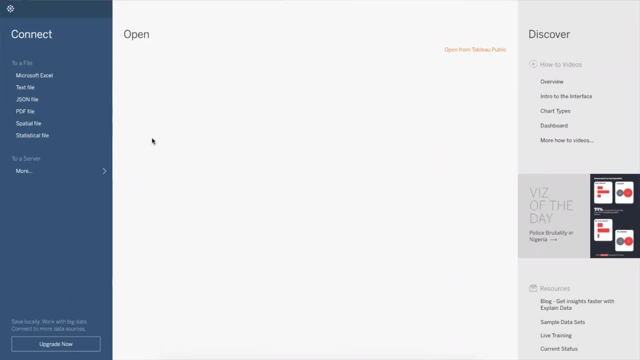 the app should look something like this, And when you launch it you should see a screen like this. So on the left you can import many different file types and you'll see that on the left-hand screen, And we're going to be using an Excel sheet, so you're going to want to use that one. 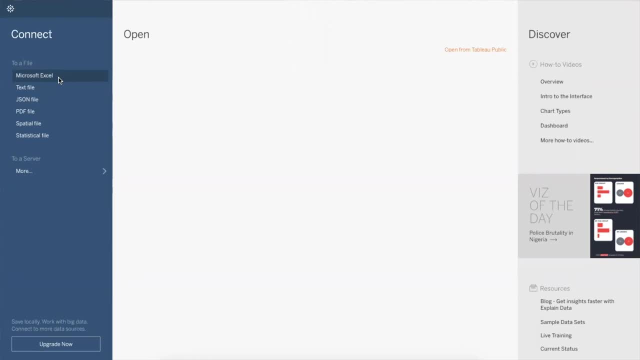 But I also want to note that you have a great repository of tutorials and resources from Tableau Public and they're over here on the right-hand side. I'll cover the basics today, but if you want to keep going, I recommend you explore these. 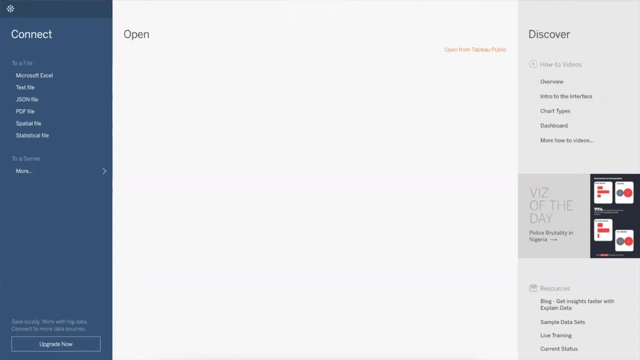 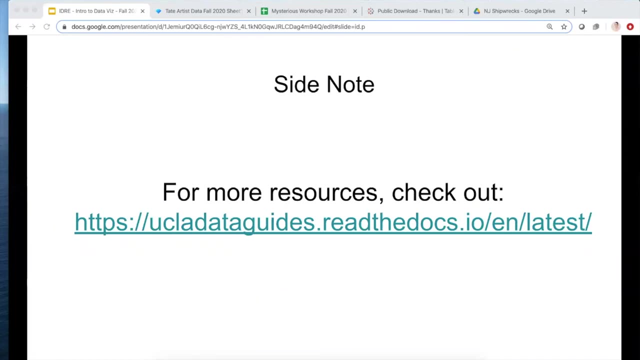 They're really wonderful. And in addition, side note for more resources, a colleague of mine- several colleagues of mine at UCLA- have put together some additional guides through Read the Docs. Definitely check these out. They'll cover some of what I'm covering, but also other things as well. so good variation. 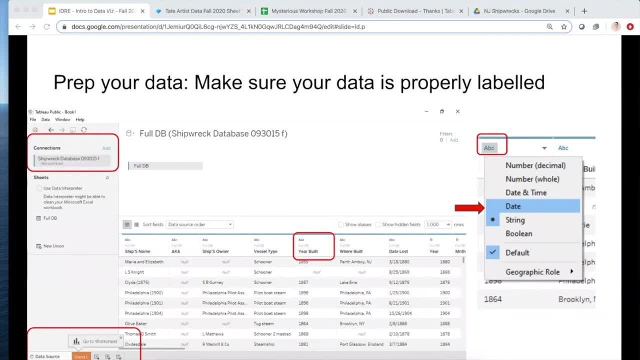 So if you have multiple sheets of data that you want to work with- say if you're working with a relational database, for example- you can connect them within Tableau, which is why it's so powerful. If you also, or for almost any data visualization tool, 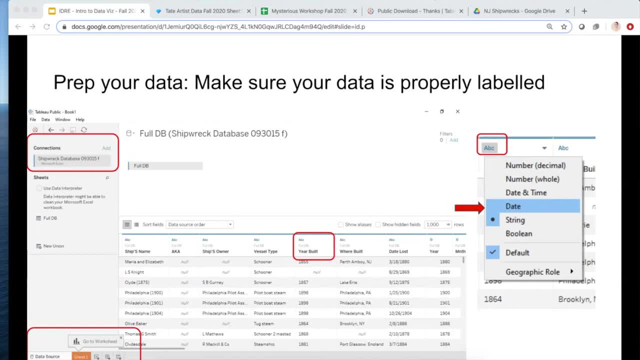 you're going to have to spend some time though formatting and labeling your data for the tool so it understands how to read it right. Computers are not smart. Programs are not smart. We make them smart. So you have to train the tool and tell it exactly what you want it to do. 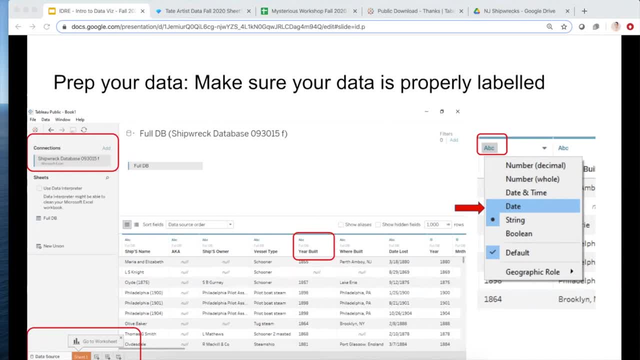 When it inputs your data, it will try to best approximate what it thinks it is, but, for example, year built right is obviously a date. It's not a text and right now it's labeled as ABC, which is a text label. 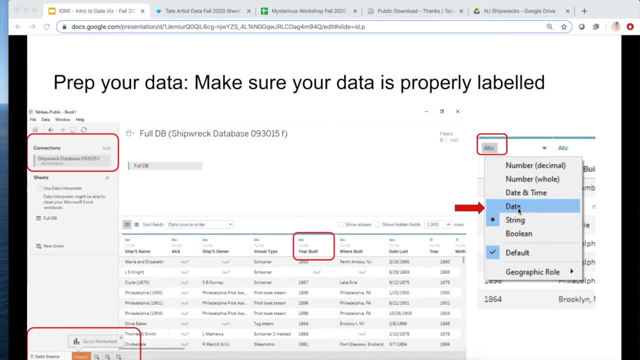 and you'll want to go and switch it to date so it understands that it's a date and it should be read as a date. So we're going to spend some time doing this when we use the bottom menu to create our own worksheet. So you can create your own worksheets down here at the bottom. 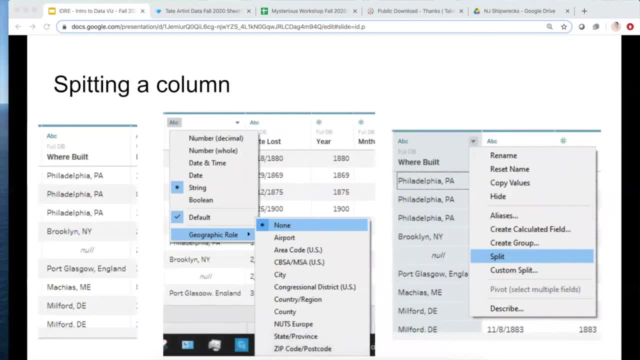 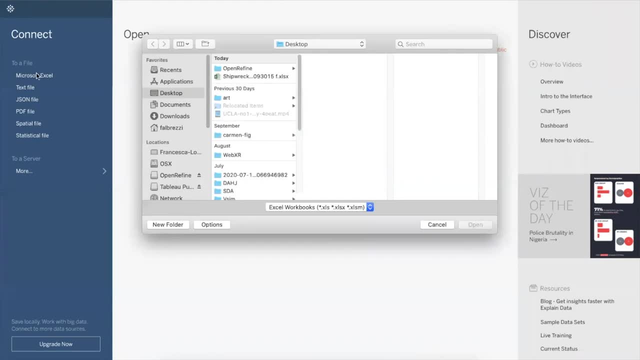 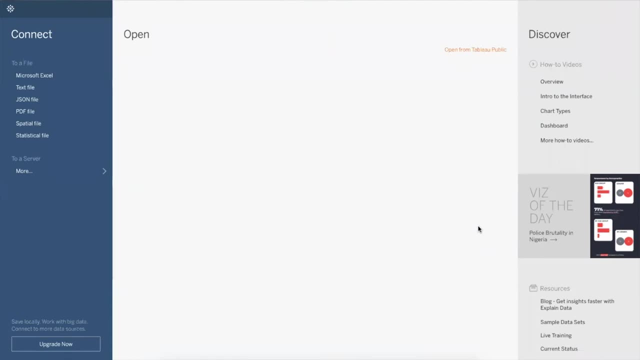 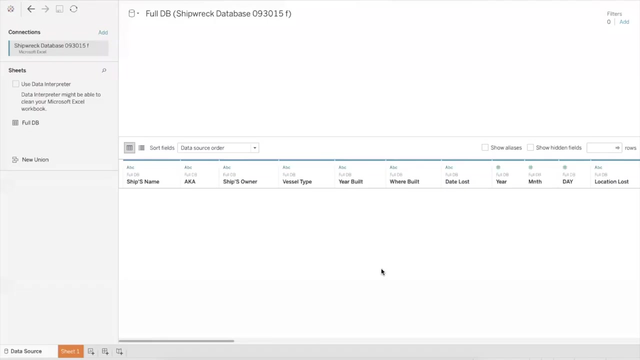 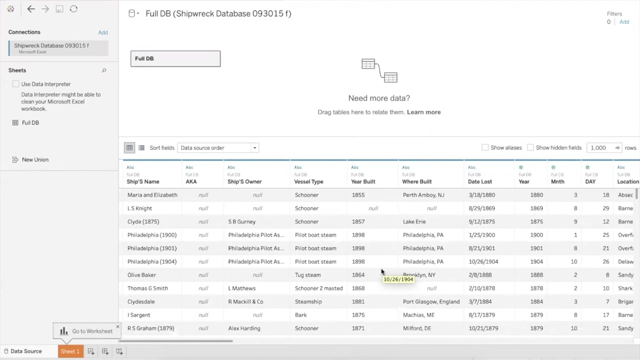 So, first and foremost, we'll show splitting a column. I'm going to actually go into my Tableau and get my dataset input So I have my ship database Right Open. that Take a second here And there it is, So I have my full dataset. 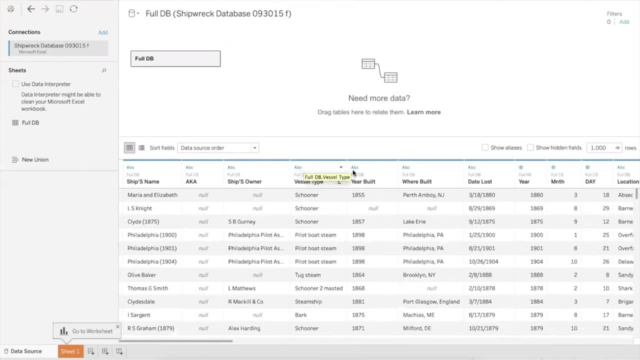 And, like I said, I have these labels at the top that I'm going to want to adjust for my dataset so that Tableau understands what kind of data it's working with. So, in terms of preparing your data, oftentimes you'll see two types of data within a single column. 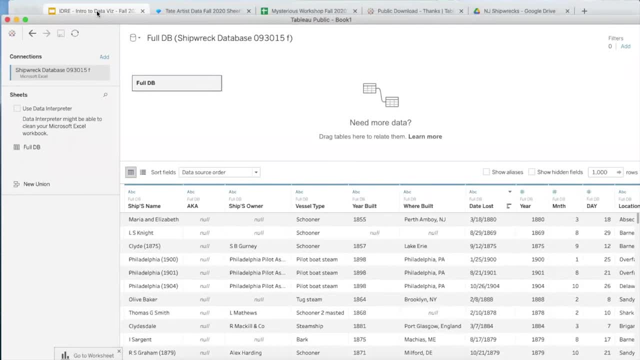 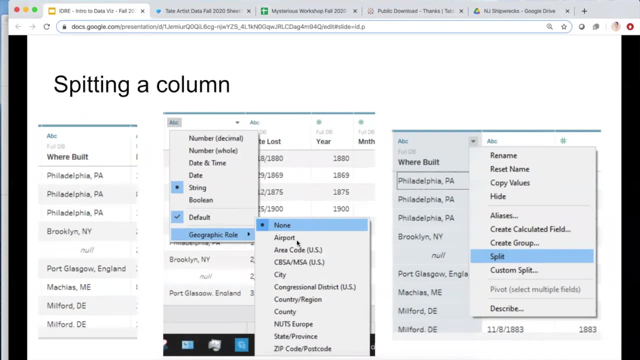 And I'm going to quickly switch back to my here. So, in order to read it, Tableau needs city and state to be separate If we want it to work with the geographic, if we want it to work specifically with our geographic data right. 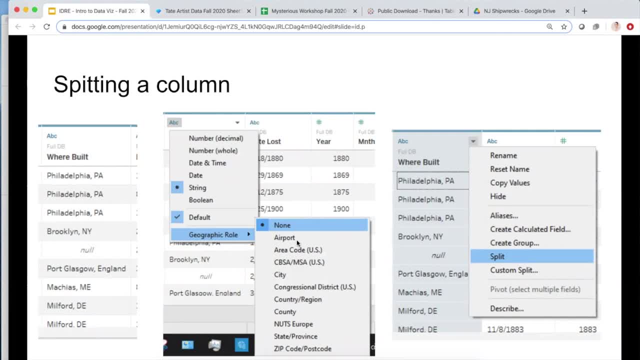 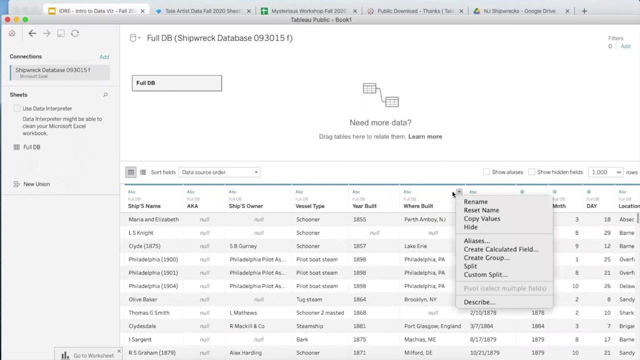 you can edit by clicking down the arrow at the top of the right of the column and choosing split, And that will separate those things. So, for example, we're built, Let's separate that column. We're built right, Split, Right. 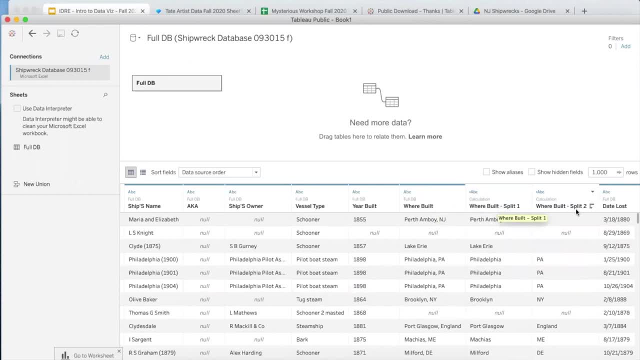 And now we have: we're built one and we're built two. So we want to rename these things so that we understand that this is the city and this is the state. We can also relabel it in terms of its data type. So rename. 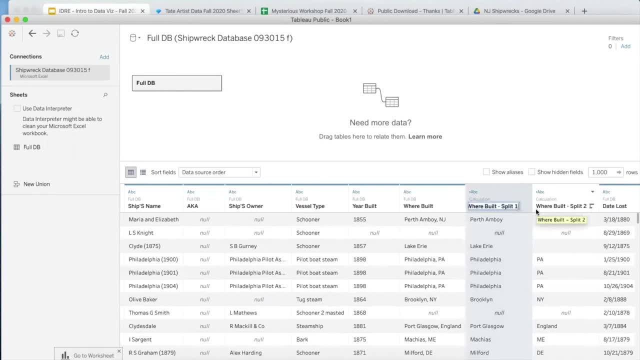 Right, We can say we're built city And then rename We're built state. Everybody got that. We can either delete or keep this original column, just in case if we want to have it as a backup And then we want to switch the type. 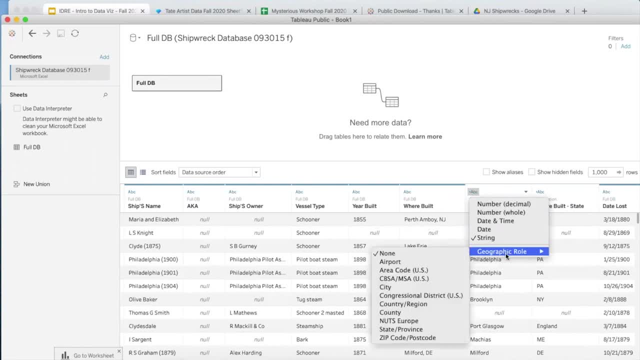 So we click on this right here And we want to tell it that it's a geographic role And the geographic role is city. That way it can go out and it can find those Latin longs for us And the same thing, for we want to say state or province. 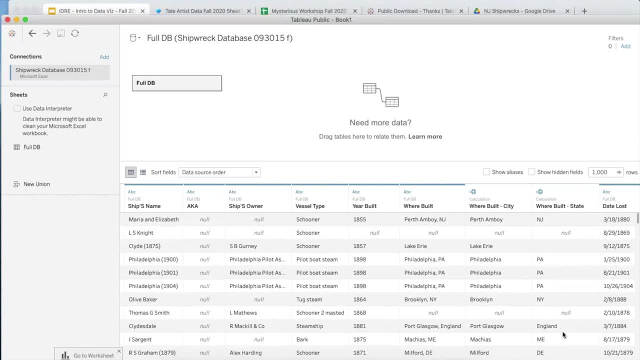 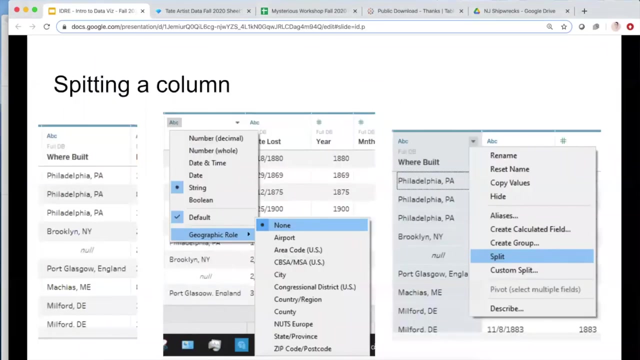 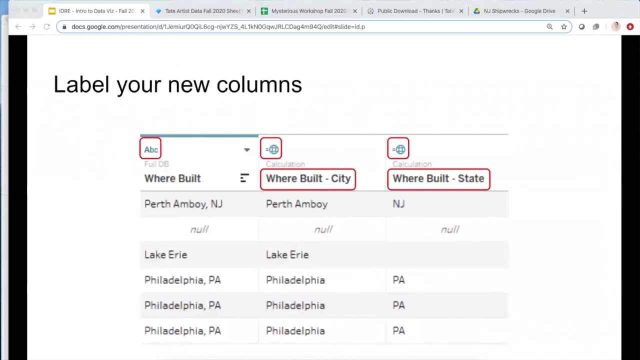 Some of these have England, so it might have some difficulty with those, But for the most part they're states, So that's all good People following along with that. Does that work out for everybody, Okay? So, as I said, we should create two new columns and double click on the column title to rename it. 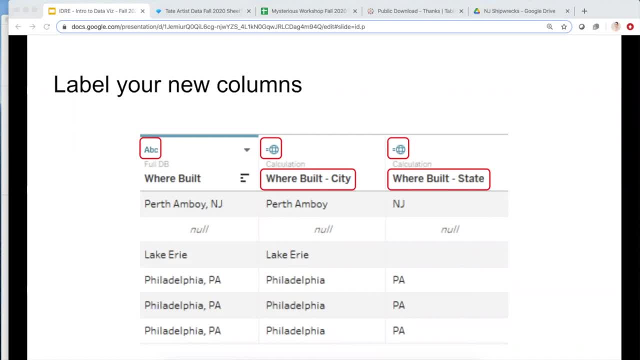 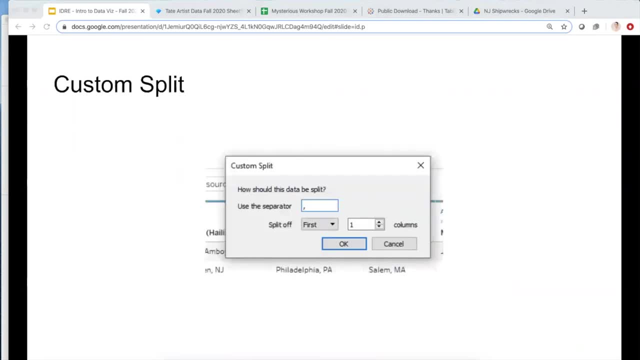 And then next we'll relabel them. We relabeled them as geographic data. One is city and the other is state. So if you see some issues within your automatic split, you can create a custom split instead. So, for example, between first name and last name, you can just use the space as a split if that needs to be. 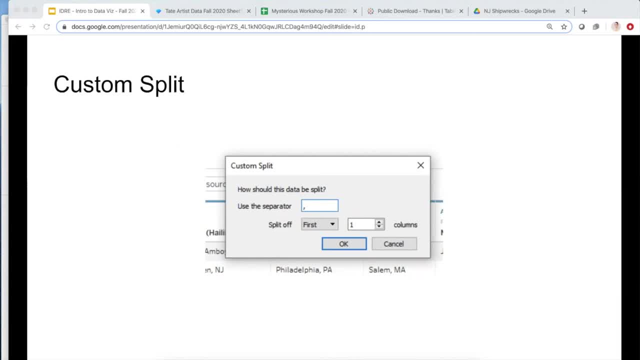 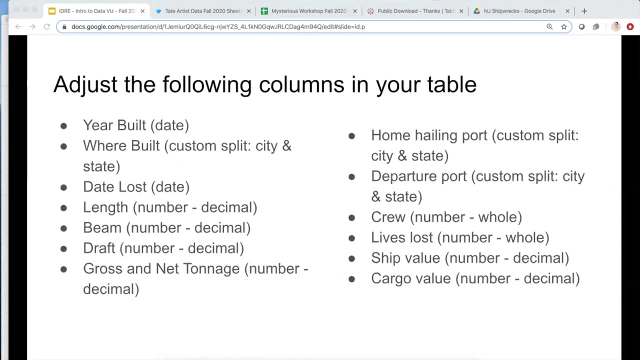 Or New York, New York comma, New York, Right That those You don't want it to split at the space but at the comma. So you have to sort of pay attention when you're working with custom split. But you can enter in a character that you wish to use as the separator and choose if you want it to split into one or multiple columns. 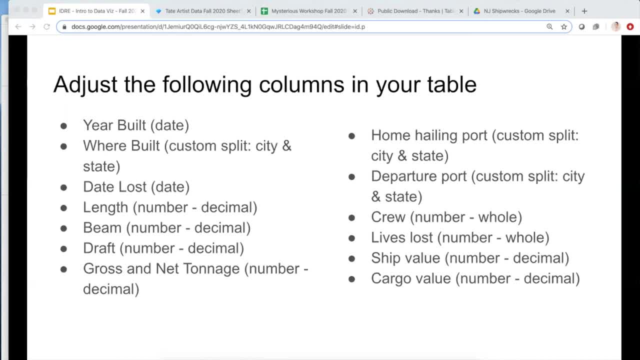 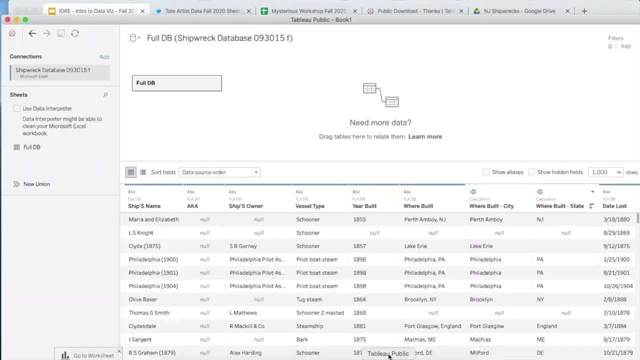 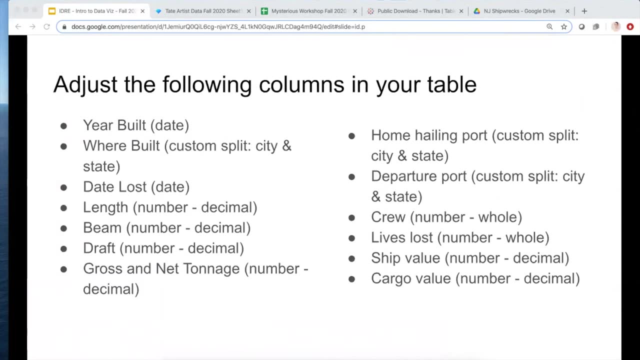 So let's take a few minutes now to adjust the following columns in your data table. So I'm going to take my tableau public here and I'm going to drag it off screen so you can't see it, But I'm going to make the adjustments along with you. 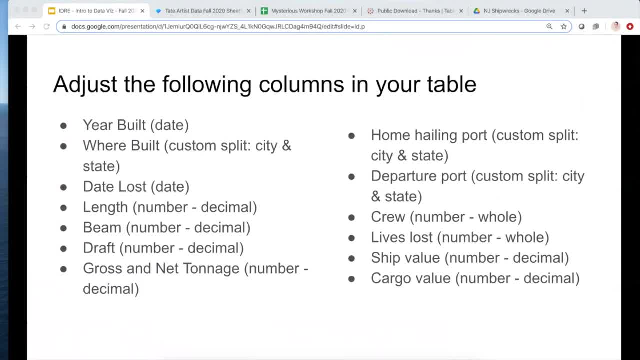 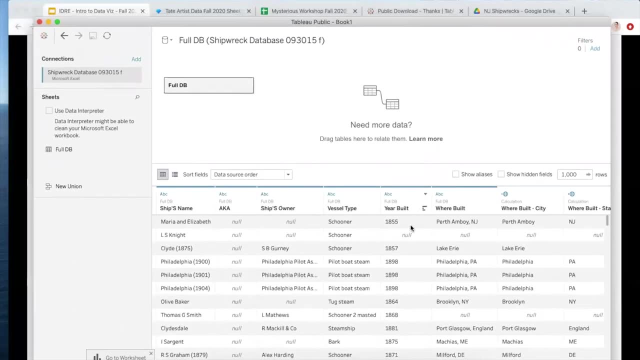 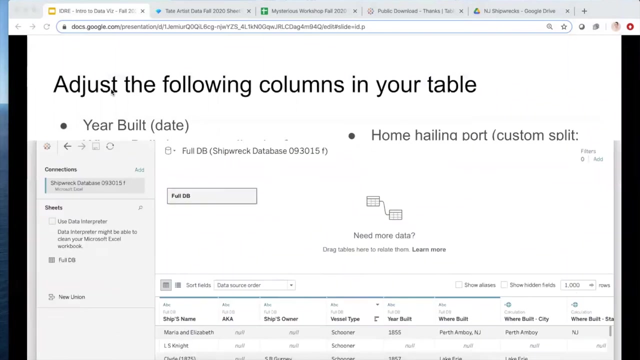 That way you can be looking at the table as you go through. So we'll first adjust the year built. So everybody go in and change that Quickly, show you. So we're going to change that year built. Right, We want to change it to a date. 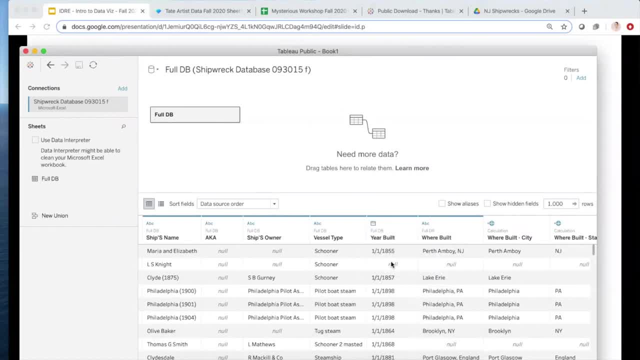 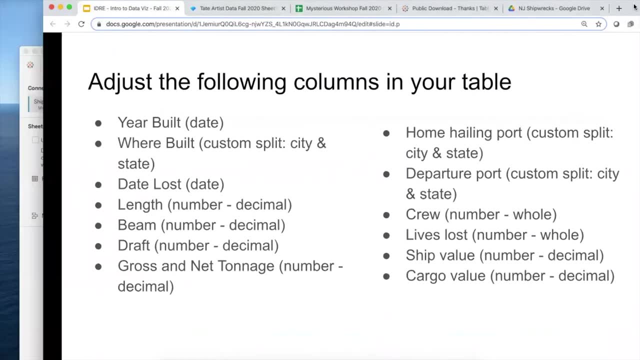 So clicking here change that to date. I'm just going to go back and forth a little bit so that you can see what I'm doing and then I'll move it off screen so it's not so confusing. So where built? we want to do a custom split right between city and state. 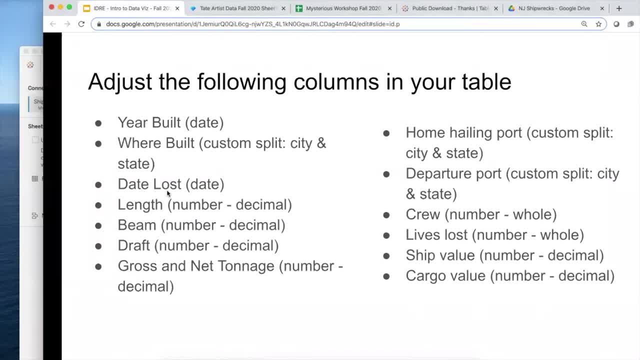 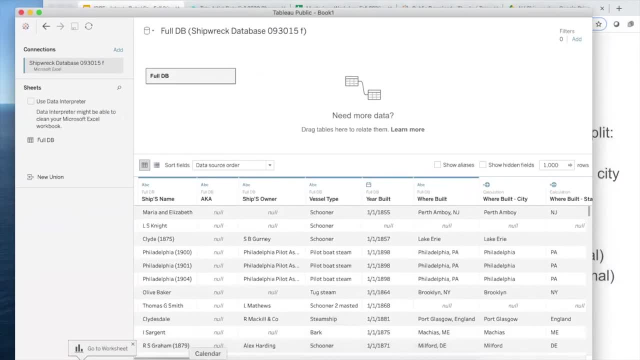 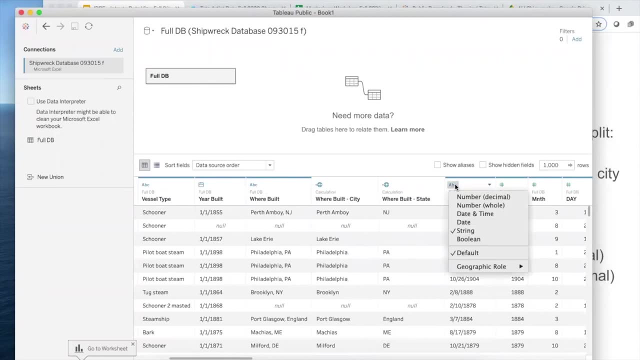 We did that. Of course, if a data is Lost, we want to acknowledge that as a date. So when our data sheet is long like this, we can just scroll using the bar at the bottom. So we want to switch date lost to date. 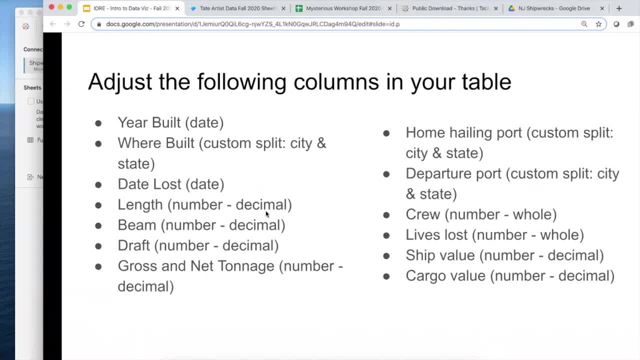 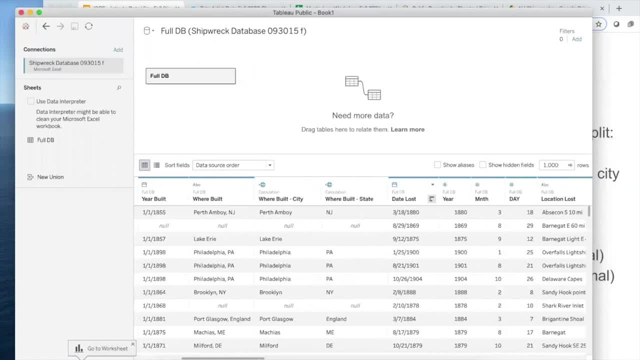 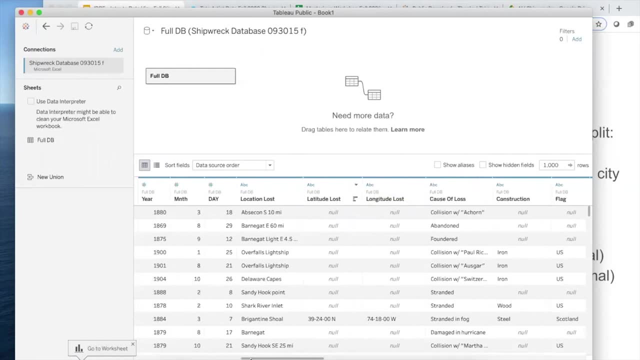 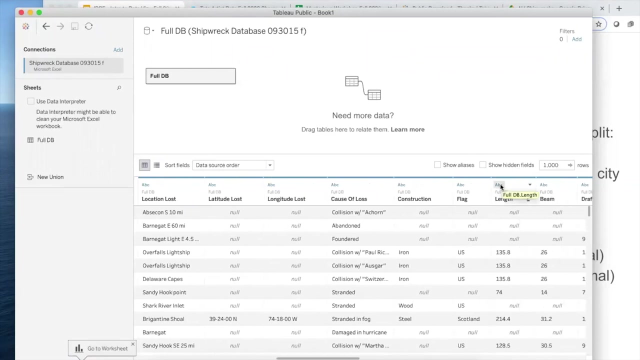 Now see how that's all reading as a date now, Like that. So these are all labeled as numbers. that's okay for now. So we want to switch that to number decimal Because we understand that the length of a ship can be longer, right- than a whole number. 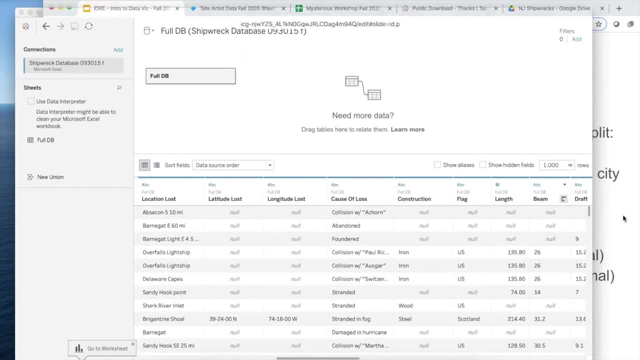 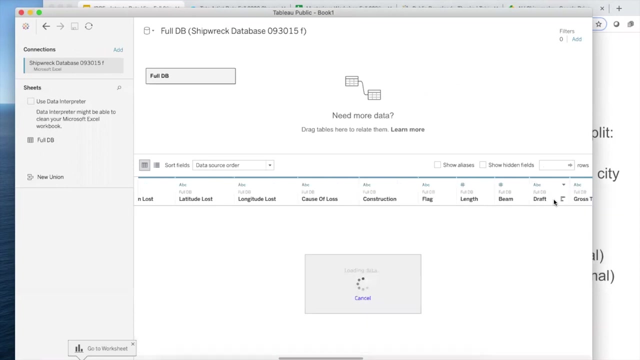 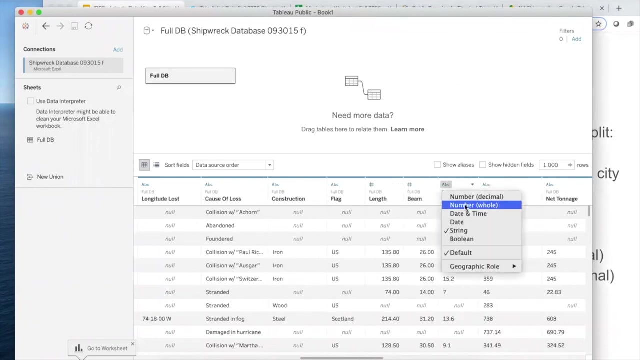 It obviously has a decimal. The beam in the same way and the draft in the same way. All right, so let's transform those. transform them to number decimal rather than number whole right? Are you able to follow along? Everybody getting that? 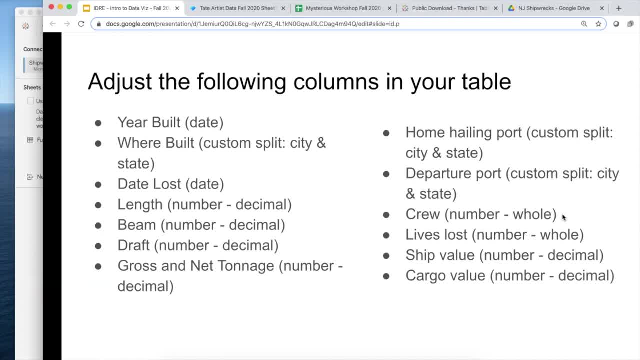 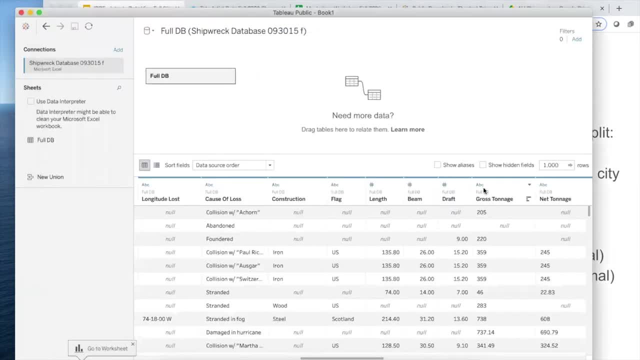 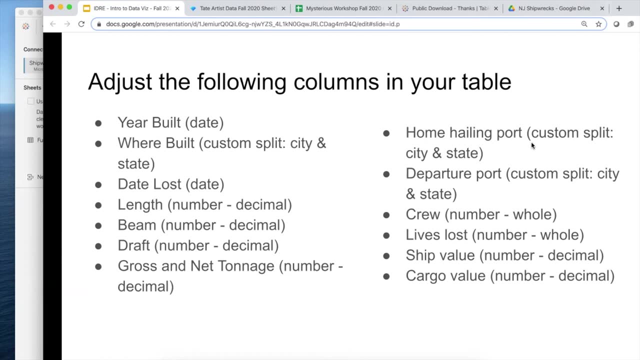 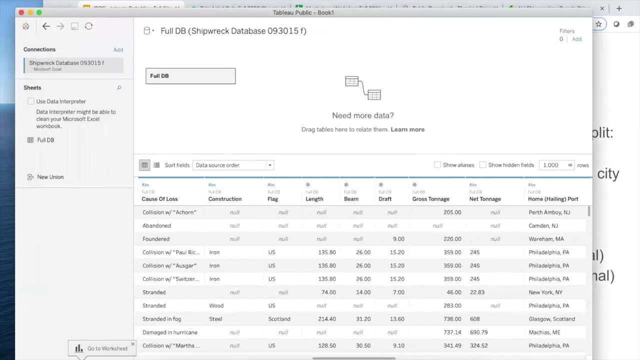 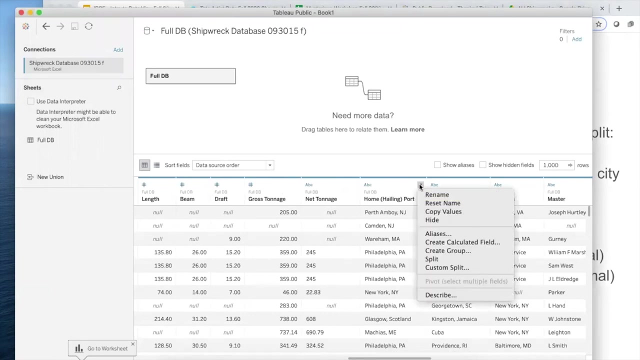 Any questions? Okay, so then we have gross and net tonnage. So again that's also going to switch to be a number decimal. Home hailing, port: This we're going to custom split between A city and state. So we do that by going to the drop down and custom split. 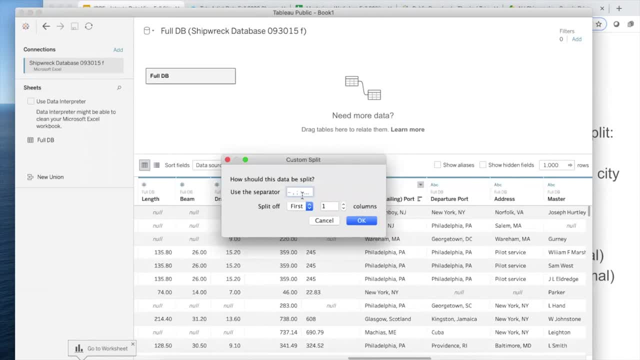 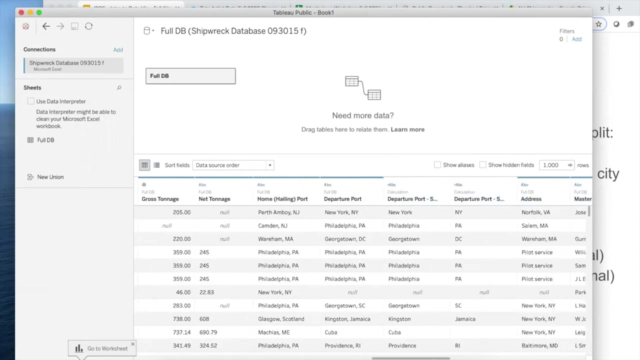 So this gives us the option of any of these separators being a way to separate. So we like that. Let's say, okay, Let's do an automatic split. there we go. So we have departure port. we also need to do that for home hailing port. 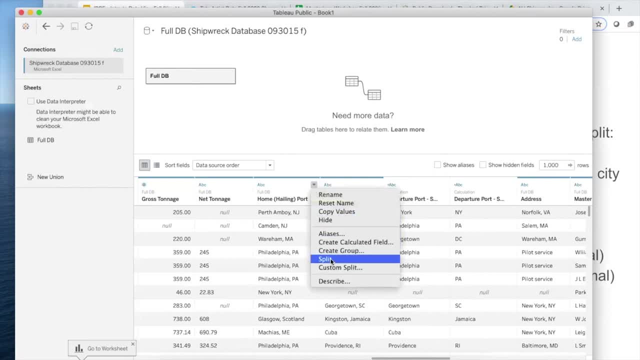 Okay, And so when we do that, We can relabel them right and we want to make sure that they're labeled correctly. So these are cities. I'm just doing this quickly, but in theory we'd we'd go through and we. 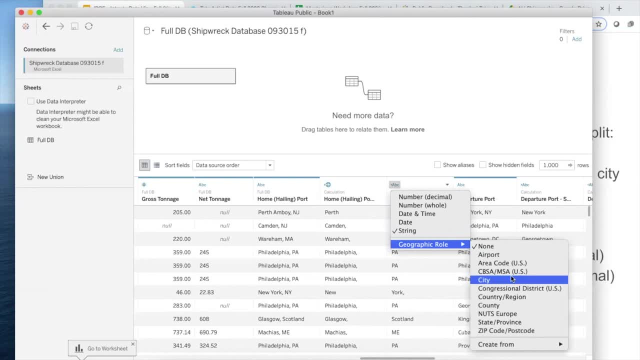 make sure all these commas are dealt with. So we're going to make sure that they're labeled correctly. So, for example, we're going to call this state, And so we want to make sure that this is the same number as the first number that we have. 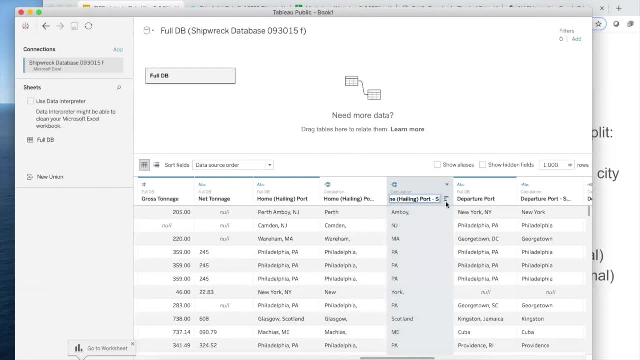 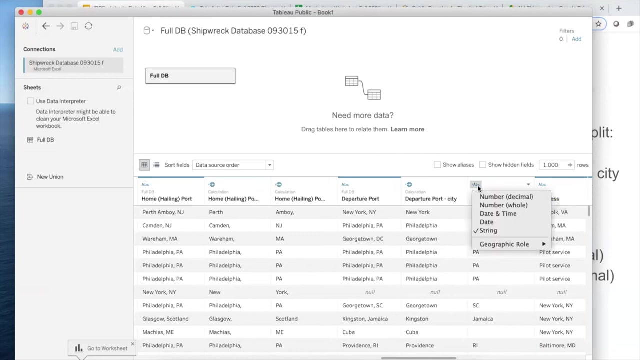 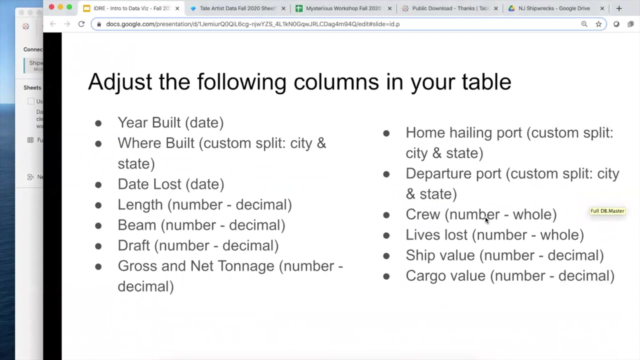 And the same here. we're all getting the hang of this now, right? So I'm going to show you my brain here. So our final things that we want to switch are crew. We want to make a whole number, because you can't have a partial crew member, right? 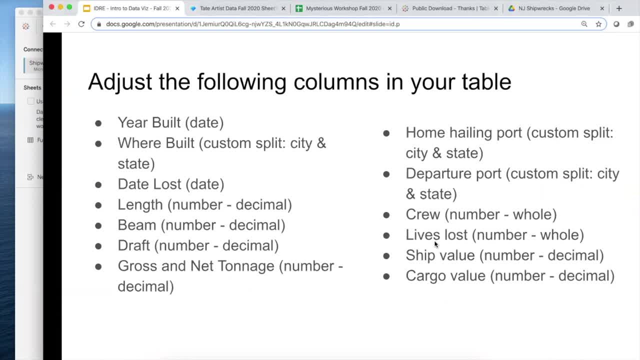 So this is when we talked about data types earlier and different types of data. This is an example of something with an absolute zero, Where you can only have whole numbers. So crew lives lost. You can only lose a whole life. Ship value can be decimal and cargo value can be decimal. 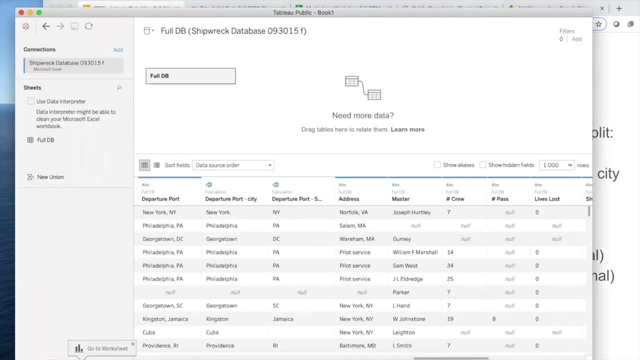 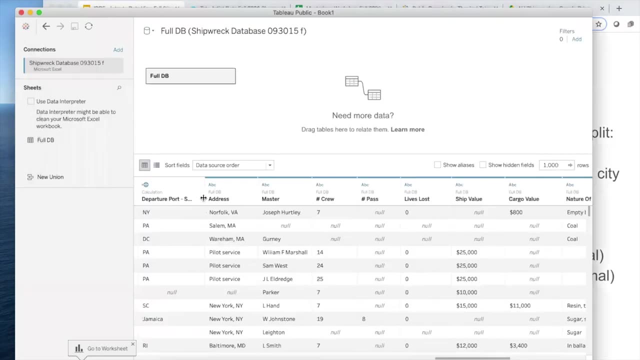 So let's quickly do those. I have a question real quick, Sure. So why do we have to go in and change the data type to number whole or number decimal, when we can probably assume that the numbers input is In terms of like lives lost are already whole like, why do we have to go in and redefine it? 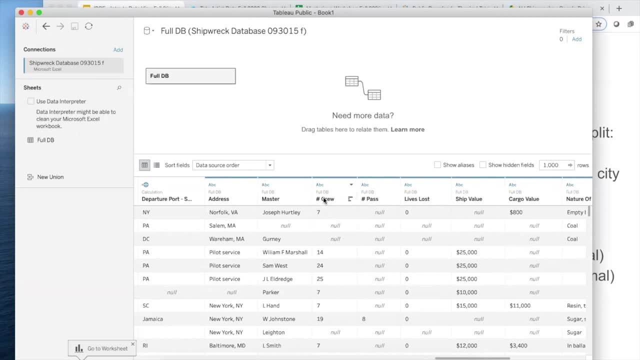 Right. So in this case, if you see here crew number it actually the problem is that Tableau wasn't smart enough to relabel this as whole, So you have to tell it that it's a whole number. You have to tell it it's a number. 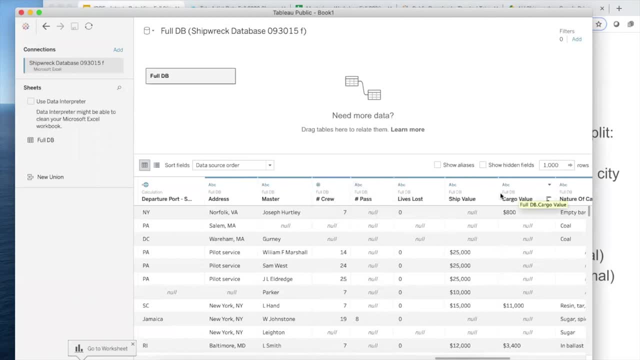 And if you're doing that, you have to tell it what kind of number it is right. So if this comes in and it already identifies it as a number, then it may work out just fine. Um, but it depends on the kinds of. 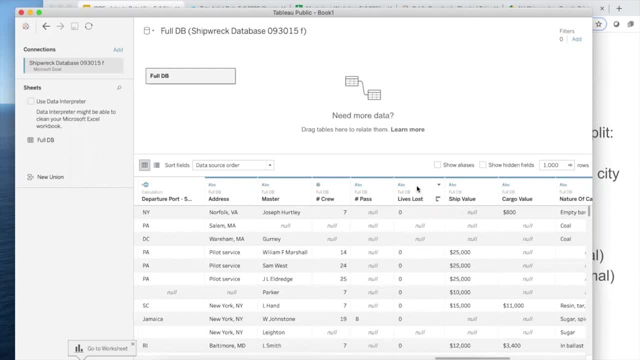 Visualizations that you're attempting to do, And that's when whole versus decimal can matter. Um, so it just depends on sort of what the goal is of your and the data, the graph type you're choosing to make. but ultimately it's because when it first comes in, it's not recognizing. 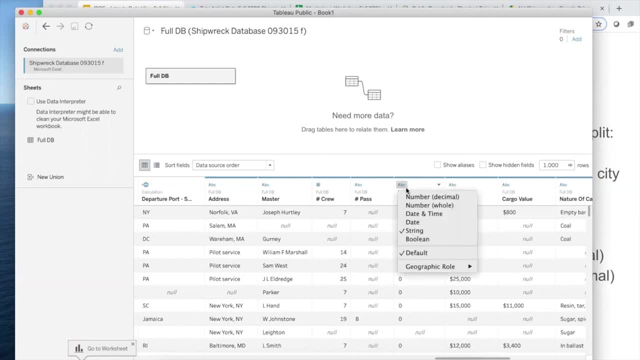 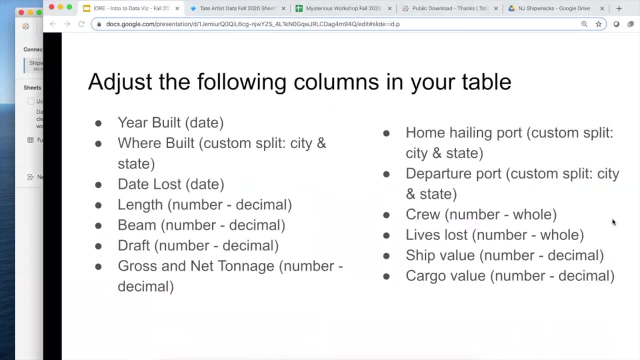 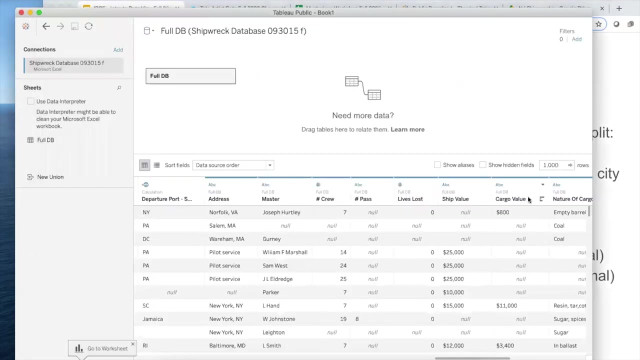 these things as um, it's recognizing them right now as a string, which is text as opposed to a number. Yeah, That's the big thing with great question, and just do quickly ship's value and cargo. Here we go, Okay. 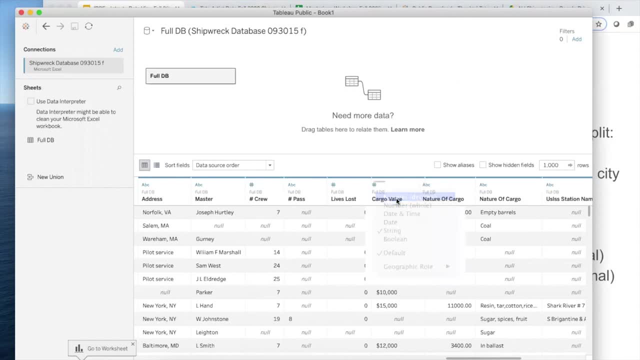 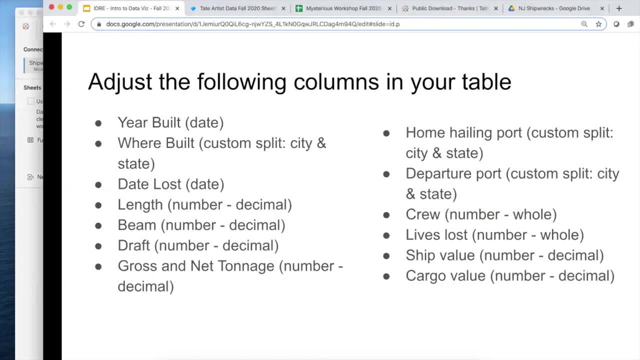 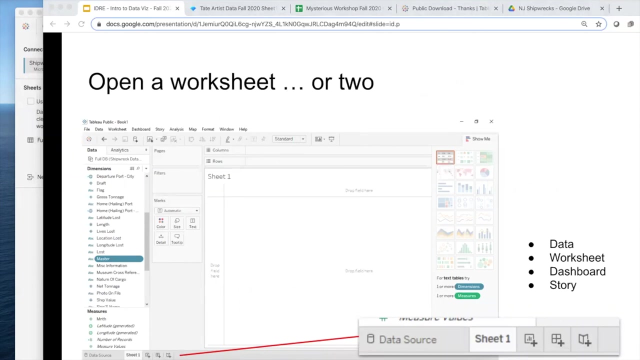 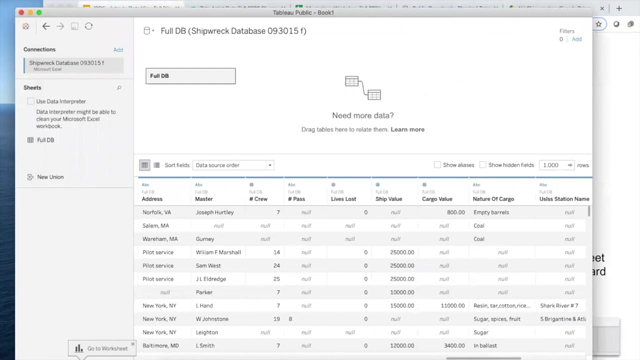 So all of those things should be switched over now. So once you've prepared your data, Now you can start working with your data. so the interface is a: you're going to open a worksheet and once you open a worksheet- so this is- you always have your, your data. 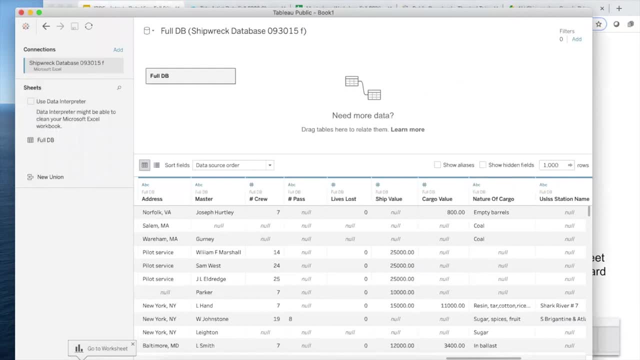 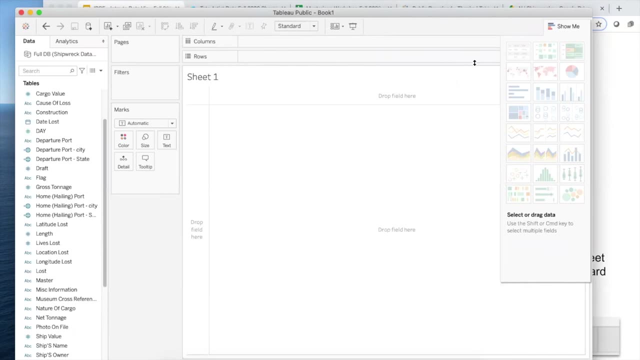 source that you can go back to, which is this, but you're going to click sheet one and that'll allow you to see your data. So now you have your Visualization, So you can see your data. So this is the visualization interface and this is a WYSIWYG interface. 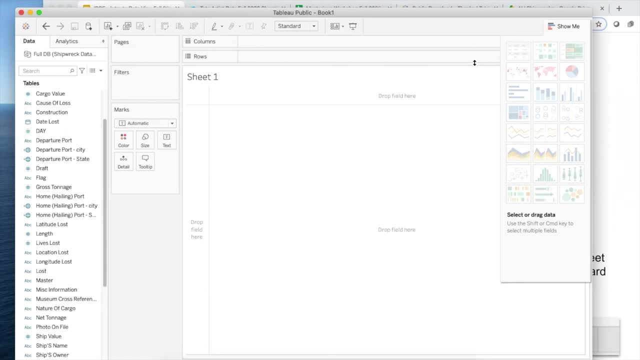 So WYSIWYG stands for what you see is what you get. Essentially, It means it's a drag and drop interface. So the difference between dimensions and measures, as we can um tend to see over here, um, right now it's in two. 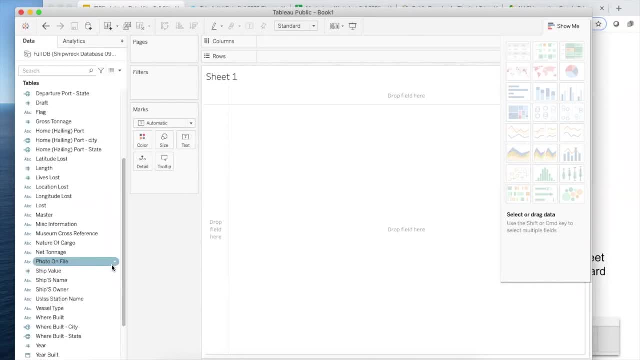 Well, so the difference between dimensions and and measures um, which you'll see in the Okay, which you'll tend to see this data side split into, right now It's in, we'll get into that in a minute, But anyway, dimensions and measures. 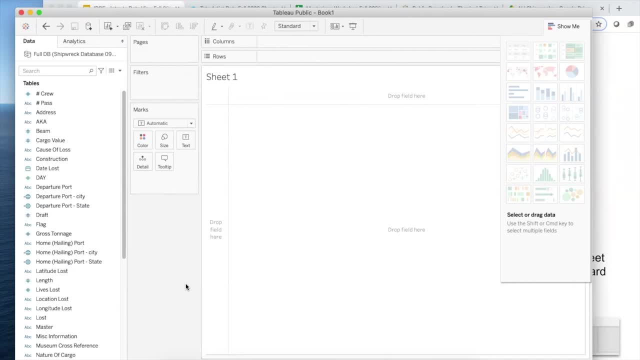 you'll often see in many different types of programs, And dimensions are fields that are used to slice and describe data records, For example, names, dates, IDs, geographic info. Well, measures are the value fields of those records that will be aggregated. 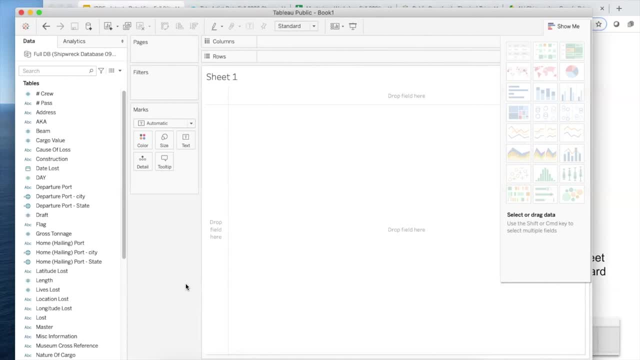 So things like whatever's going to be summed or averaged to arrive at some final results. So the show, and then finally, the show me tool here on the right is a widget that can help guide you on what you need to make for a certain type of visualization. 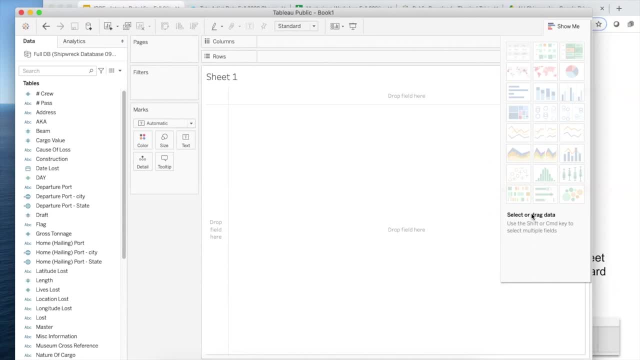 So, for example, if I come in and I say I think I want to make a really compelling bar chart or stack chart, What it tells me is that I need two dimensions and one measures. So I know from my list over here that I have to make sure. 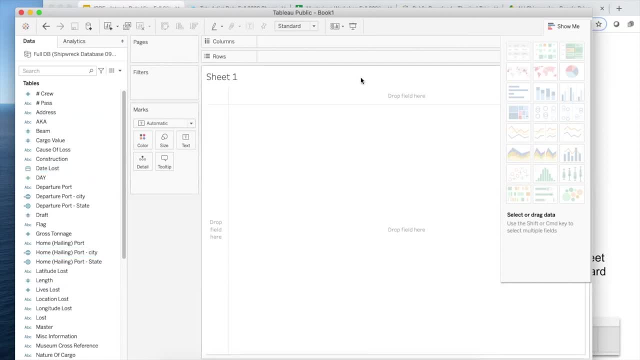 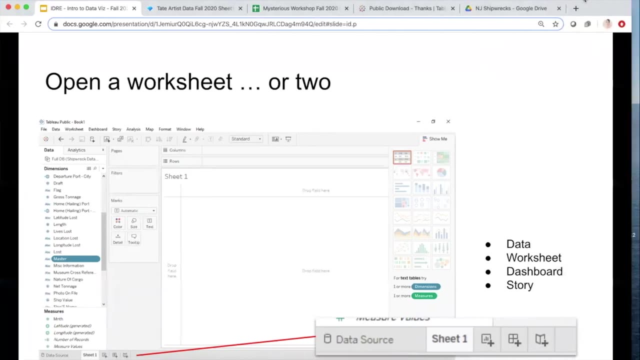 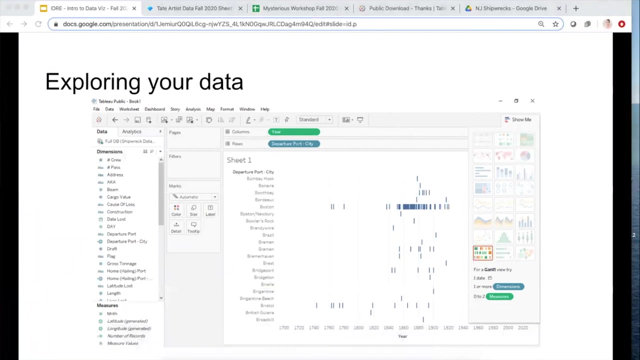 that I'm choosing a dimension versus a measure, So I'm going to hop back to my sheet here to be a little clearer as we move forward. So we're going to start by dragging and dropping the items within the dimensions and measures to the left. 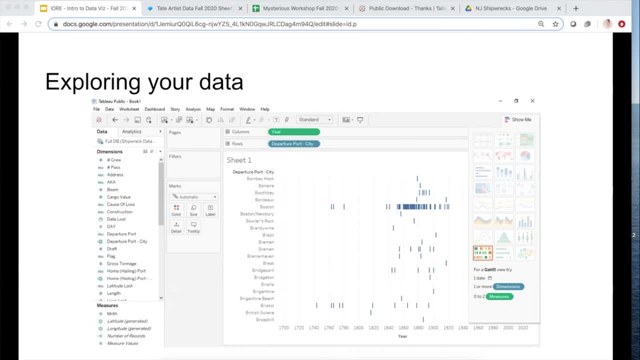 to the column and rows that are at the top to get to know your data a little bit better, And then the show me menu on the right will help guide you about what visualizations might be best suited for the data you've selected. So, for example, if you choose from over here on the left, 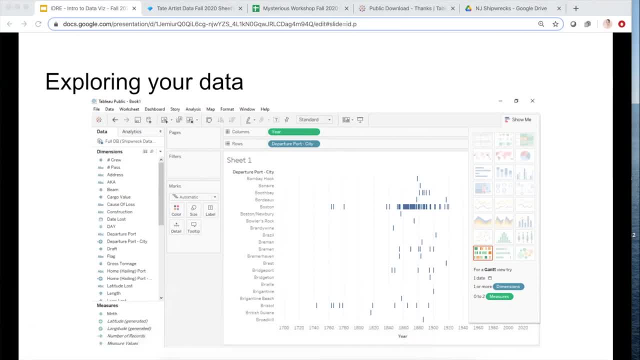 if you bring over year to the column and you bring over departure port, the city, specifically to the row, we can use the Gantt chart to see popular ports and heavy departure years or when, or we could know that the absence or outlier in our data 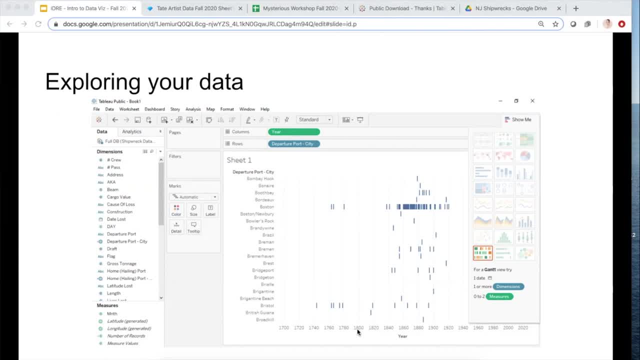 So, for example, around 1800s. when we do this around 1800s, we see there's actually very little data here and might wonder why that might be. So we might do some more research based on that absence. or we might know, wow, around 1860s. 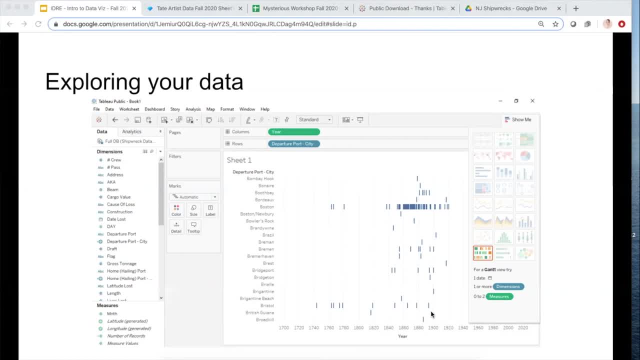 between the 1860s and 1880s there was a lot of traffic, particularly coming out of Boston Right, So we want to look at that and focus on that data for our research question. So this method is the basis for data viz tools out of Stanford. 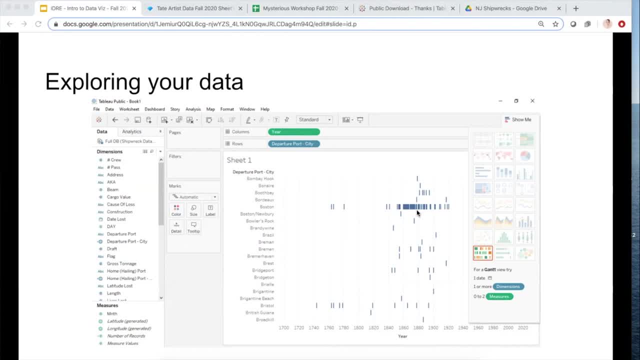 one particularly called Breve B-R-E-V-E, So you can look that up. They also have another tool called Palladio that has a great set of mapping features and can also deal with image data. The only drawback with Palladio is that it doesn't allow. 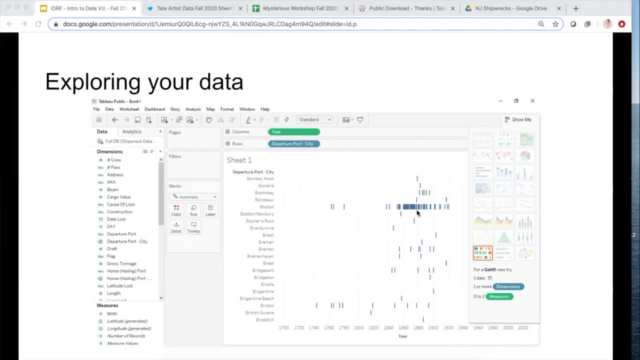 for a dynamic export of your visualizations, which Tableau does, and we'll get to that in a little bit. I know we're running low on time, so I'm going to just stick to my slides now and move forward. But if you have any questions, please stop me. 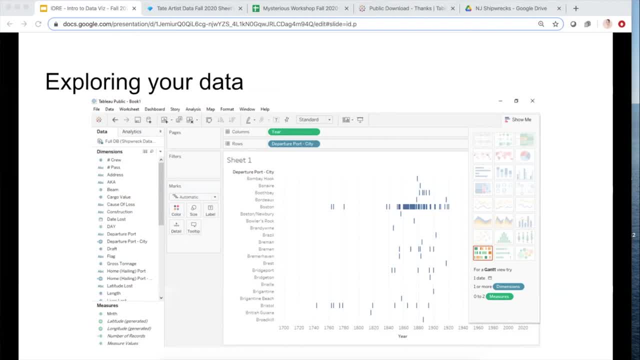 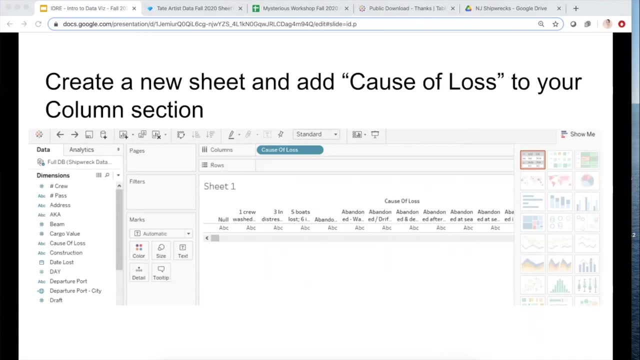 and we can try to jump in together. So if we do another one, we can create a new sheet and add cause of loss to your column section. So again, you're pulling from that left data column and you're going to bring over cause of loss. 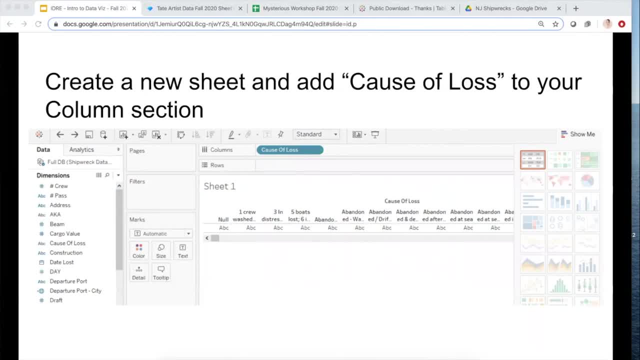 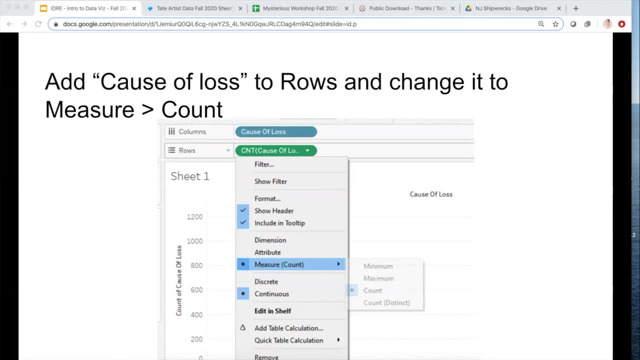 and drag it and drop it in the columns area And then you're going to add it again. So you're dragging the exact same thing, but this time you're going to drag it to rows and you're going to change it from a measure to a count. 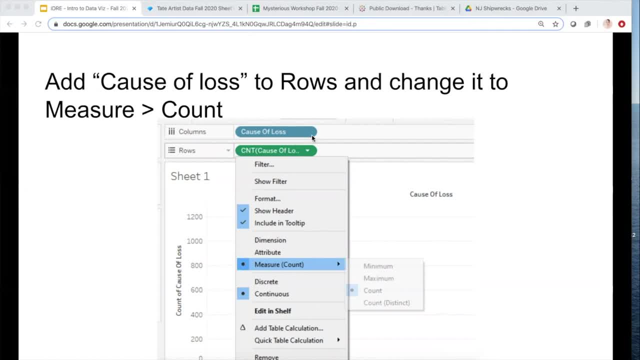 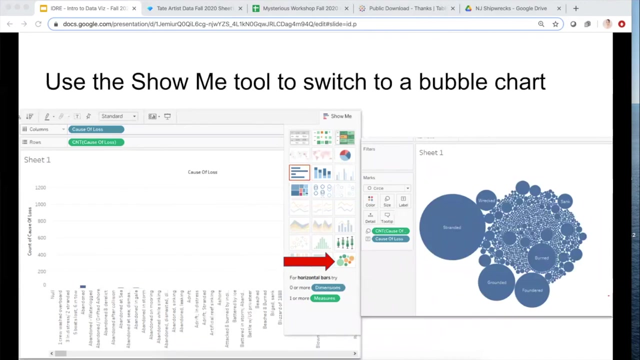 And the way that you do that is, when you hover over these things, you can actually there should be a dropdown that shows up, Okay, And you can click on that arrow and you're going to go down from measure to count. Now, when you do that, likely you'll be. 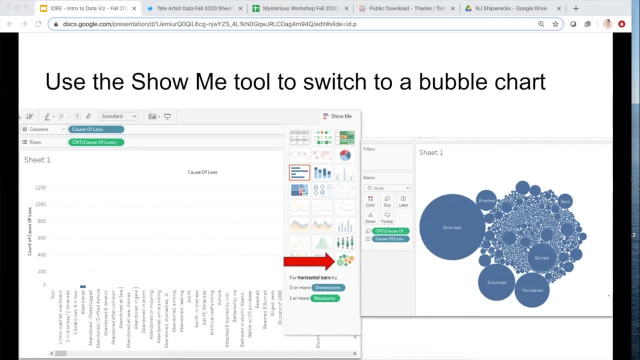 you'll first be given a really long bar chart, which is not really compelling or useful, And this is where the show me tool can be really helpful. It will highlight all of your data. It will highlight other chart types that can fit the way. 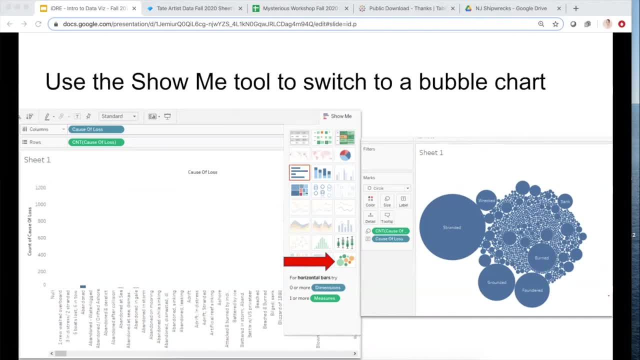 that you format it. that can fit to the way that you formatted your data. So in this case, switching to a bubble chart makes it really easy for us to see what are the top causes of loss within the data set right? So if we go back to our design- kind of fundamentals- 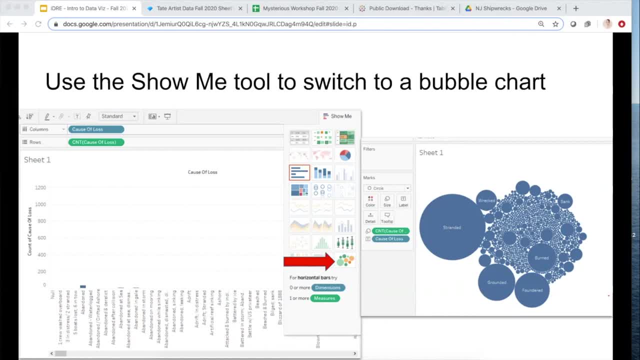 that we talked about at the beginning of the workshop. the reason why you're visualizing becomes increasingly important when you're looking at your data, And this is an example. Okay, Okay, This is an example of where a design choice can make a big difference. 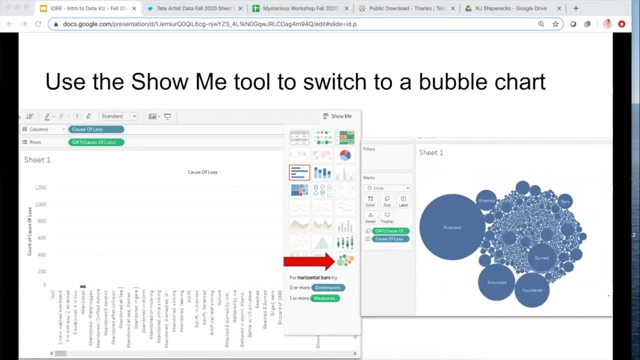 Size here instantly tells us size and shape, right As opposed to a bar chart. if we create a bubble chart, we can instantly see the top reasons for why ships were lost And while the biggest is that they were stranded, we can also see something like wow, a lot of them burned. 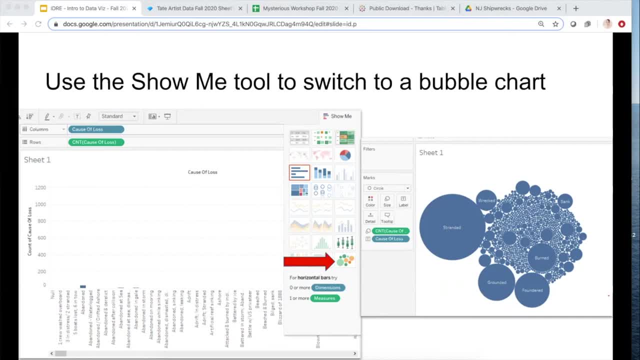 So what was the degree of fire safety? What was the degree of fire safety on these vessels at particular times, And maybe that's worth looking into. So this is a way that we can get to know our data really quickly by using a data visualization. 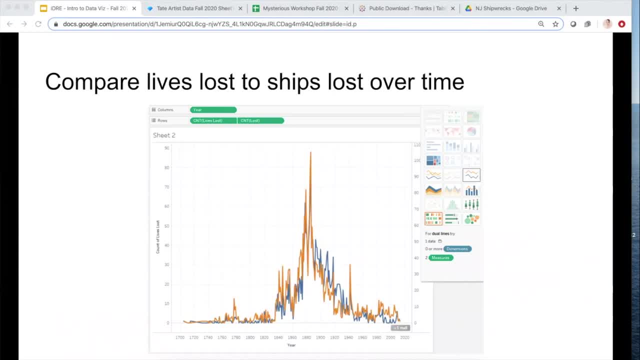 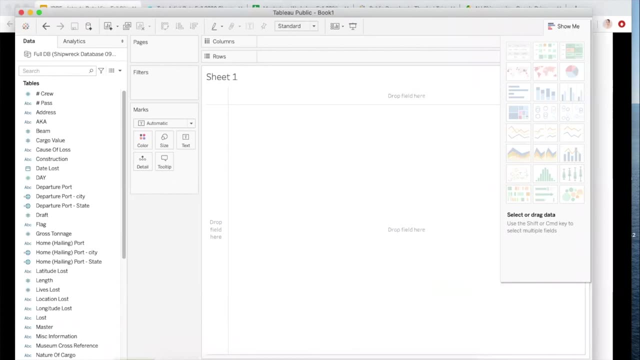 We can also do comparisons. So let's create again a new sheet. So at the bottom of your tableau. let me just show you here. you have these sheets down at the bottom, Okay, Okay, So you can create a new worksheet, a new dashboard. 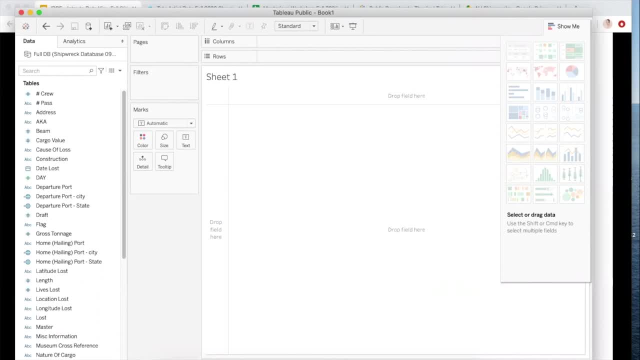 which we'll talk about in a minute, or a new story. I believe this is story. Yeah, new story. So, each one of these things, you want to create a new worksheet, And I'll show you why that is in a minute. 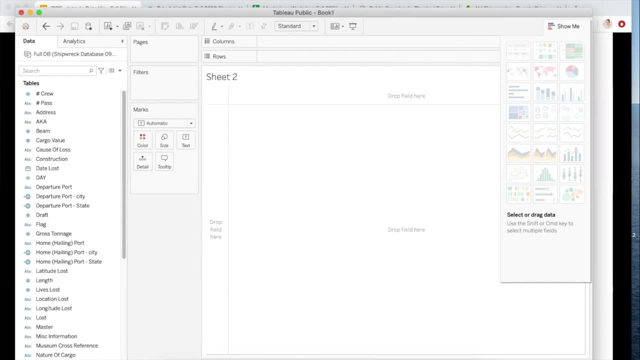 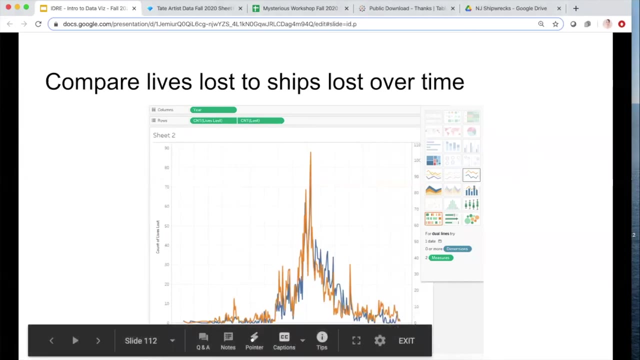 But so when you're dragging and dropping things over, just keep creating new spreadsheets or new sheets down at the bottom, because we can put them all together using the dashboard feature. So I'll show that to you in just a second. So in this chart, we can create a comparison of the lives lost. 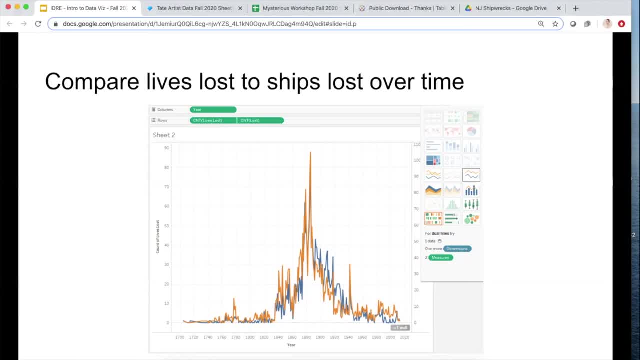 to ships lost over time. So if you drag your year to the column section again, we want that to be the thing that we're building across the horizontal And then you drag both lost and lives lost to the rows, So you're dragging both of those to the same area. 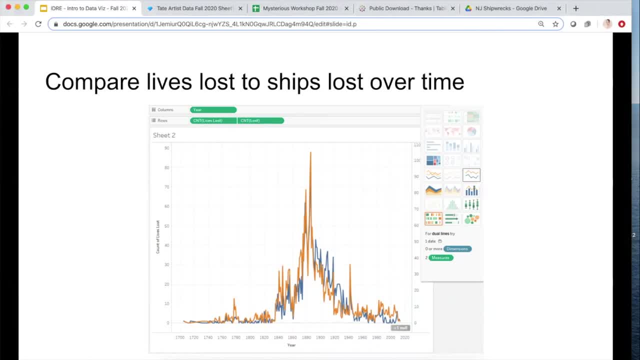 And you're going to switch the measure to select count again, because we're counting how many lives were lost and we're counting how many ships were lost over time, And we can do that side by side comparison or we can do a dual timeline, like you're seeing here, which is a chart that 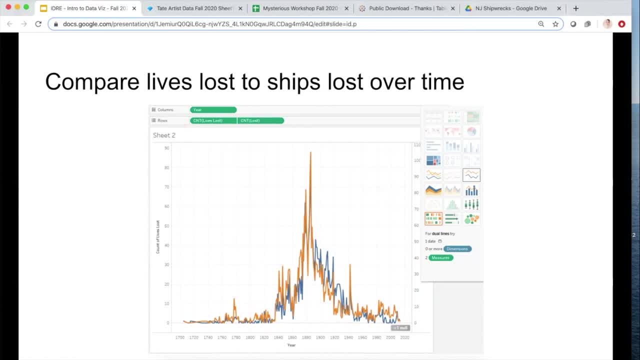 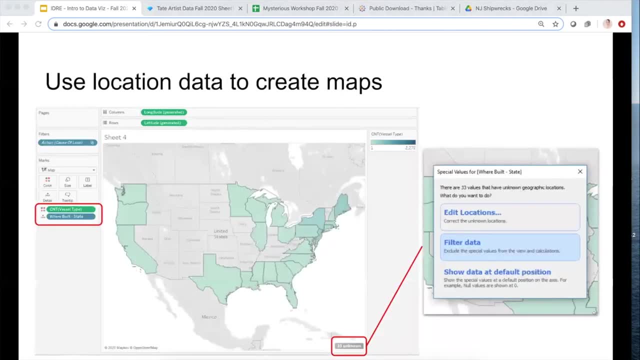 layers the numbers and see them compared directly over time, And then, finally, we'll do one last chart. So this is to show you a little bit of mapping. I recommend, though, that you take a look for workshops with Albert Kachipum or Yo Kawano in our workshop portal. 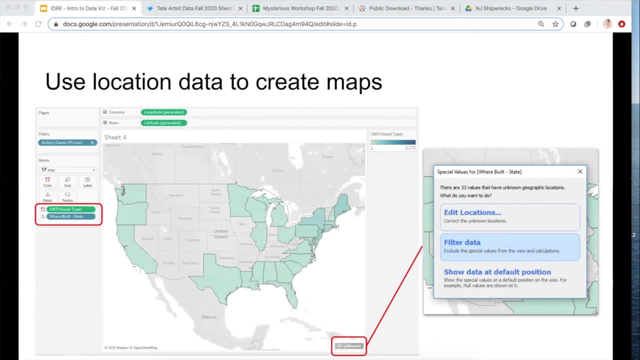 if you're interested in working with location data specifically. But we're just going to dip in, We're going to dip our toe in the water here, bringing vessel types to column and we're built to rows And if we do that, we're going to switch the type to measure. 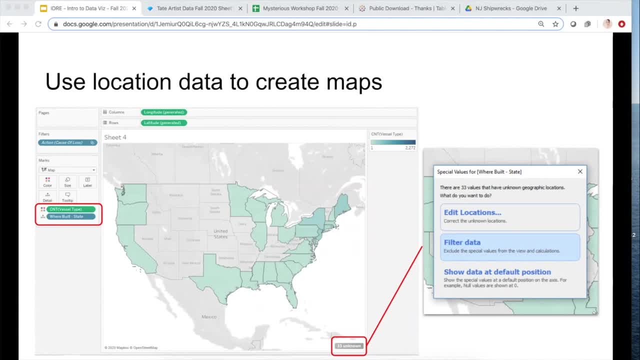 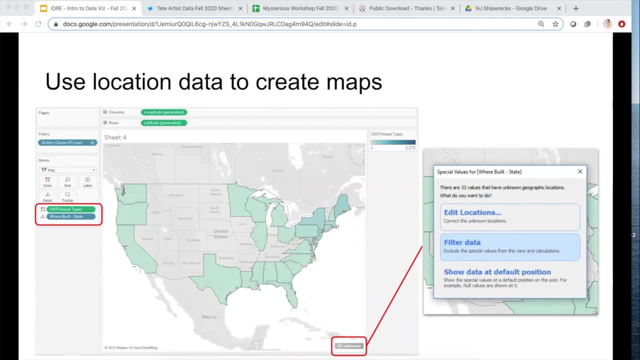 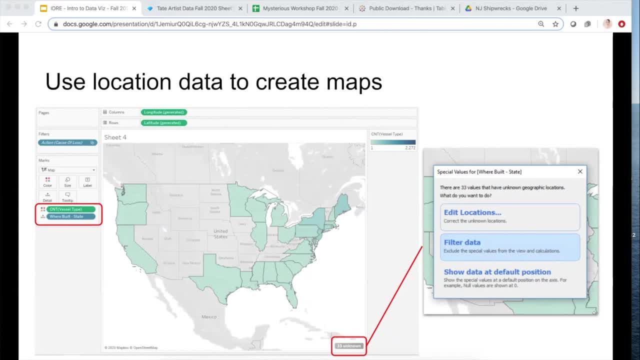 and switch the vessel type to measure and select count and then use the Show Me feature to select maps. Tableau will automatically generate the latitude for you and that's a really big deal Because, again, a lot of GIS tools, that's part of their paid service. 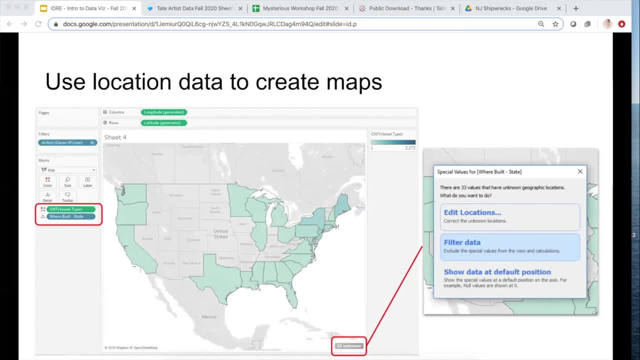 So in Tableau Public you can get it for free And you want to exclude these 33 unknowns for now, because we only want to look at location data that we know, And excluding these unknowns will give our visualization more contrast. 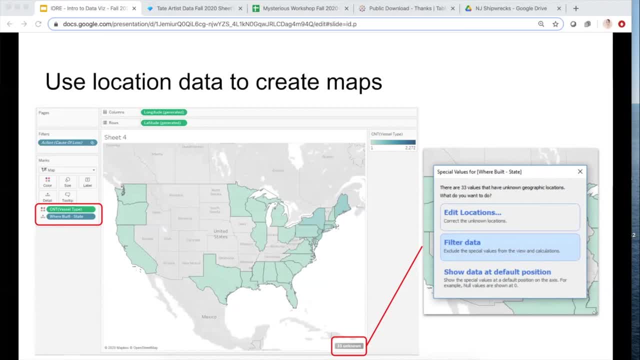 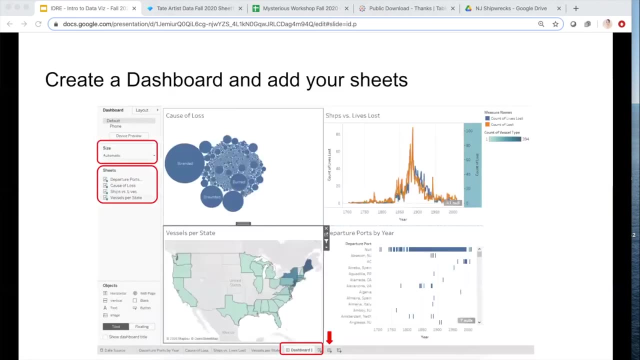 and obviously we'll look into those. 33 unknowns are examples in our data of things that we might want to look into, But for now we want to just get a sense of where these things were built. So when we do that, you'll see, we'll have a higher contrast map. 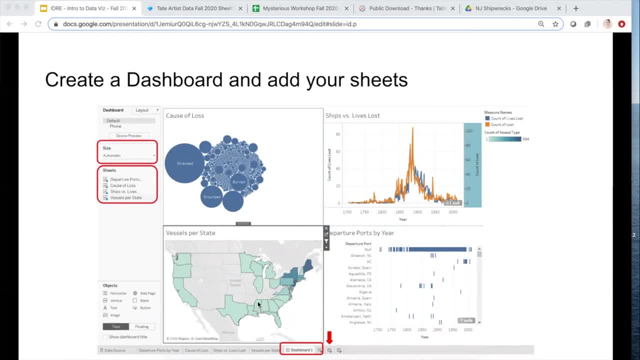 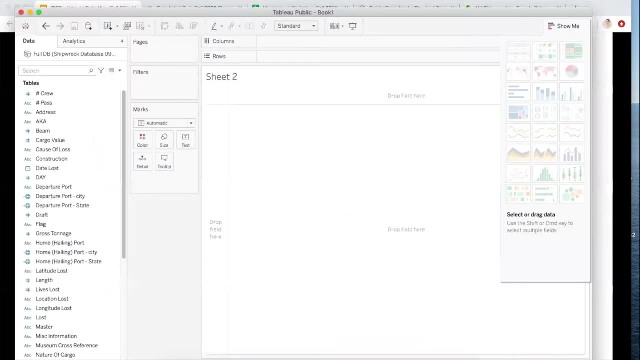 But what we can do is we can then filter our other graphs based on this map if we use the dashboard feature. So the dashboard feature again. I'm going to slide into Tableau for a second here, just to show you where the dashboard feature is. 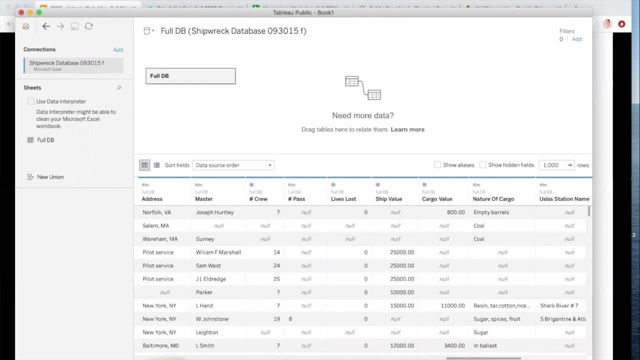 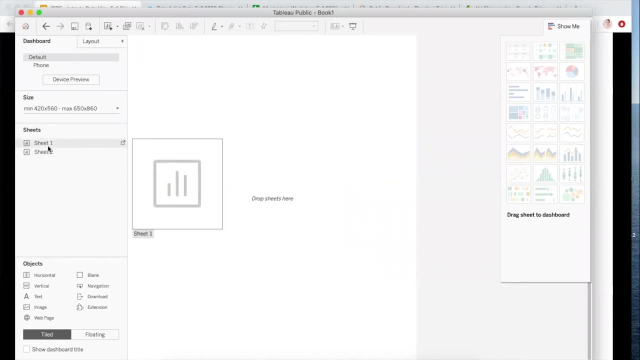 The dashboard feature is this second little thing down here, And once you've created different sheets, you'll see they show up here in your dashboard menu, on the left of things that you can drag over. Right now I don't have anything in these sheets. 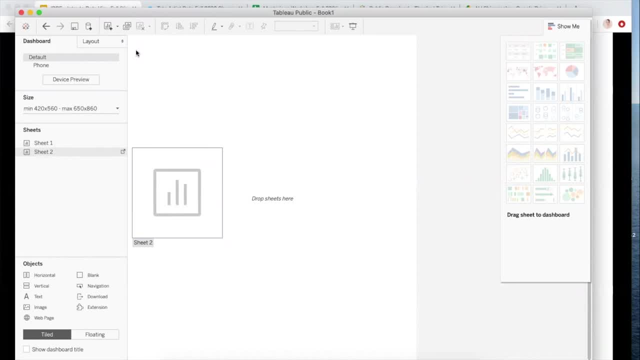 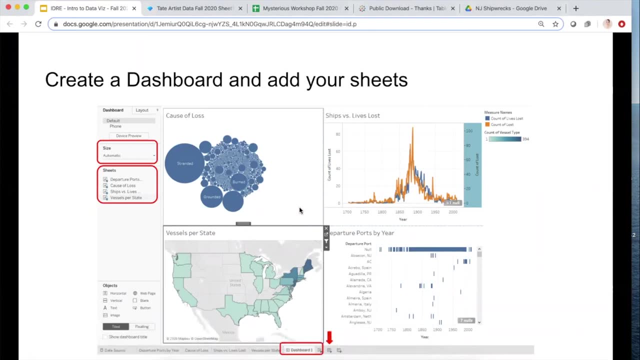 so it's not going to look very dynamic. But if you followed along and created those charts like I did there, you'll be able to drag and drop them over And they kind of snap into view. so you can pull them against each other and they should readjust nicely. 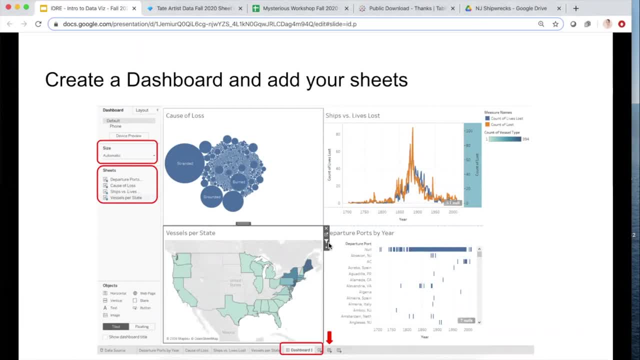 And using this little thing that looks like a funnel, you can connect all of these things to one another. So you use the center icon at the bottom of the bar to add the dashboard, and then you drag over your sheets from the left into the space on the right. 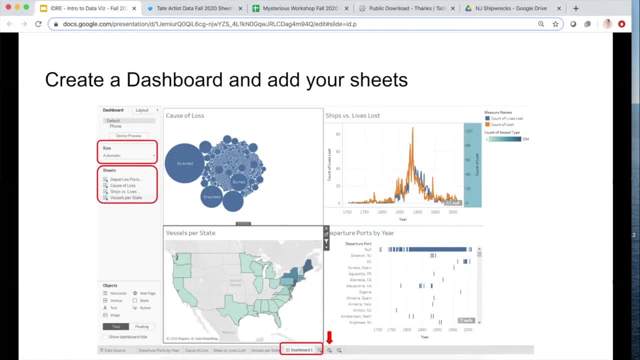 Adjust the center icon and then you drag over your sheets from the left into the space on the right. Adjust the center icon at the bottom of the bar to add the dashboard. You can import the size in the left menu to automatic and the graphs will automatically make room for one another as you drag them over. 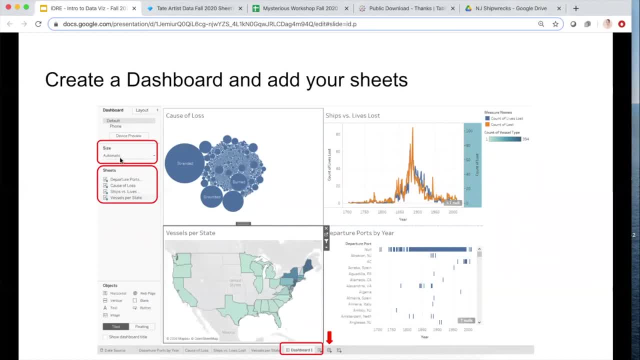 So see this thing over here: If you adjust size and make it automatic, they'll naturally kind of format into space with one another nicely, And labeling your sheets will help keep things clear. So double-click on their tab at the bottom and rename them. 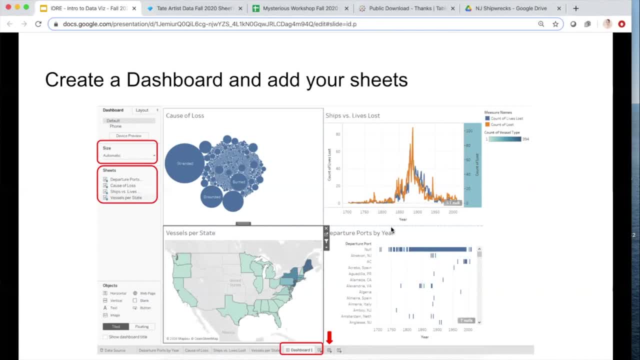 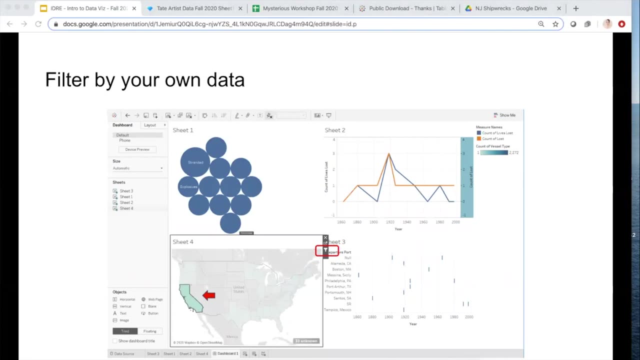 So in each one of these you can double click and you can rename these So they're very, very clear on what each graph is. Like I said, you can turn on the filter for all of your data visualizations within the dashboard. 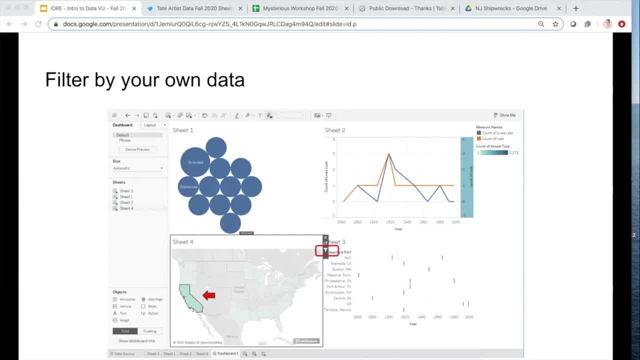 And this allows you to filter all your data visualizations by whatever data you select within one of the visualizations. So if I wanted to look at California, right, the data related to California across all these data sheets- when I do that, when I click on this, all of these charts are filtered by that piece of data. 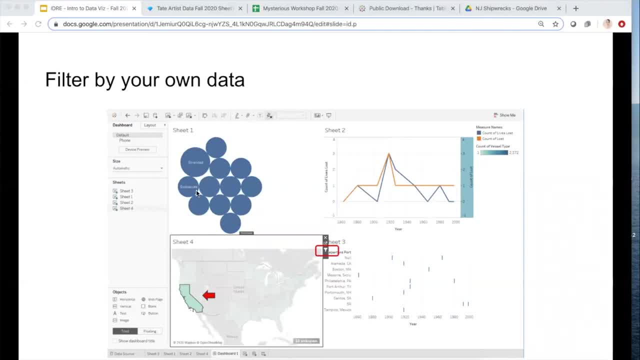 Then I can click it again and unselect it, And I can do that for if I wanted to look at the stranded ships, right, and that will filter both the map, the comparative chart and the Gantt chart by all the data. 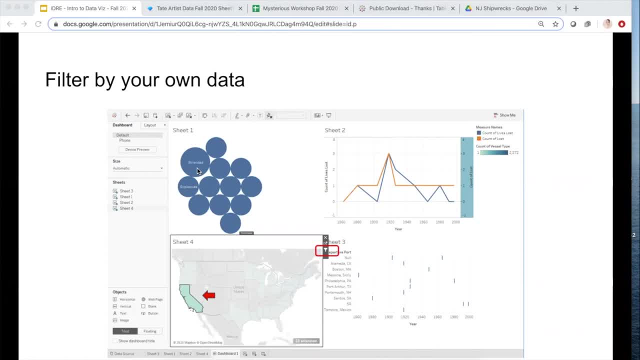 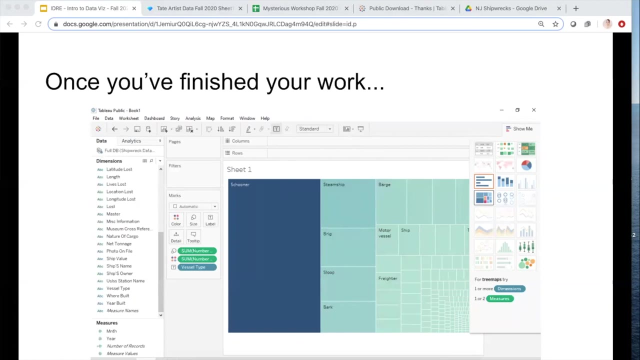 Stranded data types So pretty cool and powerful, especially when you're trying to create a narrative with your data. And for those of you who are wondering, I'm seeing in the chat. I know we're coming up on the end of our time together and I will be wrapping this up very quickly. 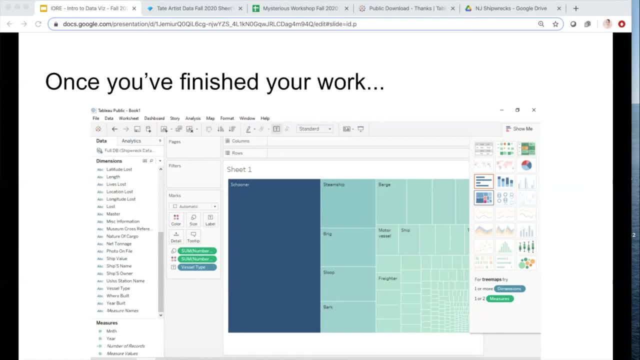 But the recording will be on the IDRE I-D-R-E YouTube channel, So take a look Out for that. I'll also send a follow-up email. if you've signed in using that spreadsheet in the very beginning, I should have your email from that. 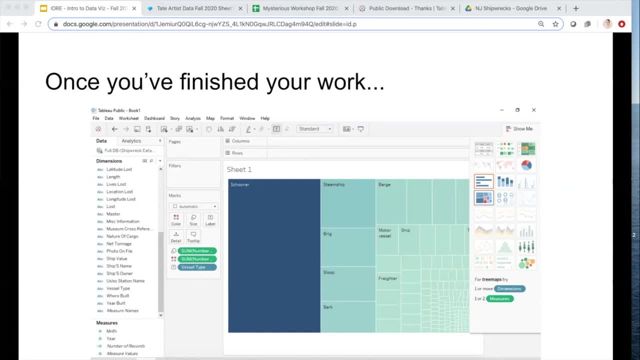 If not, you can always email me and let me know, and I'm happy to send you the recording. So great question. Thank you for that. And once you've finished your work, you can export and embed dynamic visualizations into your webpages and such. 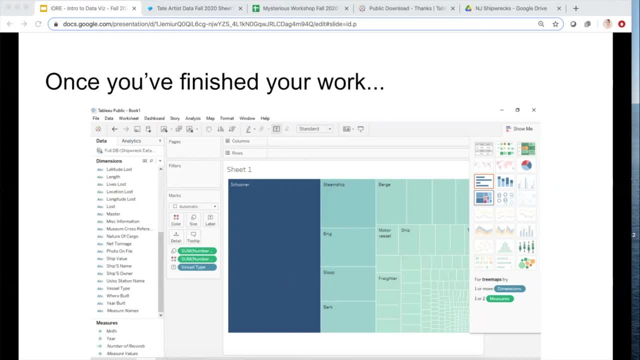 So another great aspect to Tableau is that It exports really easily and embeds really easily and you can get dynamic visualization embeds, which are so great for websites right? Everybody likes a visualization that they can actually interact with themselves, and that's what Tableau Public allows you to do. 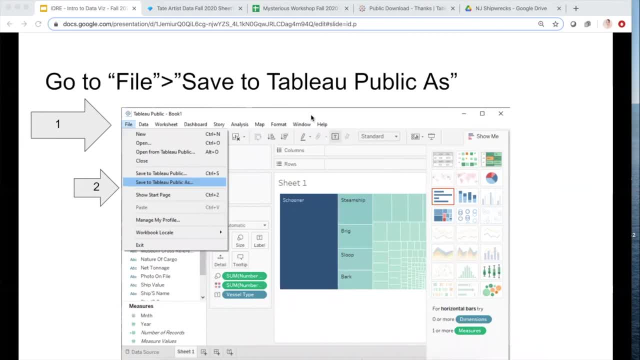 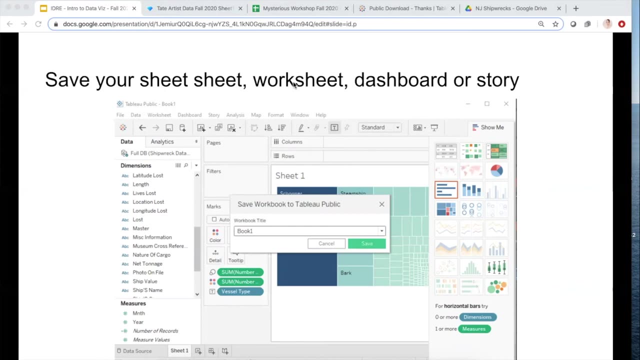 So the way that you do that is you go to File and Save to Tableau Public As. So File Tableau Public As, File Tableau Public As, And you can save your sheets- sorry sheet sheets, sheets, your worksheet, your dashboard or your story- and you'll label them and you'll hit Save. 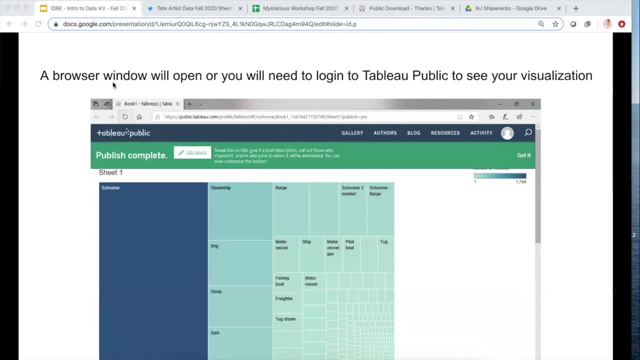 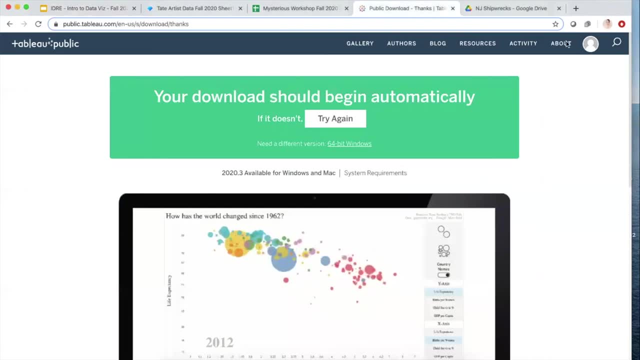 And then what you'll do is, in a browser window, you will need to log into the Tableau Public site to see your visualization. So, again, you'll have to go to this Tableau Public Page and log in. I'm logged in here, but once you do, you can go to your activity. and oh, it's making me log in again. 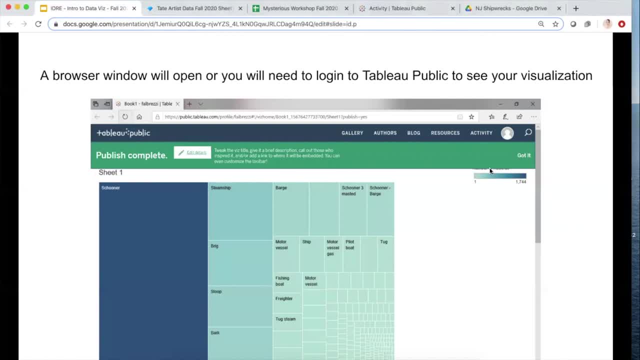 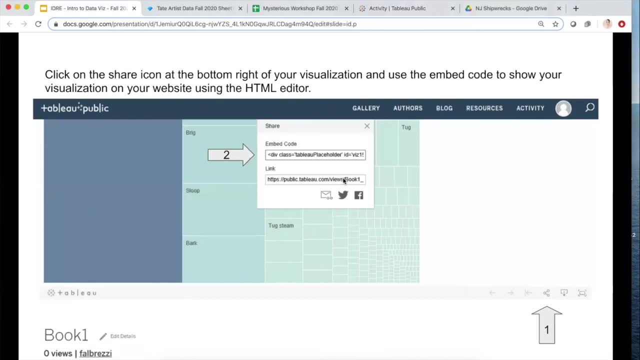 Anyway, you can log in to your Tableau Public page and see it here as an example. Oh, sorry for that. You'll scroll down. It has all your data sheets there for you that you've saved out. And if you go down to the bottom of those windows and click that, 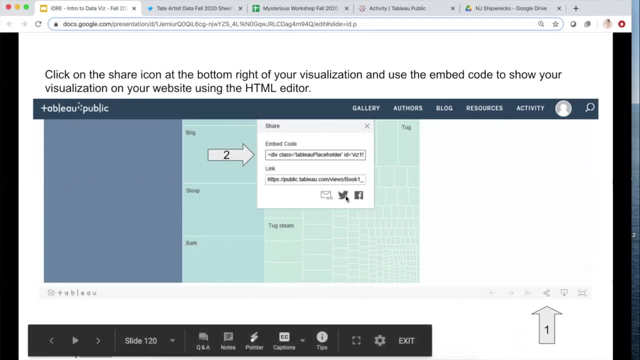 This little connected icon, you'll get an embed code or a link, and you can use either one of those to share your data. I will point out, though, that once you have saved your data out in Tableau Public, it is public. 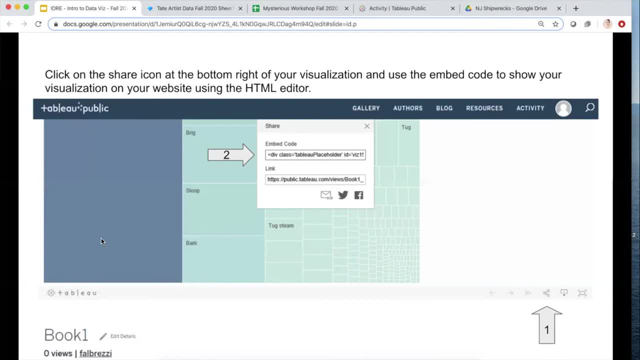 You've made your data public. So please only do this if you are okay with making your data public. If you're not, you can use it on your desktop- Totally fine. You can save it, Totally fine. But when you save it,